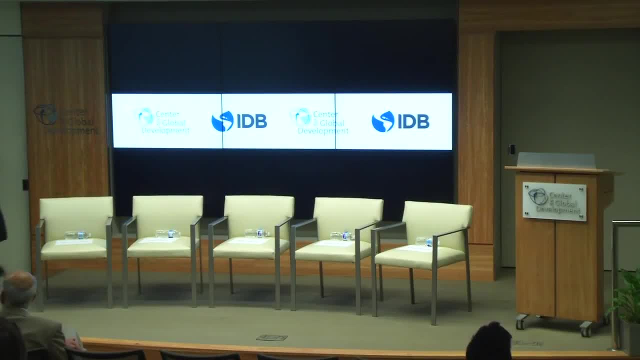 Thanks. So good morning everybody, And let me begin by thanking the Center for Global Development for giving me a book, And Amanda, thank you for hosting us. Thank you for giving us the opportunity to present this book from the Inter-American Development Bank. 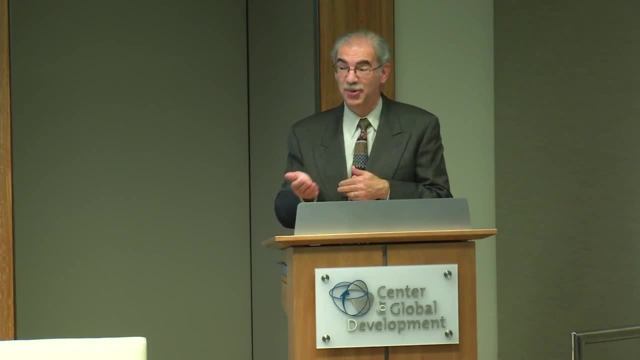 And I'm pleased to see some colleagues from the IMF and some colleagues from the World Bank or ex-World Bank, but from all the other organizations that have been dealing with this issue. So this is a book that was born from a systemic complaint of the bank, of the IDB. 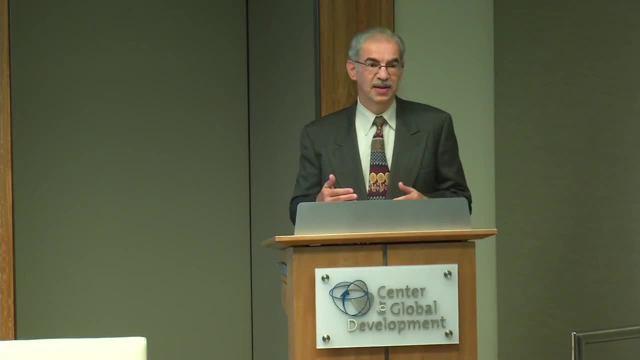 We were always trying to do work, but there's no data. And we would like to know this about Paraguay, but the data's not there. We wanted to do this project in Bolivia and the data's not there. This was a continuous question and a continuous complaint. 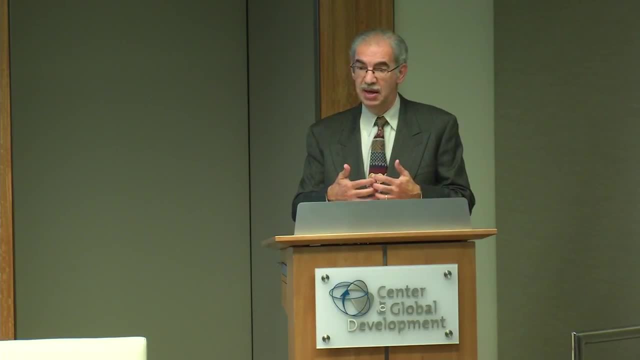 And we realized that the quality of the analysis that we were making was way below what we could potentially be making, because the data for this analysis was not there: Sure for Mexico most of the time, for Brazil, for Colombia, but even for countries like 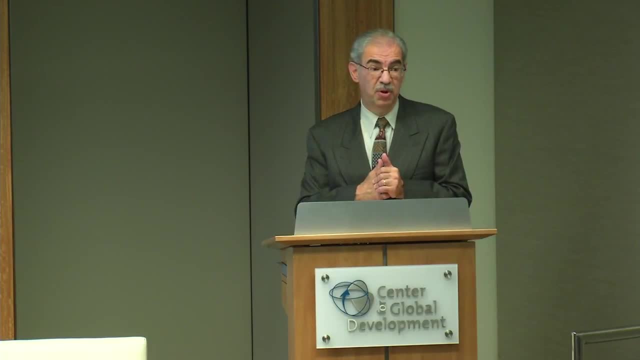 Chile and Peru, which are among the top five countries in terms of income per capita in the region. Many of the times we didn't find the data to do sort of basic analysis. Yes, most macro data, financial macro data, current account data, savings investments. 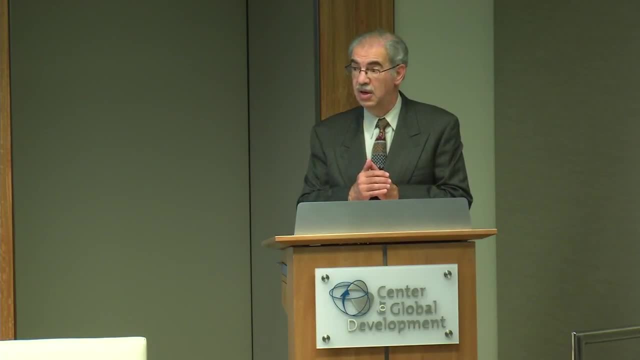 is broad aggregate and the thanks- a lot to the work done by the IMF many years ago- is there. But if you wanted to look at more micro-level data about participation of women in the labor market, statistics on violence, household surveys that went beyond basic food consumption, 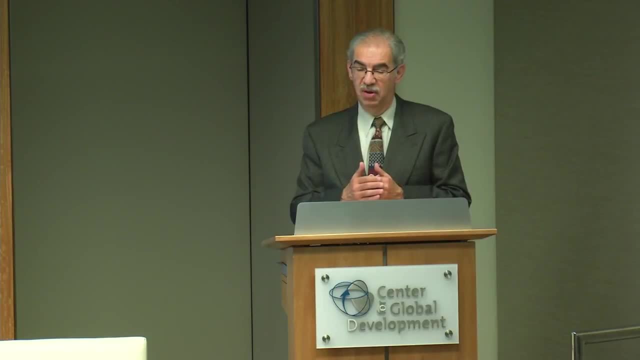 data on transit. Those were not on almost any micro-set current-level data. For most countries in the region that data was actually in the book. So after many years of complaining with José Antonio Mejia and the department of institutions at the bank, we decided to try to understand why this was so. 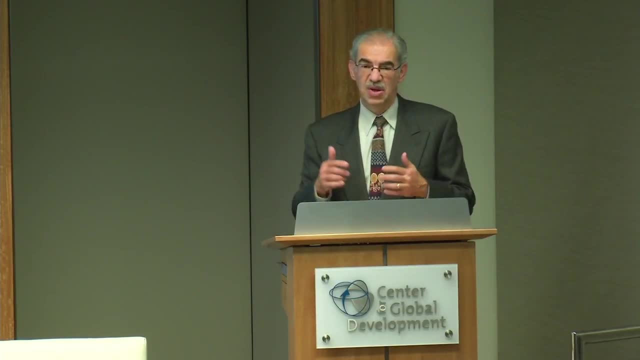 And the premise of the book that José Antonio is 20%- is that the reason this situation is there is not because of money. It is not because countries in Latin America don't have the money. It is not because of money, the resources to fund a statistical institute. 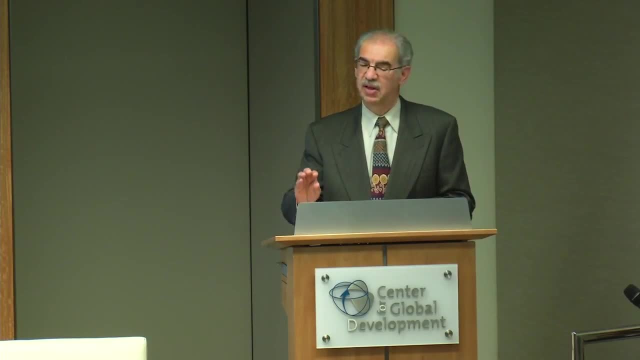 and to be able to actually collect data, Even countries like Honduras and even countries like Paraguay, which have low income per capita. the budgetary effort that is required to gather data is not significant, particularly relative to the rate of return on budget. 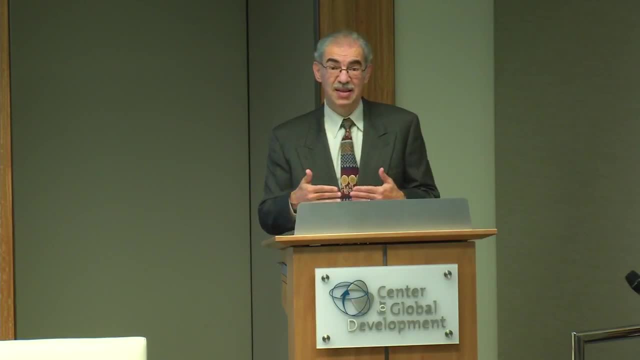 So the premise is that this is not because of money, and it's even less because technological change has actually reduced substantially collecting data. Oh sorry, Do I need to use this, or can I put it here? You need it here, OK. 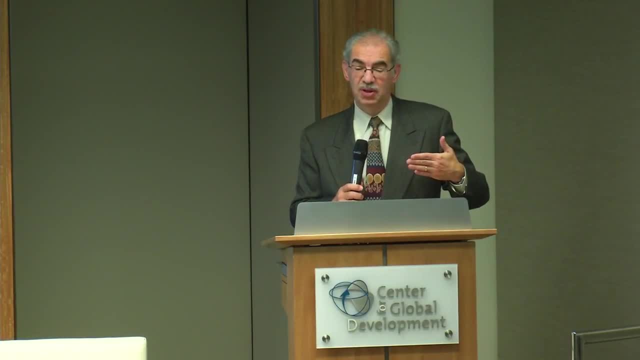 So the point about money is really important, because this is not a money issue And technical change has actually made collecting data ever cheaper. Now in some countries you can actually the people who collect data go around with their iPads that are connected to the internet. 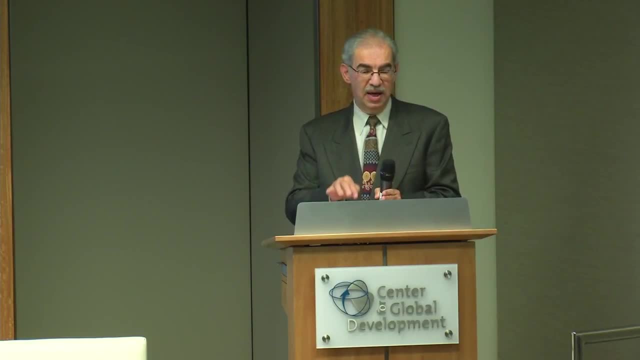 And as the data is being collected, they're collecting the data right on the iPad And the data is being sent in real time to the statistical office, which is processing the data in real time. So there's not even paper involved And you'd need a lot fewer enumerators. 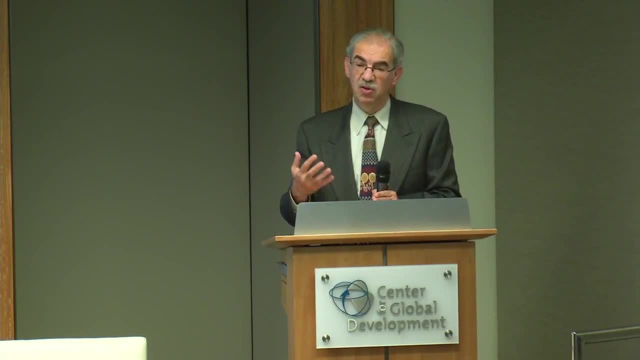 than you needed in the past. So the premise, this problem that we all suffer is not because of money. and why is it then? So The book is an attempt- and Jose Antonio is going to expand a little bit more- is an attempt to understand why is it. 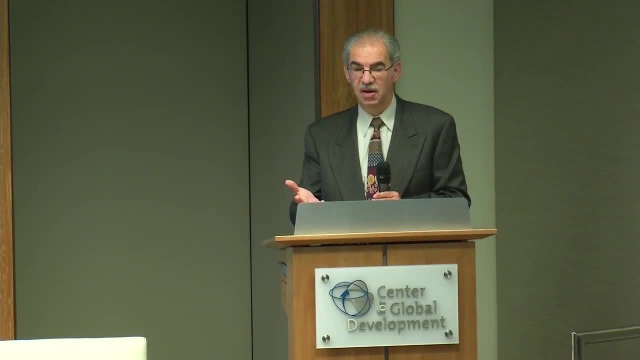 that the demand for data is not converted into actual action by government in producing data, when money is not the reason why it's not, And so we're in the presence of a public good, but it's a public good. that's kind of weird. 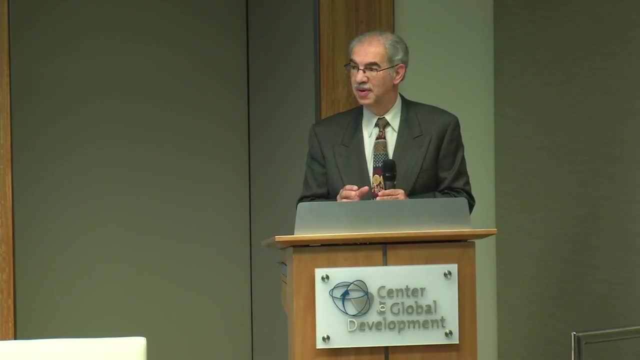 because it also implies some limits on governments, Because when the data is published, the public good is produced, but at the same time something is said about government performance, about how many doctors are in the health clinics and about how many policemen are actually relative. 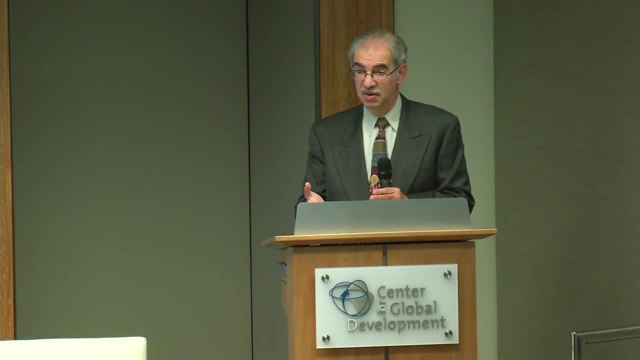 to the numbers of crimes, And so it enhances accountability, and you can see why now the political economy of this becomes a little complex. So let me stop there so that we can actually present what the book has to say. The book is 10 case studies about 10 different countries. 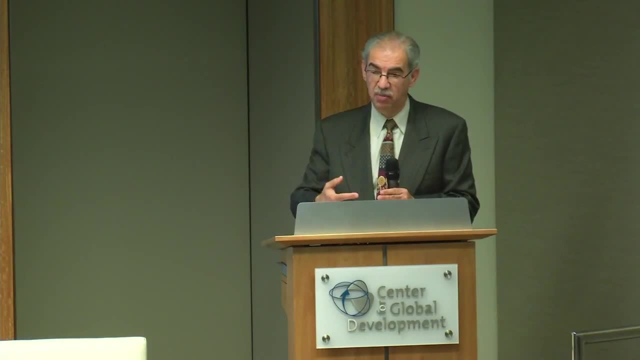 in Latin America. It was put together by some authors within the bank, some authors outside of the bank. It's a research project from the bank And the idea is to help us all understand this problem and hopefully eventually to make something to do and improve it. 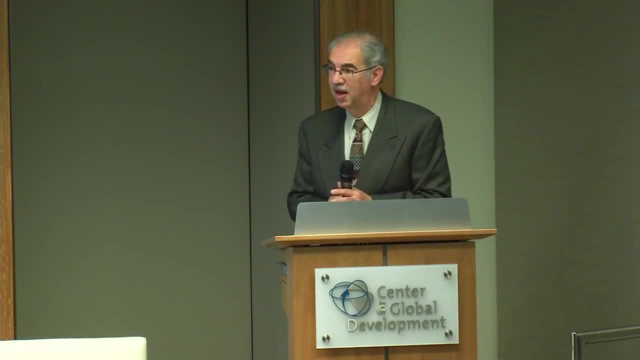 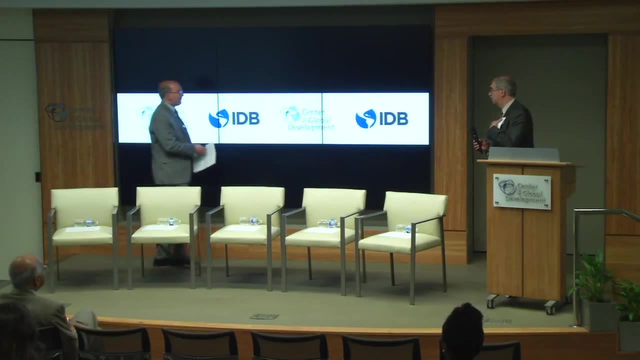 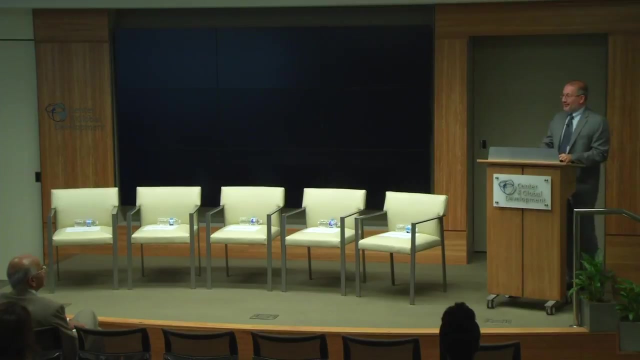 So, thank you, Amanda, And I don't know where Jose Antonio is. I think he's breaking the presentation. Let's see. do I need to use this? No, All right, So I'll give it back. Well, good morning to everyone. 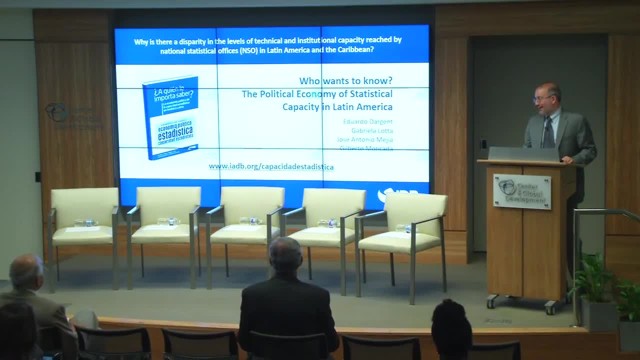 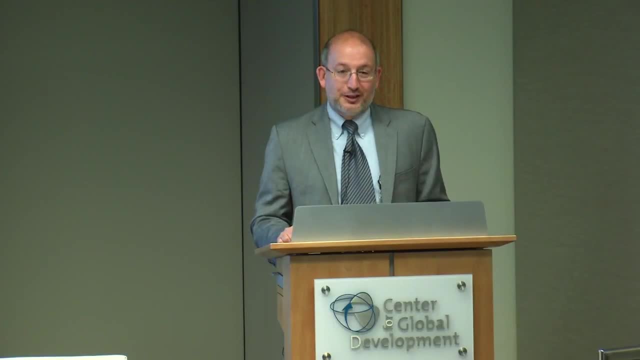 Thank you very much to the Center for Global Development, Amanda in particular, for welcoming us this morning and for hosting this event. Thank you, Santiago, for the introduction and the support through the years for this project. Thanks to Cheida, Roberto and Matthew. 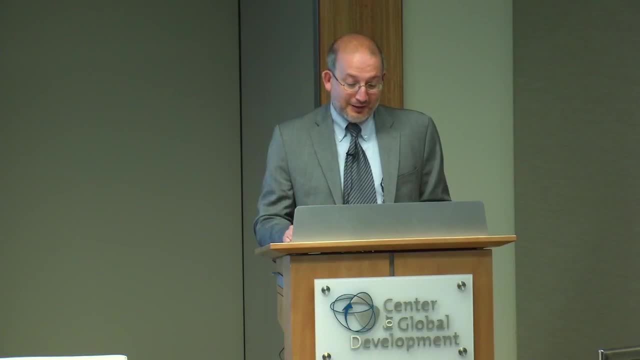 for agreeing to comment on this book. Thank you for all of you that are present here and for those connected through the live stream and through the 10 countries that participate in the research, And I would like to thank the Er oben research in the research project. 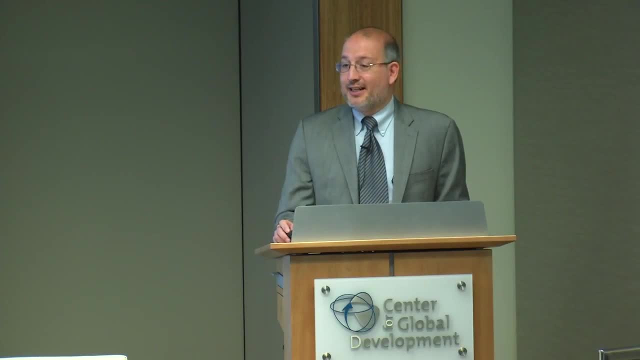 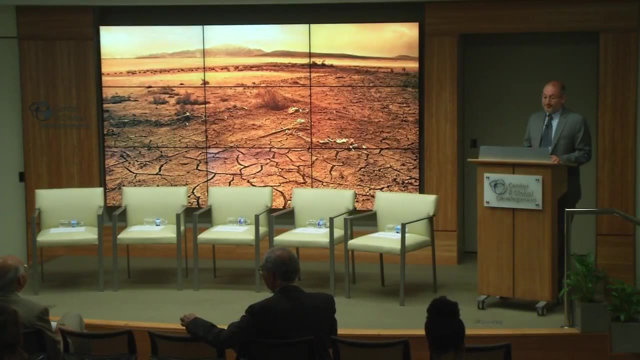 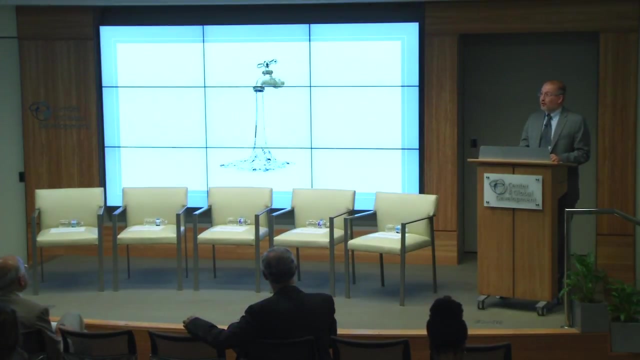 And particularly thanks to Eduardo tsun, Gabriella Lota, the co-authors of this book, And you know, just in line with what Santiago was saying, You know, I think that data is like water, And just like we take water for granted. 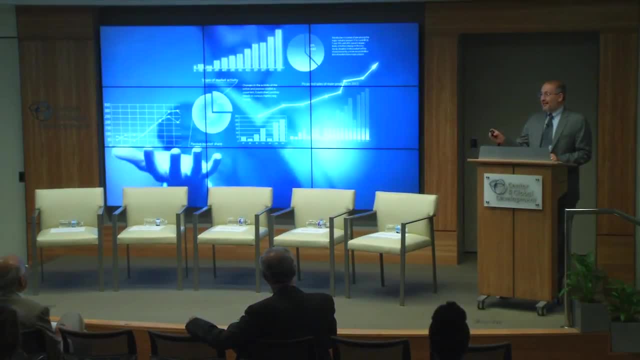 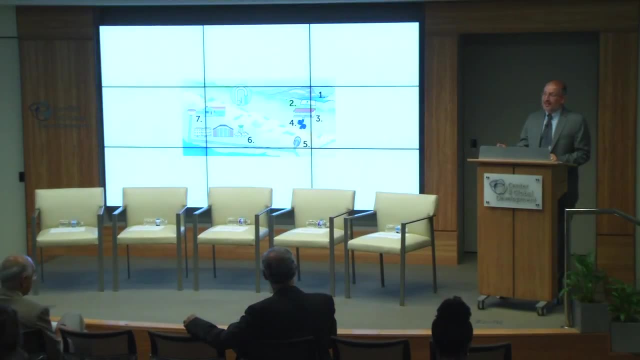 and expect it to come out of the faucet every time we open it. we take data for granted. We expect to open a website and just find the data right there. We seem to forget that behind those numbers, behind those flows, there's a complex process. 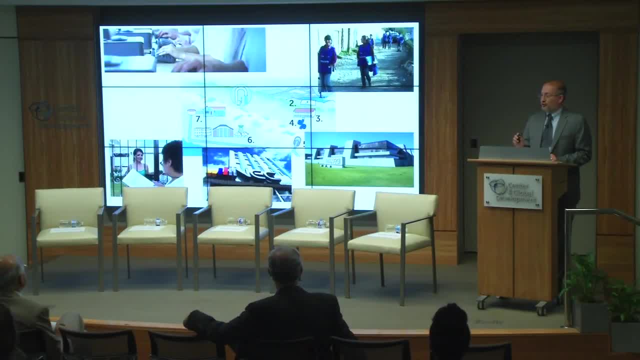 and there are complex institutions, And these institutions- the national statistical offices- is where the IDB is focusing with this study. We decided to embark on the research to understand not the technical part of this institution, but more the organizational part and the way they work in their relationship with society. 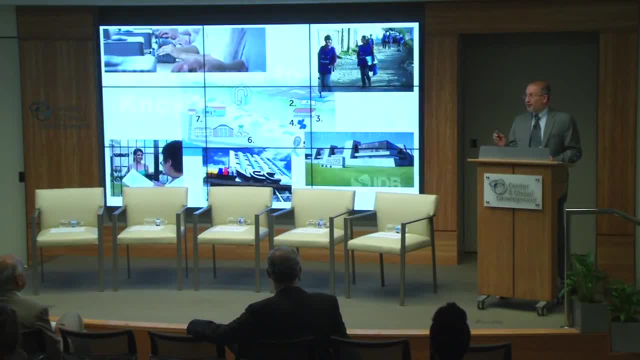 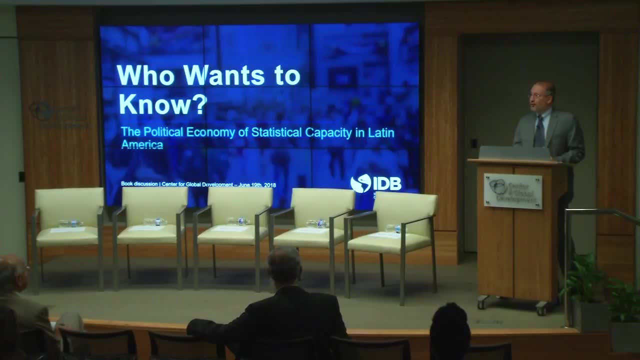 and with the rest of government. So today I will present to you this book that Santiago says is the product of many years of research, and it's called Who Wants to Know The Political Economy of Statistical Capacity in Latin America? I will divide my presentation. 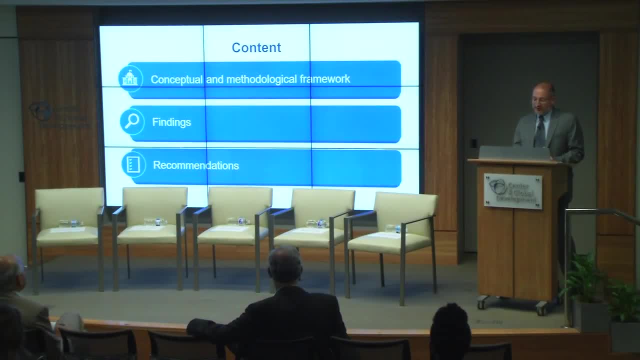 into three parts: First, the conceptual methodological framework that serve as a guide for the case studies. Then the findings from these 10 case studies that we did in the same number of countries. And finally, some recommendations and conclusions for the way ahead. 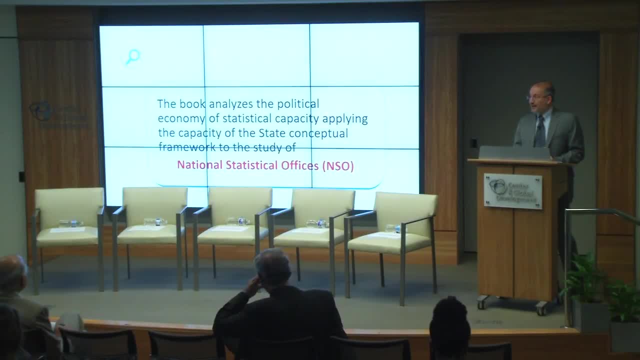 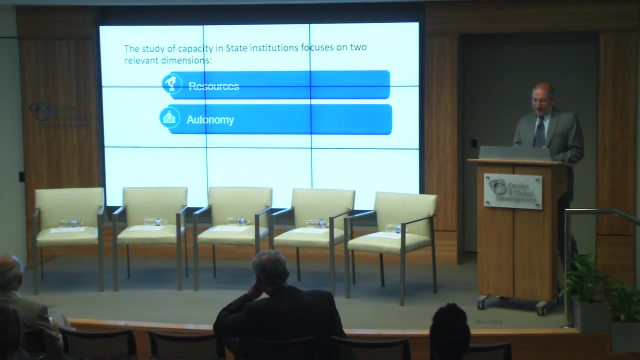 And, as I said, the book analyzes the political economy of statistical capacity from the perspective of the study of the capacity of the state. We're applying this perspective to the study of specific cases, Specifically the national statistical offices, the NSOs. The conceptual framework of the book: 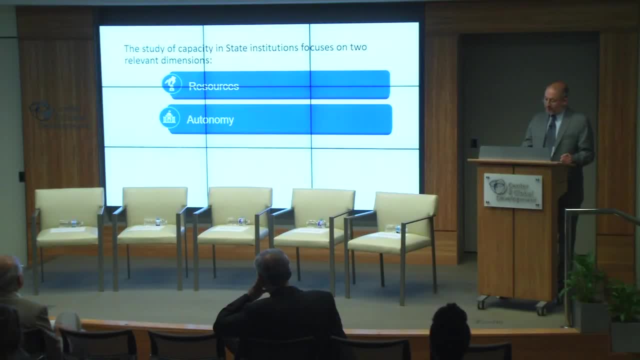 starts by indicating that, while the study of the capacity of the state focuses on two dimensions- resources and autonomy- in order to study national statistical offices, it's necessary to focus in another dimension- coordination, And that's because the NSOs have the responsibility. 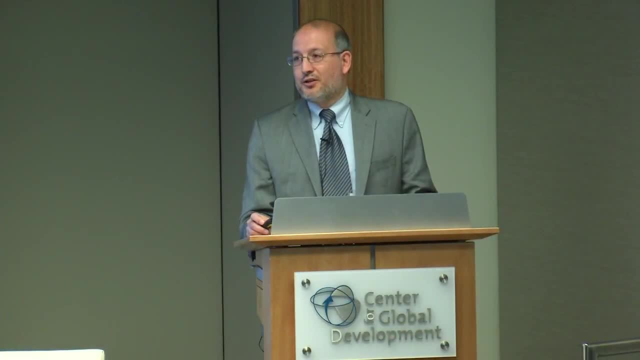 to conduct and to organize and regulate the work of the national statistical systems. These dimensions determine how the NSO interacts and works within the state, But it's also necessary to understand how the work of the NSO impacts the capacity of the state. So, as you can see in this graph, you know the capacity. 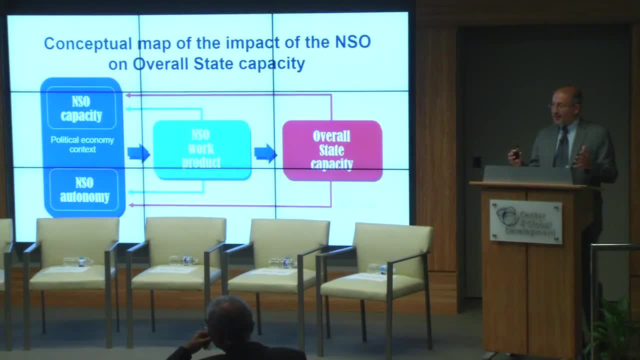 of the NSO is determined by the political economy. on the context in which the NSO exists. This capacity translates into the ability to produce data. This data impacts the overall status and capacity of the state, And then the capacity of the state feeds back to the capacity of the NSO. 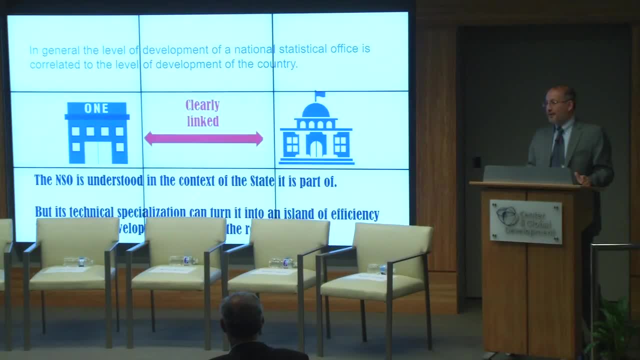 And this is key because, as expected, the level of development of an NSO, of a national statistical office, is correlated to the level of development of the government in that state. However, what the book shows is that the technical specialization of these institutions 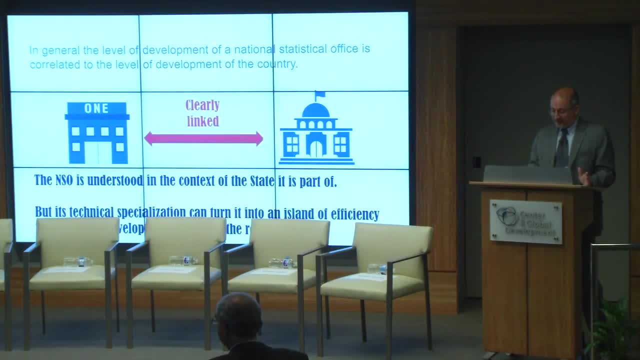 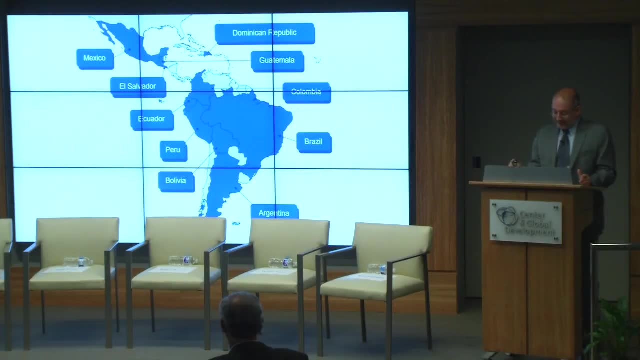 gives them the opportunity to become islands of efficiency In the government, that is, to have a higher level of development than the rest of the institutions of the state. And it's exactly, you know, understanding this divergence that has been, you know, was one of the objectives. 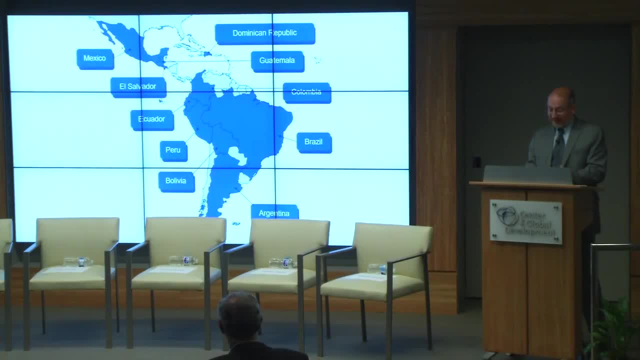 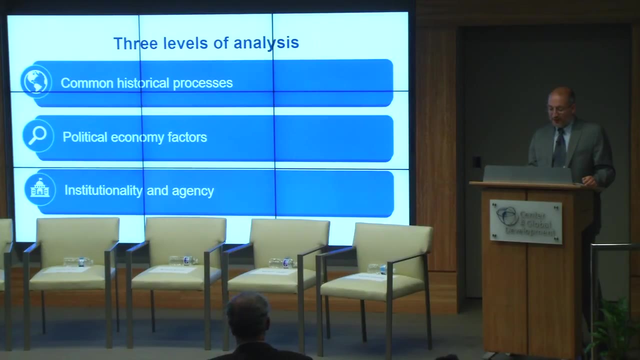 of the book And to do it, the authors analyzed 10 case studies in the 10 countries listed in this map in Latin America, which have very different levels of statistical capacity And the. you know there are three levels of analysis for the results of the. 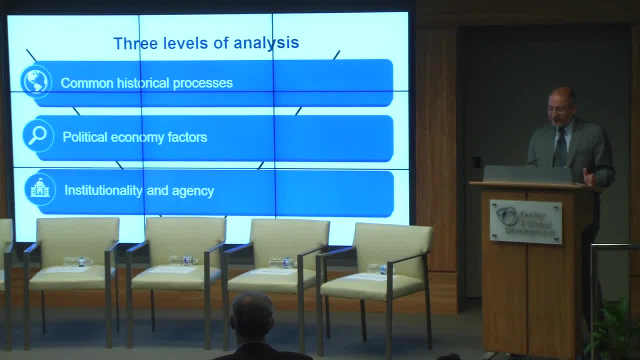 of the books organized, you know, from general to specific. First, common historical factors, processes that are found in many of the case studies. Second, the political economy factors that have some similarities about some of the around some of the case studies. 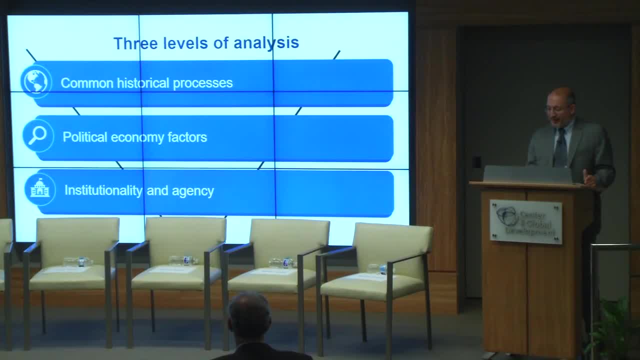 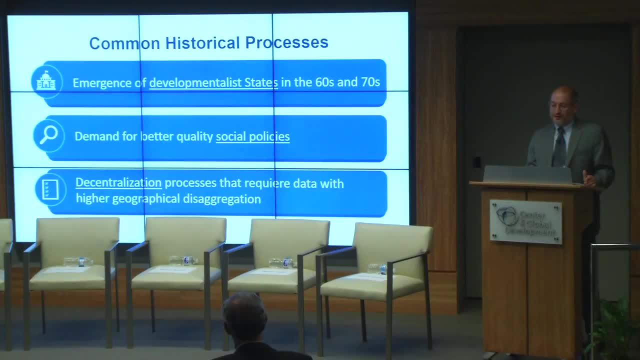 And finally, you know the country-specific elements that reflect the experience of particular institutions. So let's start with some of the common historical processes that have strengthened the statistical capacity across the region. in these 10 countries that we looked at, You know many NSOs can trace their origin. 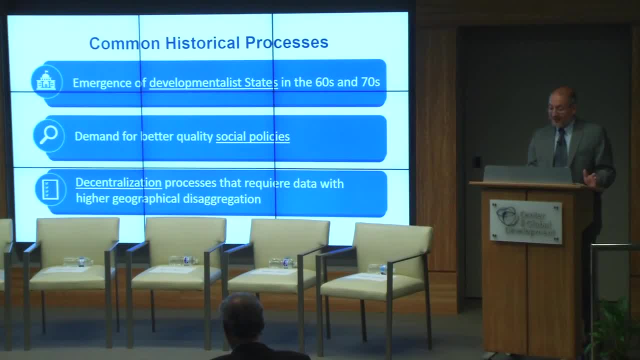 to the emergence, in the 1960s and 70s, of developmentalist states that put an emphasis on planning, And you know this emphasis on planning resulted in an investment in statistical production. More recently, you know, these institutions have gotten a boost with the advent. 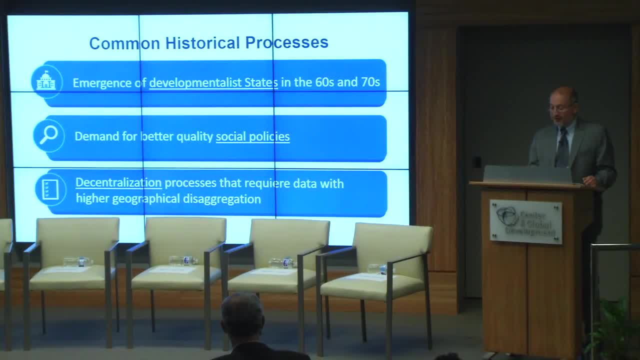 of better quality social policies, such as conditional cash transfer programs. You know social policies that imply a very high demand for data and hence again an investment in data production. Another positive impact came from the increase in demand for data with a higher level. 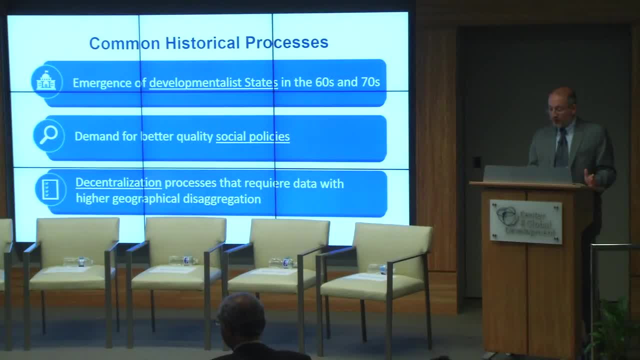 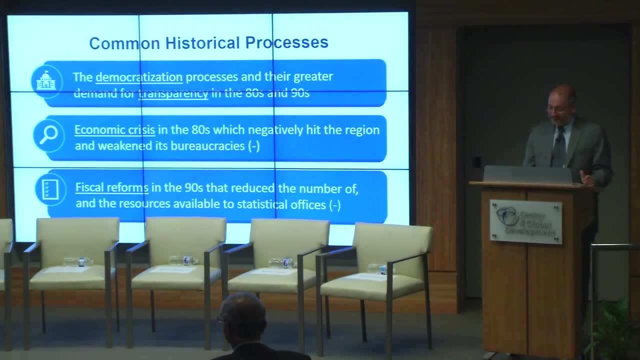 of geographical disaggregation that came as a result of the decentralization processes that some countries underwent In the 80s and 90s. the democratization process in the region implied a push for greater transparency, which had a positive impact in statistical capacity. 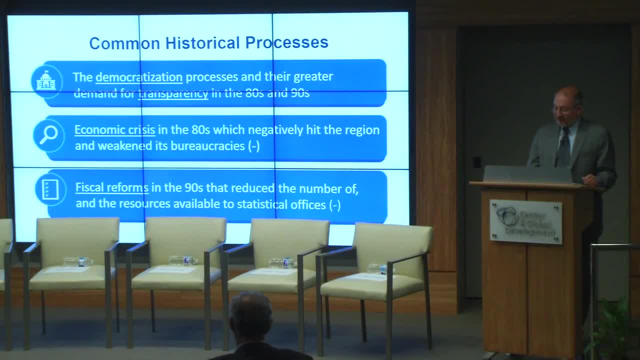 However, you know there are also some, you know some common historical processes in the region that had a negative impact on statistical capacity. Among them, you know the economic crisis of the 1980s, which weakened bureaucracies and the state in general. 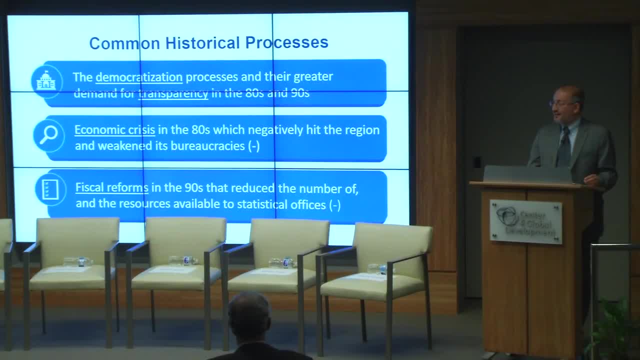 and the fiscal reforms of the 90s, which reduced the number of statistical agencies within line ministries and sometimes it also implied a reduction in budgets for the national statistical offices. Moving on to the political economic factors you know, let me highlight a couple. 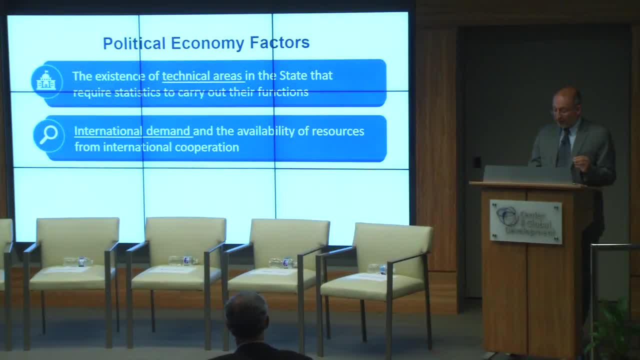 As said earlier, you know, the statistical capacity of the NSO is directly correlated to the capacity of the rest of the state, of the rest of the government. So the existence of technical institutions within the government that demand data has a positive effect on the statistical capacity. 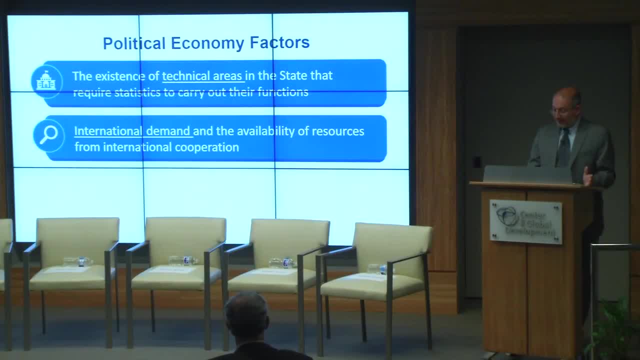 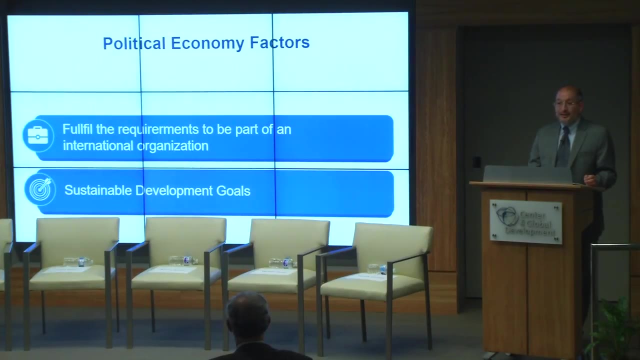 Another element that has a positive effect is the international demand and international cooperation. Now we see that the active participation of multilateral agencies has an important impact on the statistical capacity, And let me mention just two examples: The need to fulfill certain requirements to be part of an organization such as the OECD. 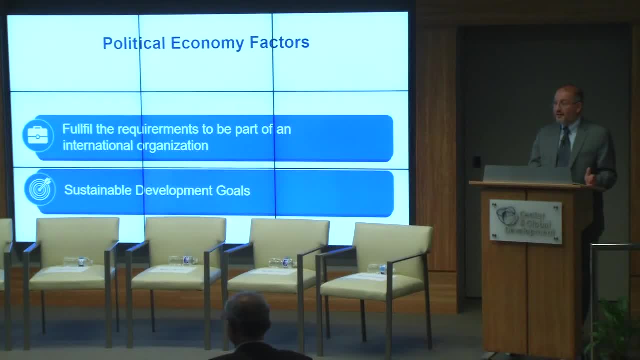 or the need to be part of the IMF. the Specialized Data Dissemination Standard implies the need to invest in better data and in data production Or in other levels of development, the need to report progress in certain areas, such as it was with the Millennium Development Goals. 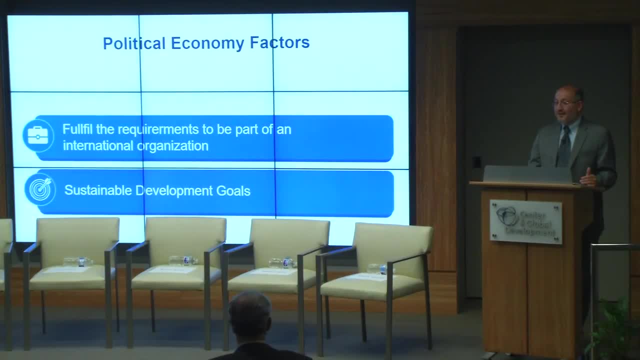 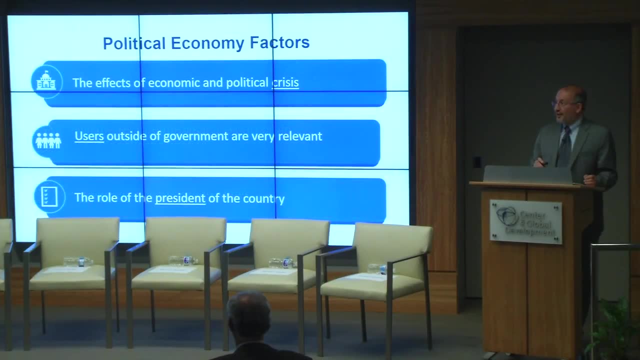 and, as it will be with the Sustainable Development Goals, It's an incentive for countries to have more resources, and more resources into national statistical offices. Other political economy factors that impact are the effects of political crises in particular countries, The high levels of demand from outside of the government. 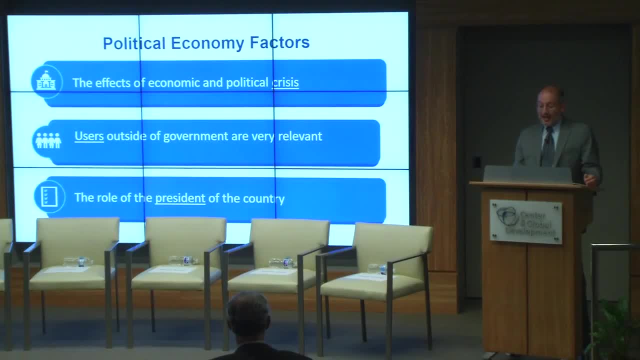 are very relevant to increase the statistical capacity, And having a high level champion that believes in data can have can influence the statistical capacity in a positive or a negative way, depending on the mood of the champion. We saw that in a couple of the 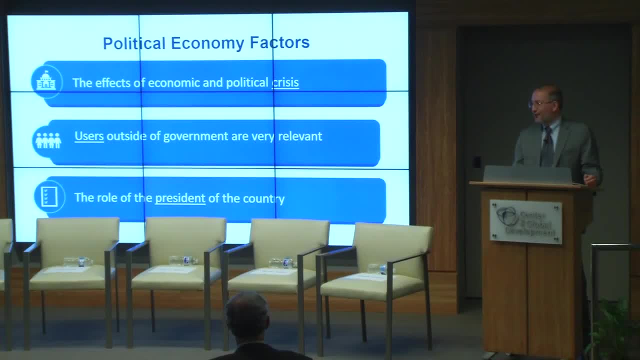 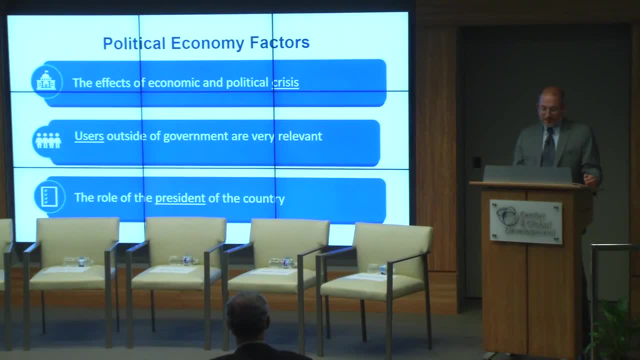 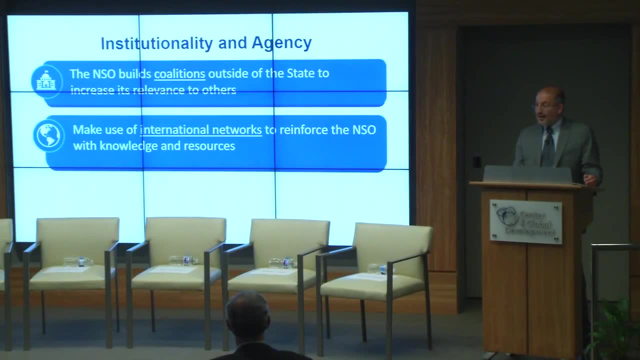 and, in some cases, limiting the developmental statistical capacity. Finally, the more specific findings from this study refer to elements that are in direct control of the national statistical office, And among them are that a way to increase statistical capacity is for the NSO to build alliances. 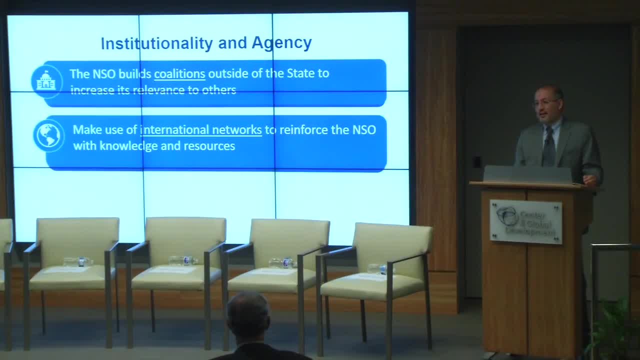 with data users outside of the state, such as academia and civil society and the private sector sector, And you know, because of the technical nature of the work that the NSOs do, there is a strong international community of national statistical offices and it is important for 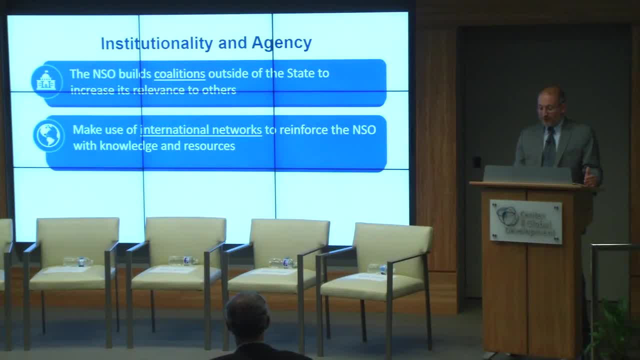 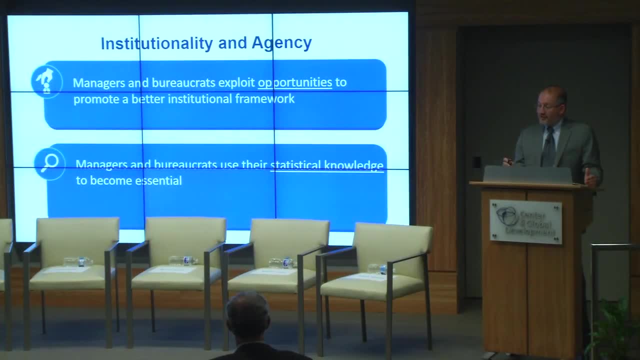 local, national statistical offices to take advantage of this as a way to reinforce their knowledge and resources, to take advantage of what this community has to offer, Specifically in terms of the role of leaders and managers within these agencies. you know they can take. 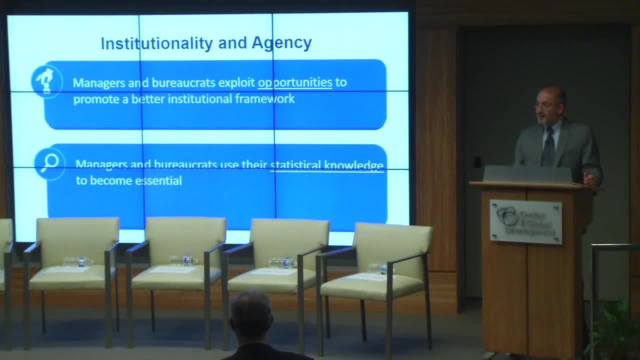 advantage of opportunities to influence decision makers and push for better institutional frameworks. you know giving particular opportunities when they see particular opportunities, And managers and bureaucrats can also use the technical expertise of the NSO to make it essential for the rest of government, since no other institution, usually in the country, has the 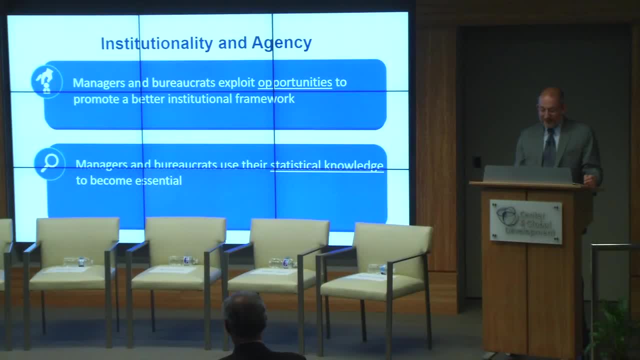 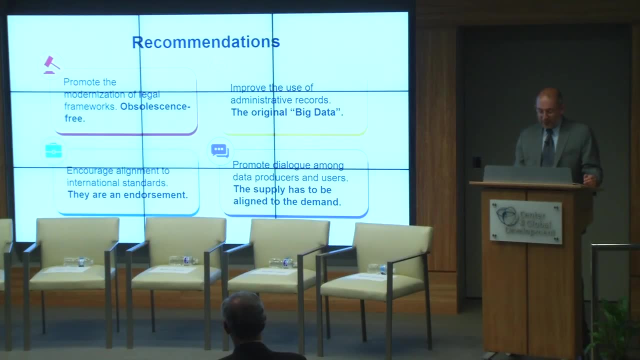 technical capacity to produce the data that the NSO produces. In terms of a recommendation, the book presents proposes a following. I'm going to mention Some you know. one is, you know, to promote modern legal frameworks for NSOs In Latin America. 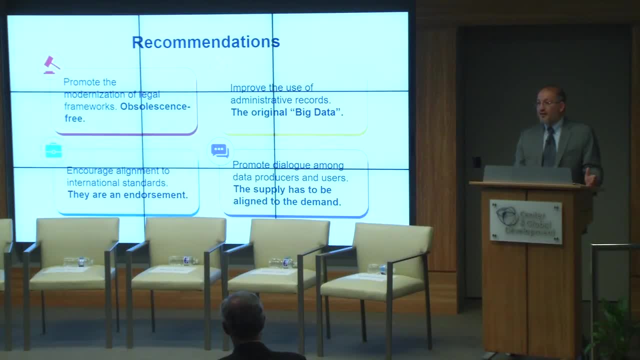 and I see in, maybe in the, as we see in the rest of the world, we have legal frameworks from the 40s and 50s. You know they are really, you know, behind times, even when, even with dealing with 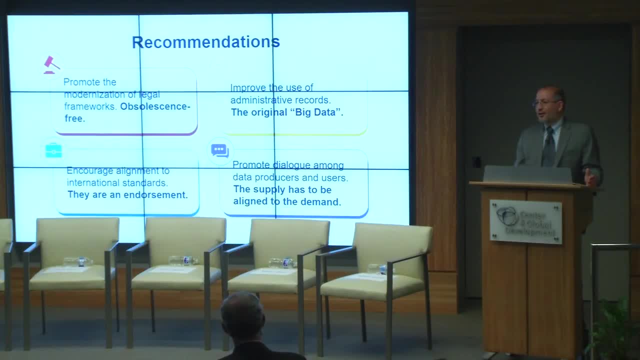 you know a simple factor of how to store data And you know they talk about having to store paper for 10 years or 15 years, And you know this modernization of the legal frameworks is important because it's very relevant for the coordinating role. 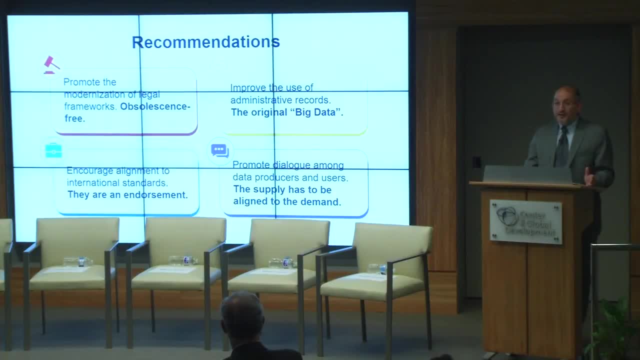 Of the NSO within the national statistical system and also for its interaction with data producers outside of the government. Another recommendation is to improve the use of administrative data. you know the original big data. You know, first we have to concentrate on the things that we already have in hand. 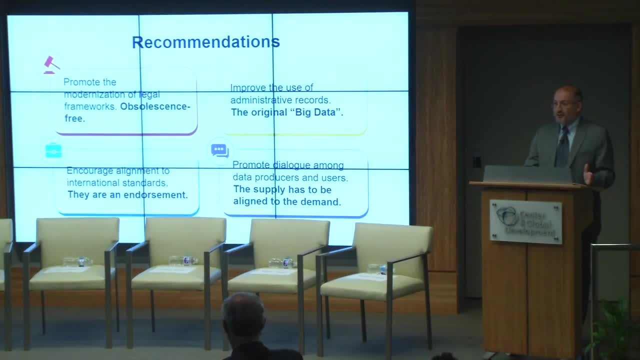 Another one is to encourage the alignment to international standards. You know, aligning to international standards can serve as a protective barrier for these offices. So when somebody questions the definition of unemployment or the way that the CPI- you know the the price index- is measured, one can make a reference that this is. you know this is because 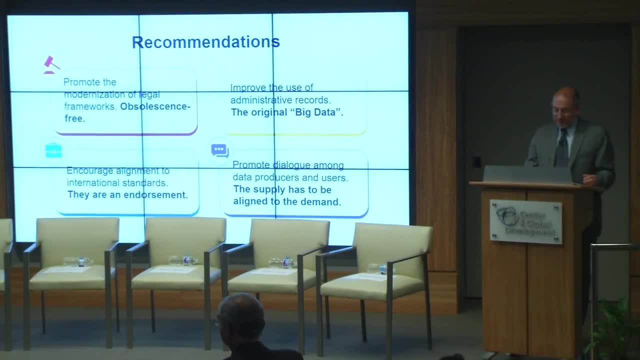 such and such international organization defines unemployment or the price index in such a way. Another one is to promote a dialogue among data producers and users. You know it's necessary that the supply of data is relevant to data users. It's necessary to promote transparency in data production and to increase data dissemination. 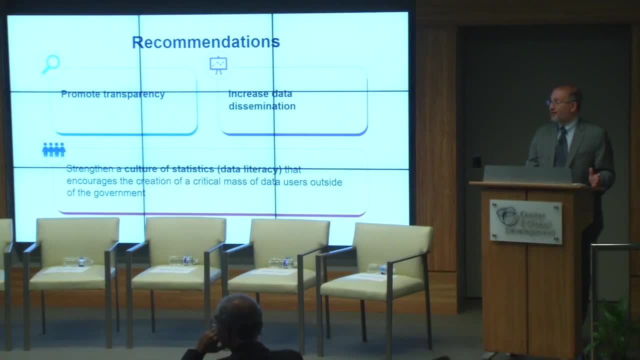 And, at the end of the day, what we want is to strengthen a culture of statistics. You know what some call data literacy. You know a culture of statistics that encourages the creation of a critical mass of data users outside of the government. 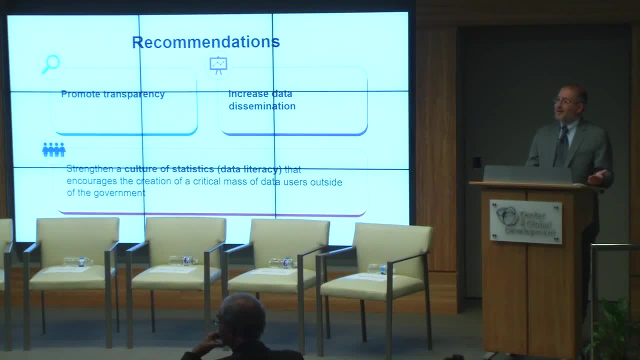 You know, it's not only the, the statistical office have to depend not only on the demand from within the state, but also from the demand outside of the state. And it is this demand outside of the state that, in the case studies proves, in the case studies, proves to be very relevant, relevant. 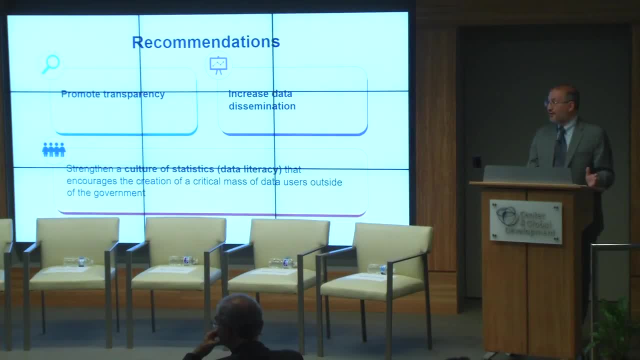 Of course, these recommendations are drawn from the experience in these 10 countries, but we hope that they can apply. they can be applied to other, to other places in the in the world And of course, you know there are there are challenges. 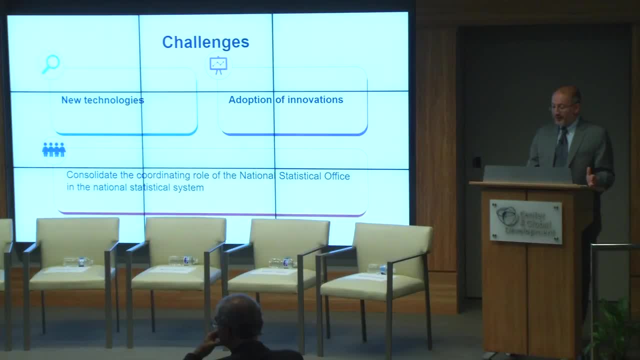 And among them, you know, the incorporation of new technologies in the data production process. It's necessary to understand that technology is a tool, but it's not the goal. Another challenge is the adoption of innovation In general. what we see is that national statistical offices are very conservative and cautious when it comes to change the way things are done. 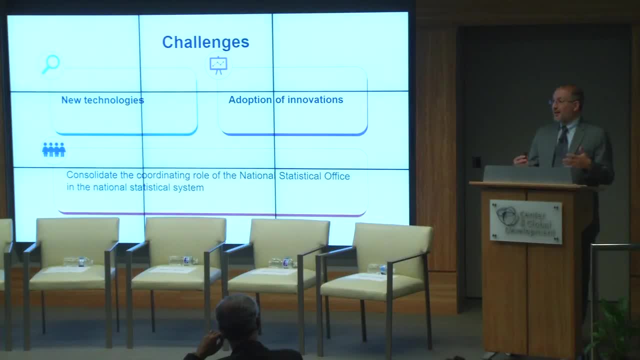 You know Santiago was mentioning the use of tablets for data collection. Recently, in the last year, in Latin America, we saw two countries that went back to doing the census like it was done 50 years ago. You know where everybody had. you know there was a everybody. nobody could move from their houses. 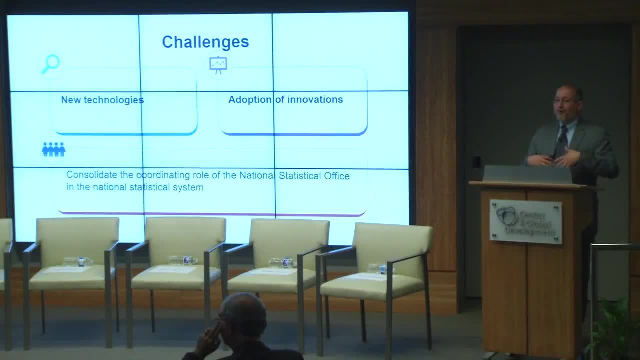 and they had to stay in their houses for one whole day while an army of half a million people went through the country collecting, collecting data. Another challenge is, you know that there's a need to consolidate the coordinating role of the NSO in the national statistical, in the national statistical system. 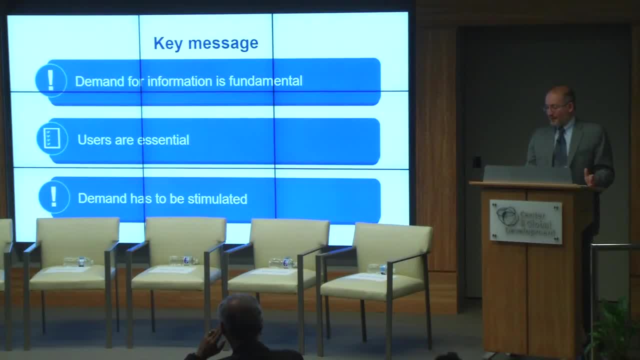 And if I have you know, to conclude, you know there's one key message: Demand is fundamental. Hence users are essential. And users, you know, when we talk about users, we talk about users not only within the government. 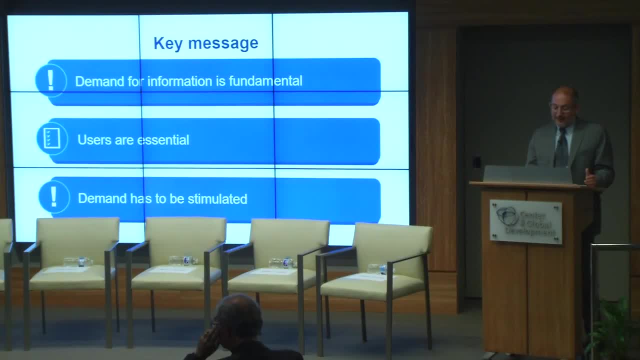 but particularly users outside of the government and outside of the country. But demand needs to be stimulated, You know, there needs to be a flow of information so that users- users- can take advantage of it, And what is needed is the existence of a critical mass of individuals and institutions that will complain. 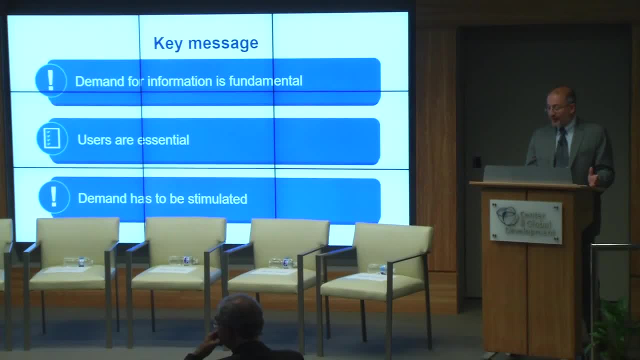 when data is not related, related to data That is, according to a pre-agreed calendar. Individuals and institutions that will protest when methodological changes are not transparent and discussed. Individuals and institutions that will grumble when a statistical product is not funded. 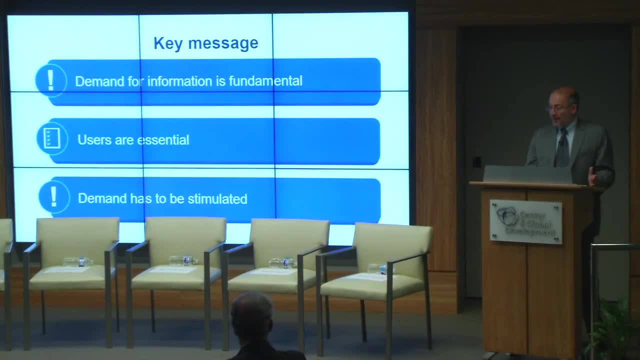 The NSOs need grievers. needs grievers that will cry when bad things happens and funds that will support them in good times. Now, something you know, I you know when, things you know, when a new question is introduced in the census without any you know. 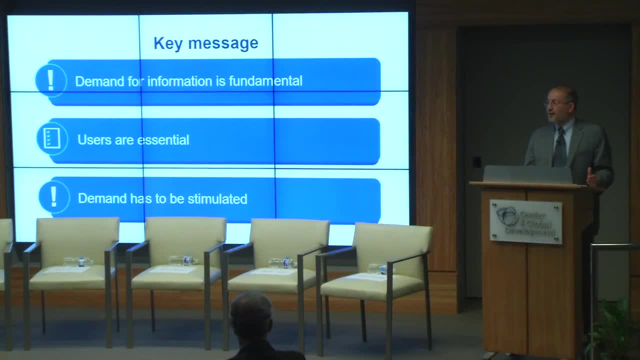 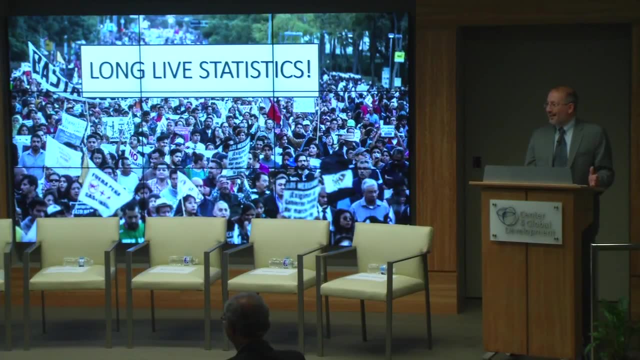 without consultation, or a or a, a survey is not funded anymore. you know, this is what I would like to see in the streets. No, You know, really a mass of users that are willing to, to protest and to defend the statistical agencies. 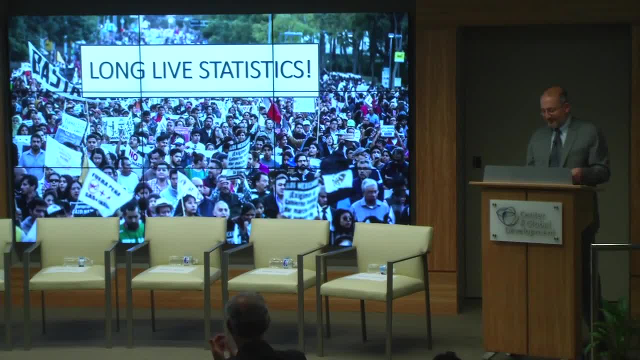 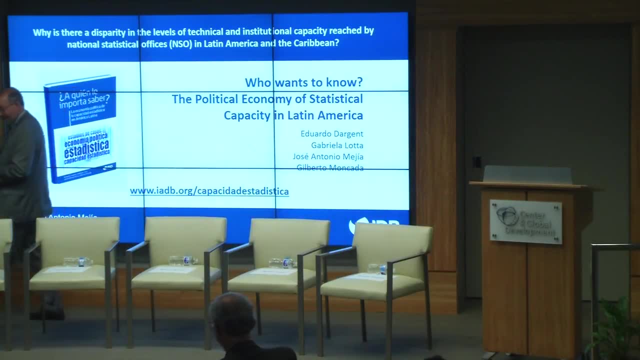 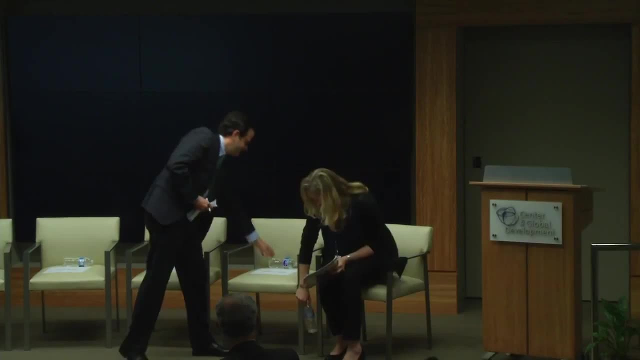 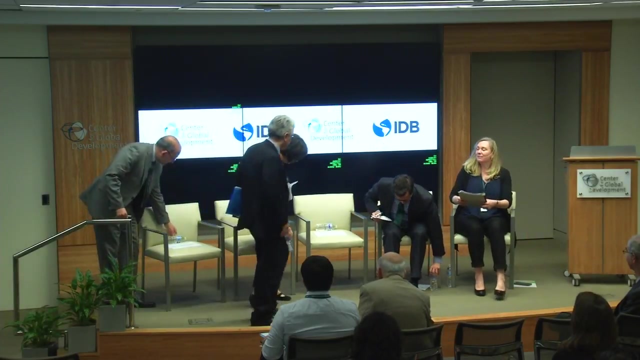 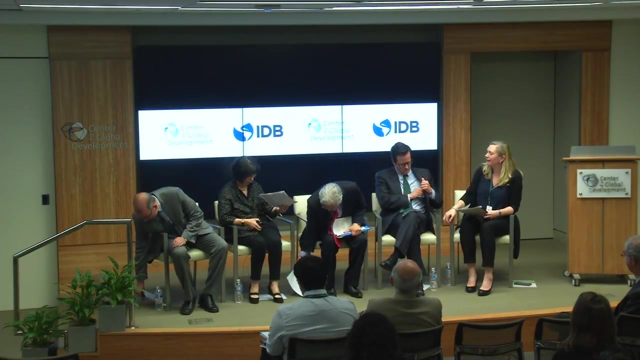 Thank you. So you're you're suggesting that data revolution take to the streets, No longer in the conference halls. Okay, Great. So let's get a round of sort of general responses to what you've heard and read so far related to this report. 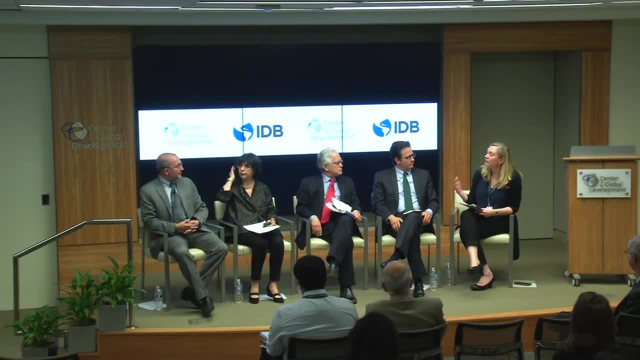 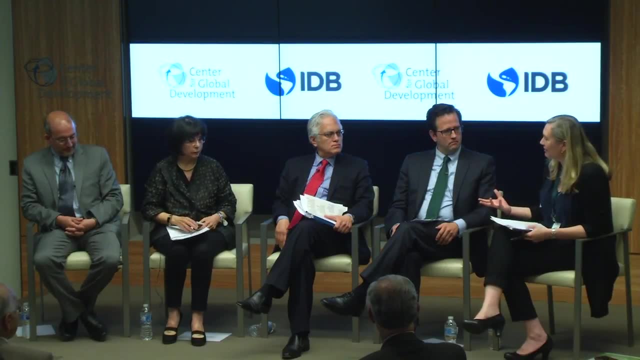 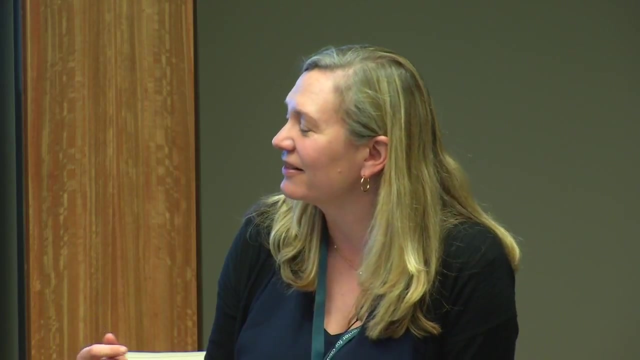 I I was struck by the emphasis on user groups and how that creates a constituency for the accuracy and availability of data. One of those constituencies are organizations like the Inter-American Development Bank or the World Bank or the IMF. So maybe you could reflect first on that big finding with this role of standards user groups. 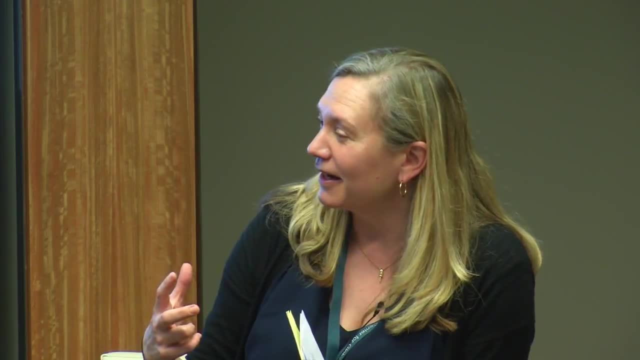 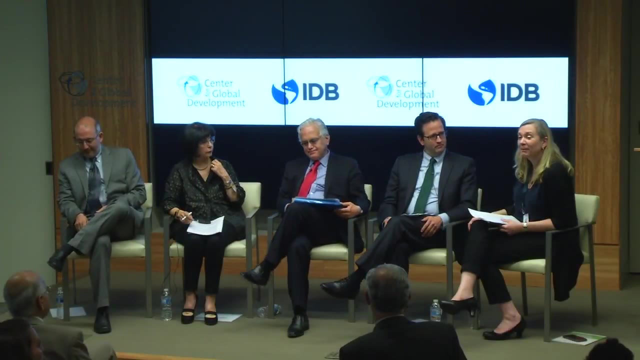 Maybe you could also talk a little bit about how this would compare to other parts of the state. Maybe I can start with you. Sure Matthew's a professor- an associate professor- at American University, who's focusing on state capacity and and looking at NSOs in that context. 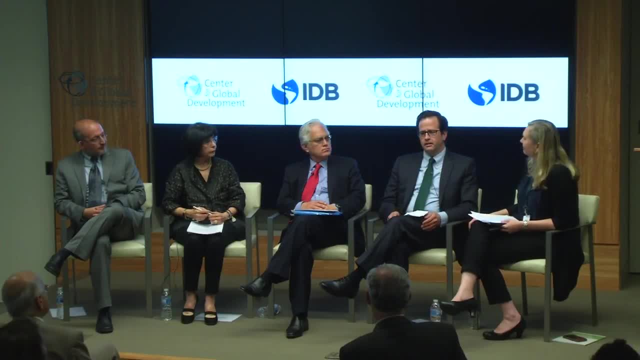 Definitely Well. first of all, congratulations on the really marvelous book. I think that the Jose Antonio would never say it this way, but the key message here is there needs to be proselytizing by international bodies, And I think part of the reason for that is that state capacity is both de jure and de facto. 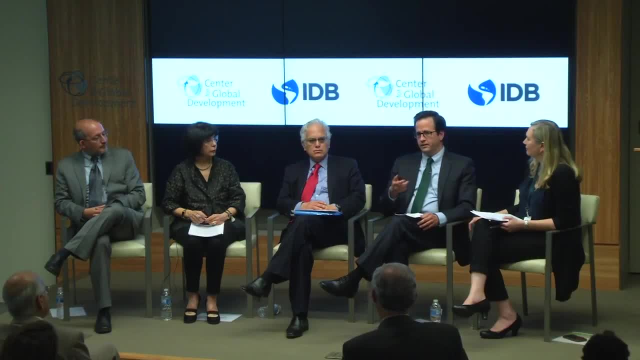 And so, in order to actually achieve statistical capacity, it's not just sufficient to have data, It's not just sufficient to have laws on the book. We saw this in Argentina. There's a case study on Argentina in the book, which is marvelous, looking at what happened with INDECI. 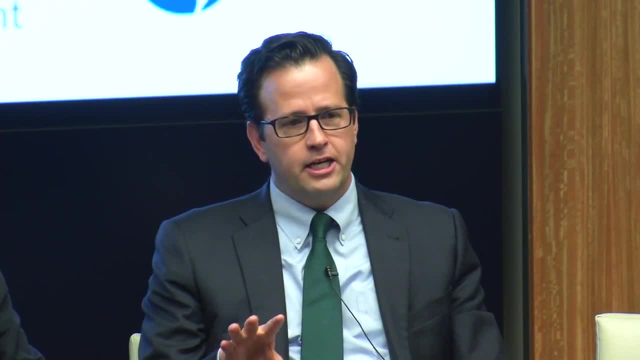 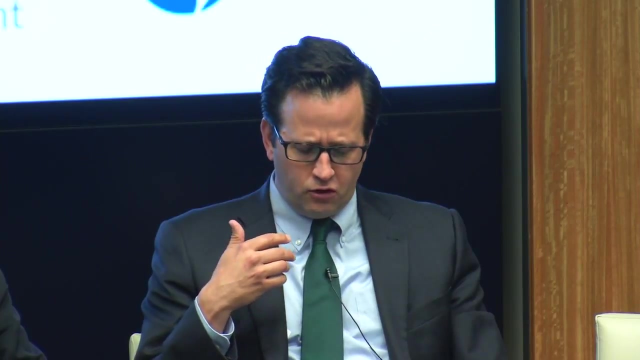 And the degree to which the laws on the books didn't change but the de facto rules did, And so I think that proselytizing, creating the client base which Jose Antonio mentioned, is really essential to making this happen And, in terms of de facto, 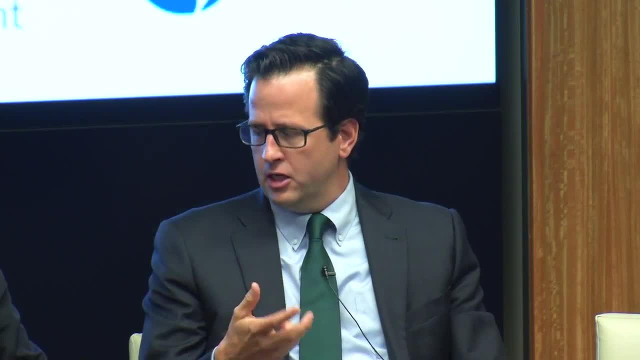 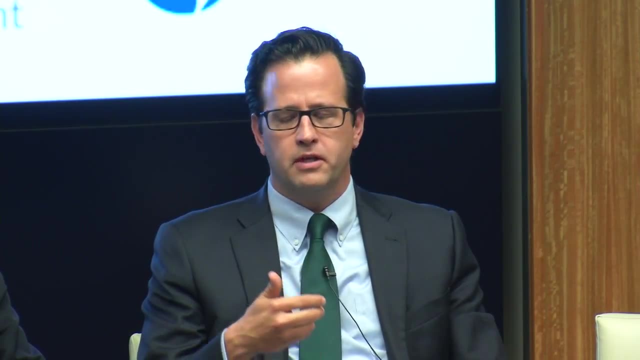 guarantees of statistical capacity. legitimacy is central. So there's the demand side and there's giving legitimacy to the statistical agency because we know that the results are credible and because we know that they're replicable. Maybe I'll go to Shida now. 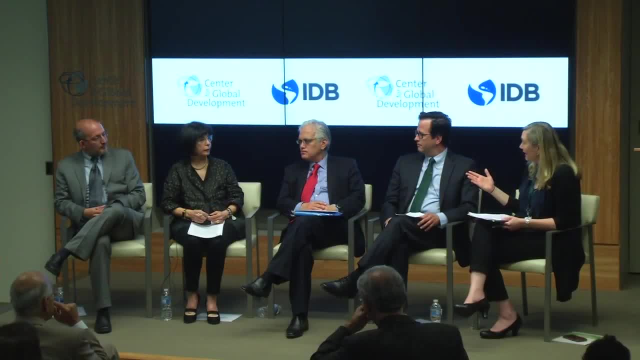 Shida Badia is the CEO of Open Data Watch, but she was also the data for development director at the World Bank for many years. Can you reflect a little bit? You've both been civil. You're civil society now. You were the World Bank before. 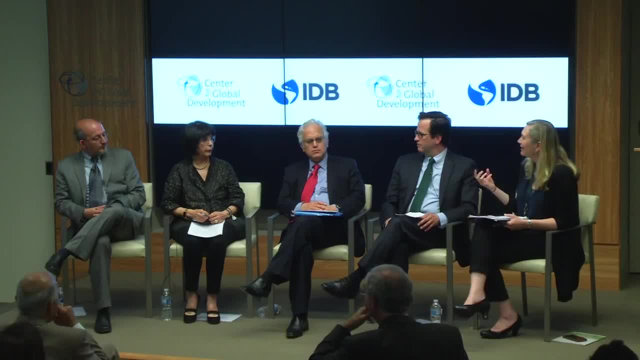 How do you see this issue of users and the constituency? How does it relate to capacity? Well, thanks, Amanda. First of all, congratulations to IDB and, of course, to Jose Antonio. This has been a really terrific book because I've been a long time- maybe close to 40 years now- in the business of data and capacity building. 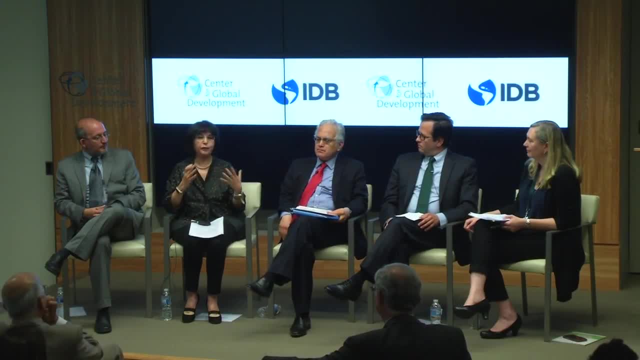 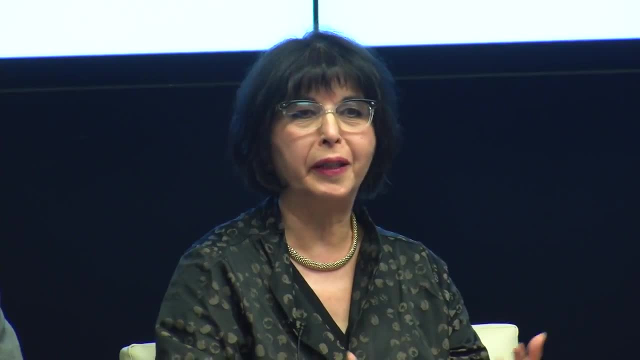 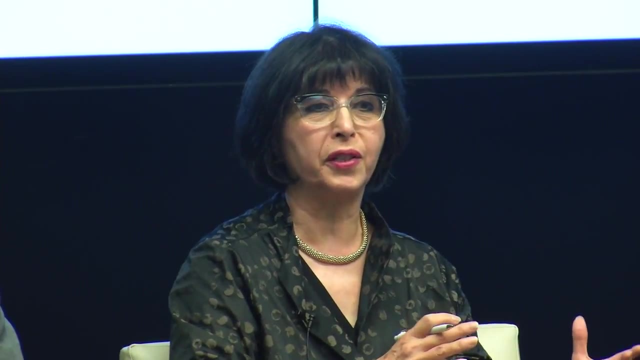 And I think we really need to take a fresh look at this And we need a reform. Some of us are advocating for what we call statistical capacity development 4.0. And that, as part of that, we really need to look at. we've been very much focusing on the production side and the technical side of capacity building. 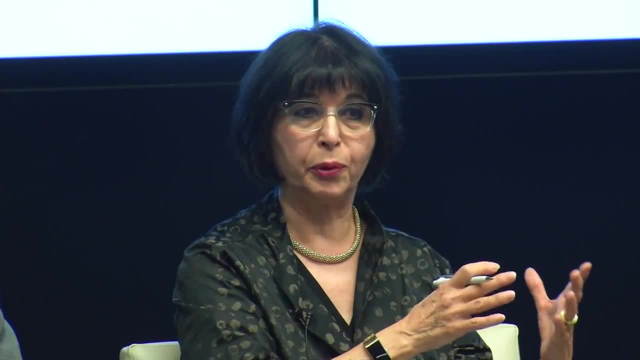 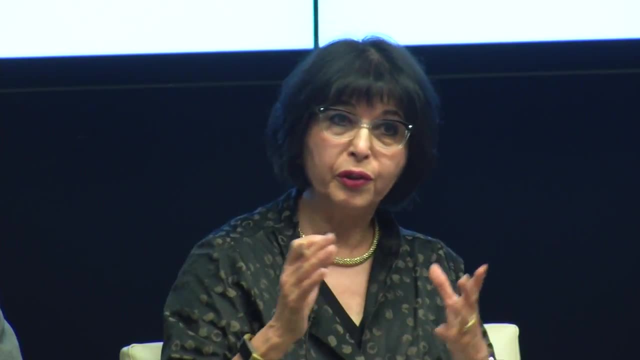 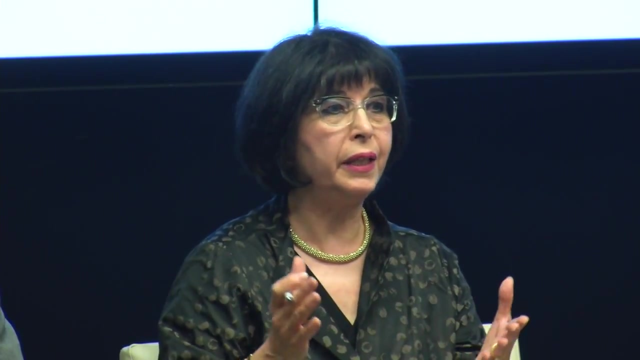 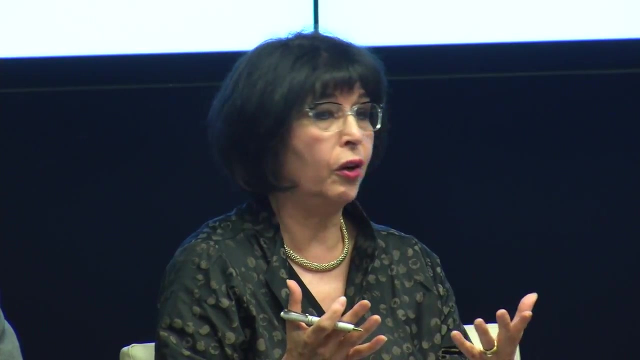 What I call this sort of in the value chain of data very much at the production level, rather than going more into the uptake and impact And you know policy And for doing that, for getting the data and the value of data down to the value at the impact level. you really need to be much more smarter about understanding the political economy of data and the context of data. 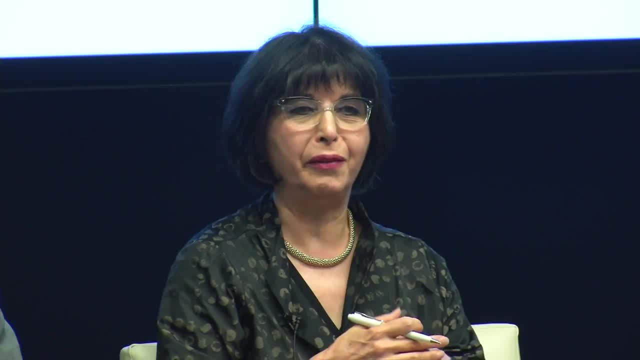 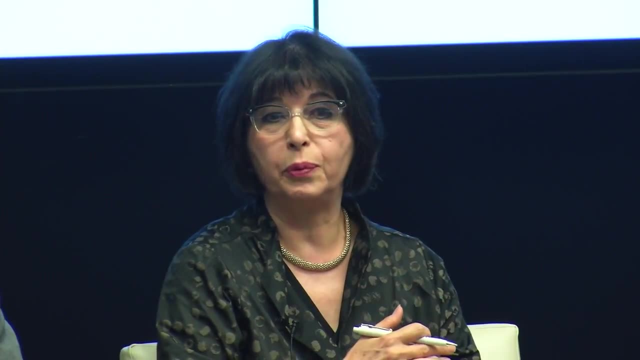 And believe me, it comes from a lot of experience in the field- that if you ignore it, you basically it's like you know you produce the machine that you really don't know what is working Right, You don't know what its use is going to be. 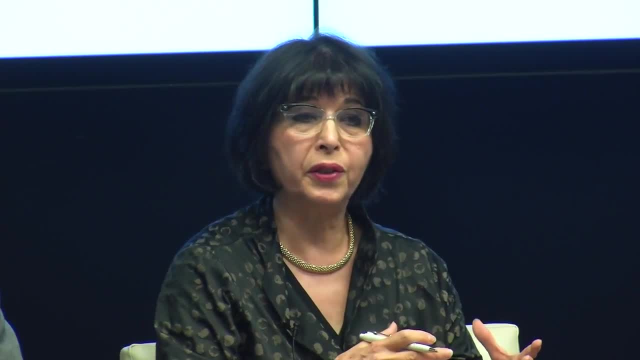 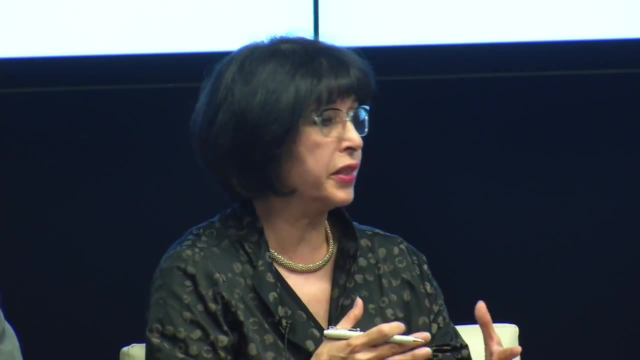 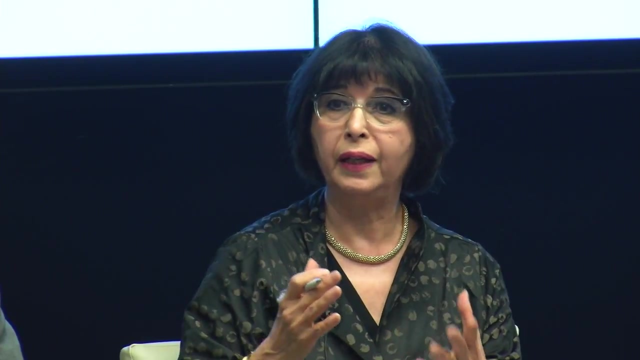 So I think this really sheds light on the importance of the demand side, importance of users, importance of building leadership for statistical capacity building And, I hope, also the time. I think is right, because a lot of organizations, UN and countries are thinking about reforming the statistical system to respond to SDGs. 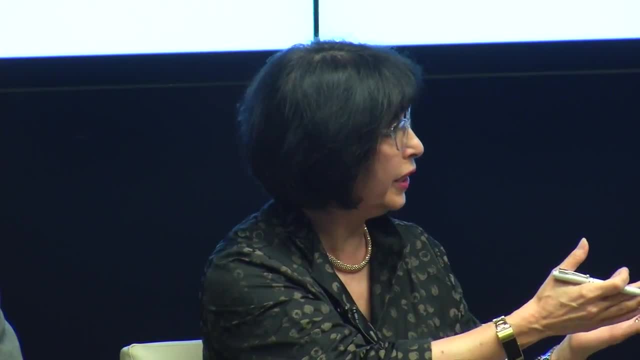 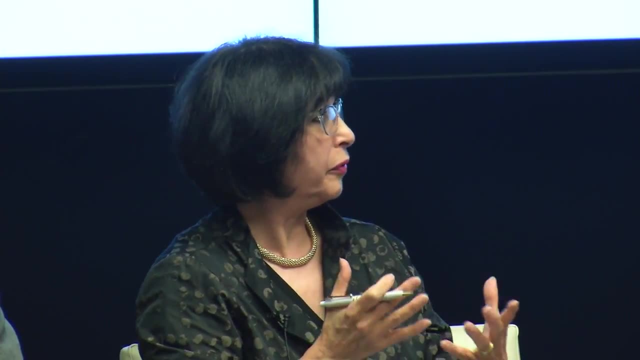 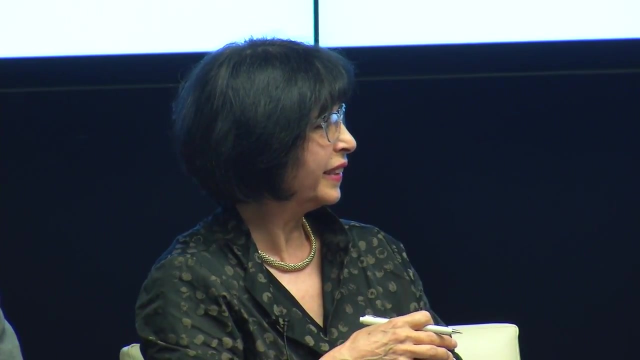 So I think it would be really a good time to advocate within organizations like this, Organizations like the World Bank, OECD, UN, even IMF, of taking these factors much more into the consideration in designing their capacity development work Absolutely, And I mean making sure that capacity development work is adequately financed and prioritized is obviously a key part of that. 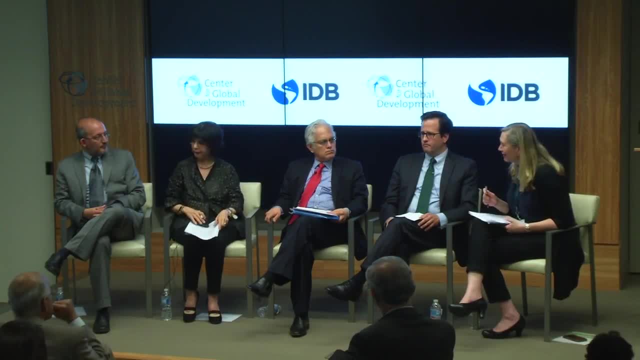 And we'll come back to that issue with you and Jose Antonio. But, Roberto, what about? so we've talked about standards as a kind of pull mechanism To get better accuracy and availability of data. You've been doing some work at the IMF on this very topic. 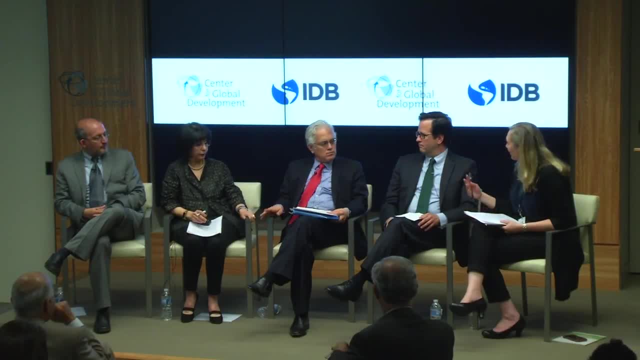 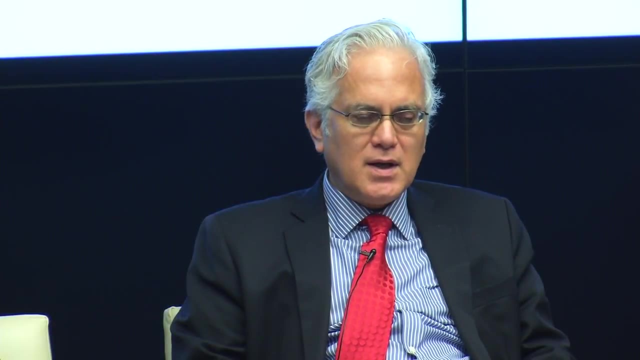 Do you want to reflect on that and how that's worked in Latin America? Yeah, First of all, let me congratulate Jose Antonio and the IDB for an excellent book. I think, in my opinion, this is probably the first time- an institution such as the IDB looks at this in a very structured way. 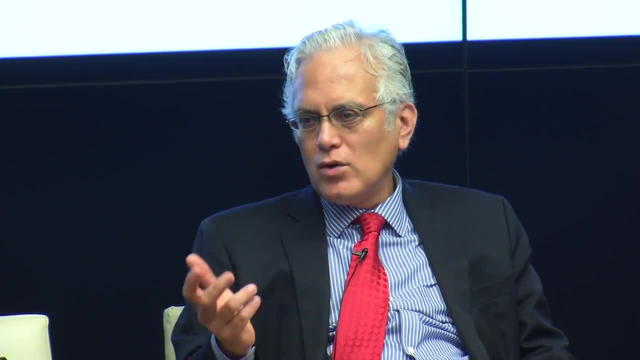 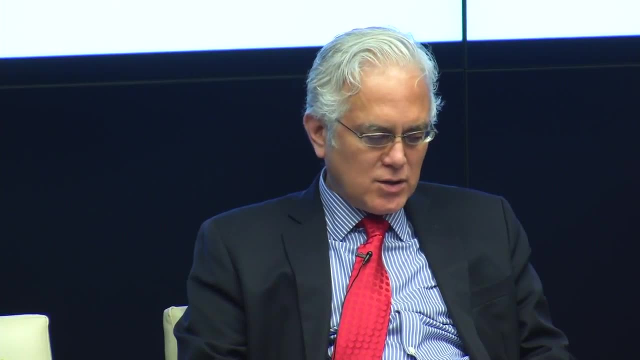 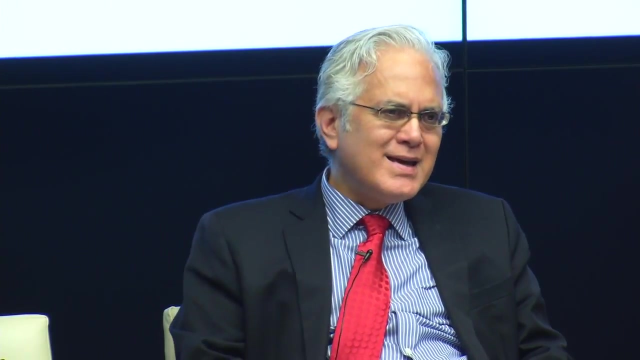 The second thing I would like to say is that we pretty much agree, That we pretty much agree with all the conclusions and findings of the book. I think the emphasis on the legal and institutional framework is right, on The same resources and the topic of interagency. collaboration is essential. 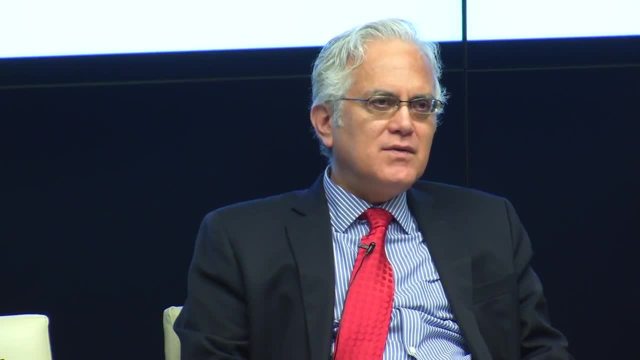 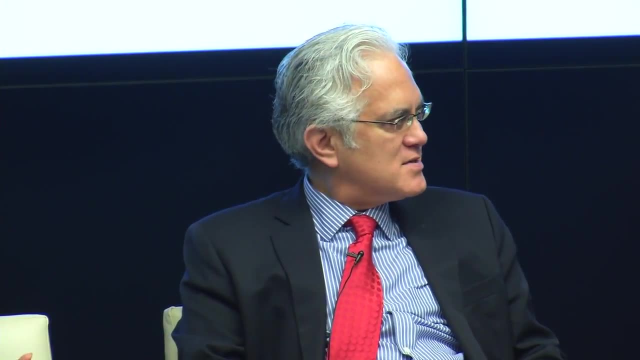 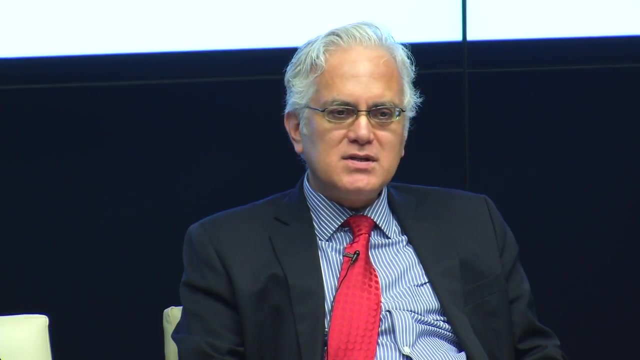 I would like to perhaps take a different view with regard to the users, And this has to do with what Santiago was saying in his remarks: Wow, You know. today, I would argue that the demand for statistics is infinite. Everyone wants more statistics of every kind. 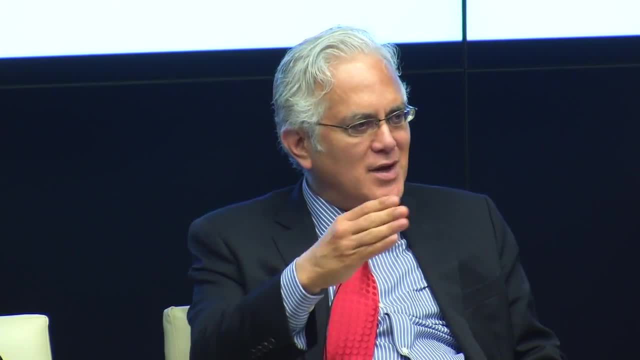 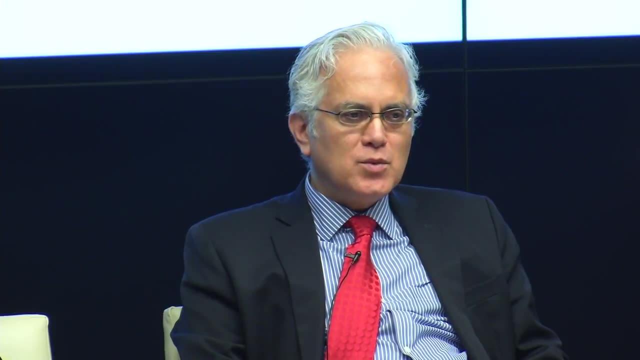 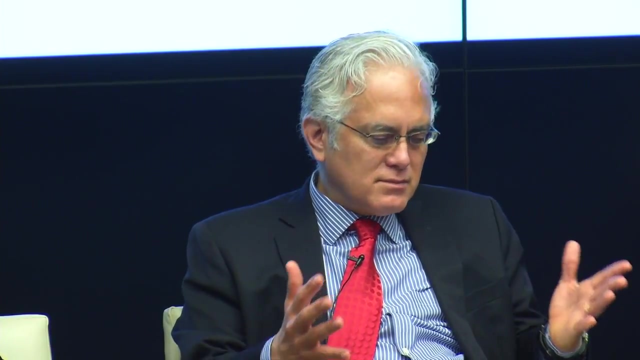 You can ask every minority group in every country and they have their own agenda for statistics. But I think that there is a ranking of users And I would put at the top of the ranking the policy makers. Traditionally, the resources and the statistics have been relatively scarce. 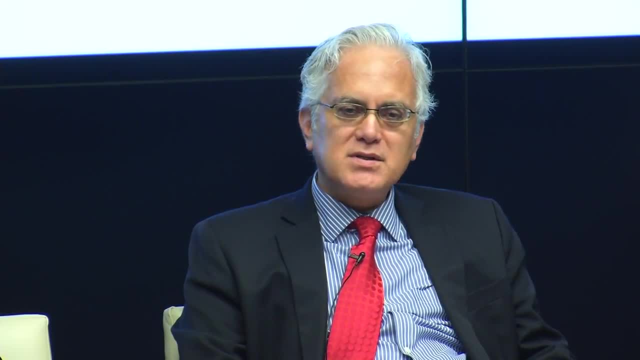 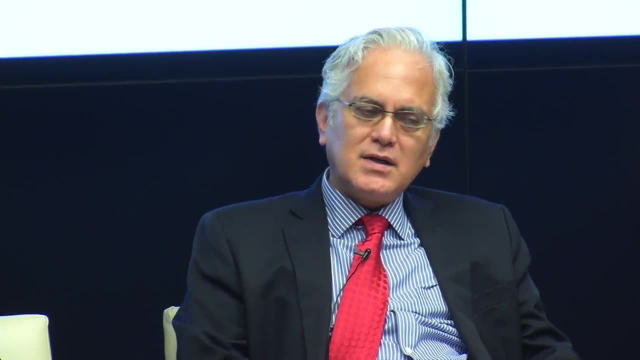 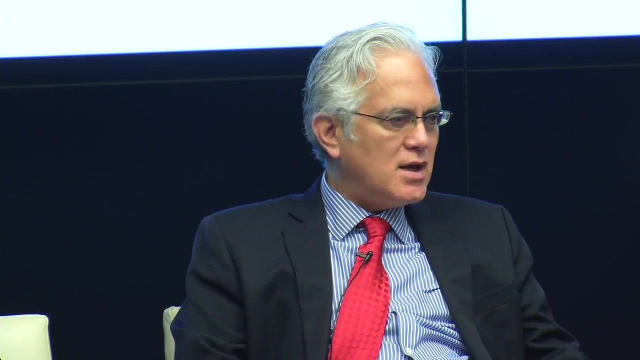 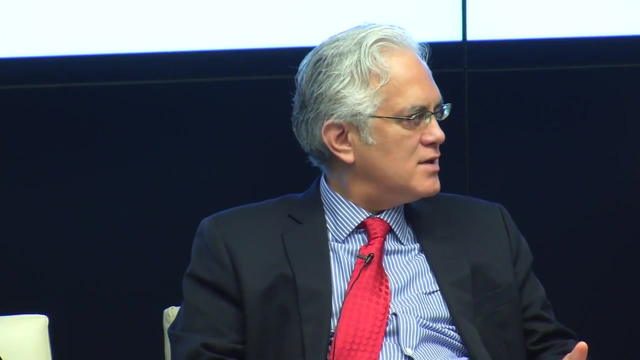 And the ministers, the cabinet and the president have preferred that the statistical offices- not only the NSO, but also the statistical office of the central bank at the different ministries- focus on the data that are needed to formulate policy making, And so, from that point of view, I am not so sure that we have plenty of resources to do everything that is needed. 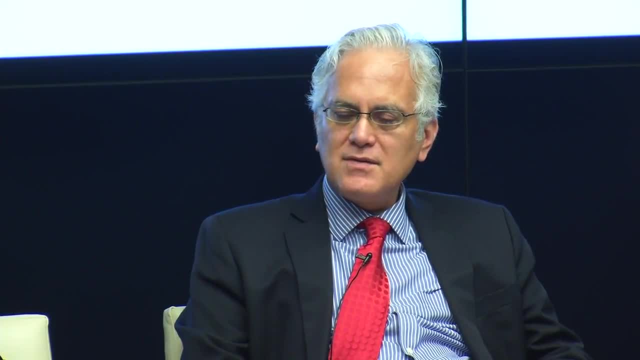 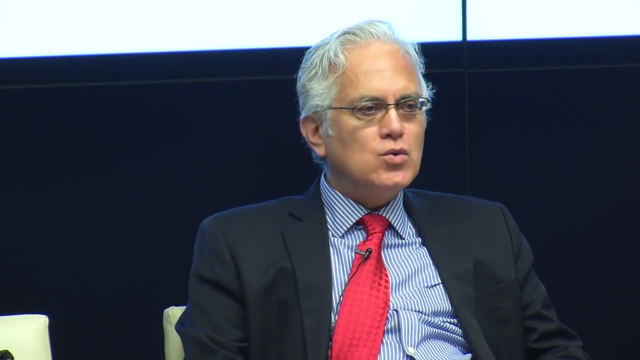 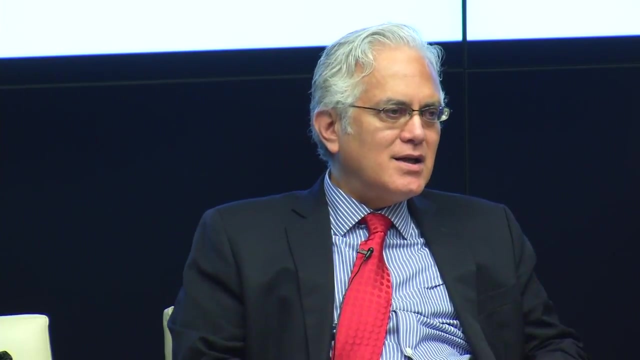 In our case, in the case of the fund, we have, since the 1950s, we have been providing capacity development everywhere, trying to enable countries to calculate the balance of payments, the government finance statistics, the essential data that are needed to formulate and monitor financial and economic policies. 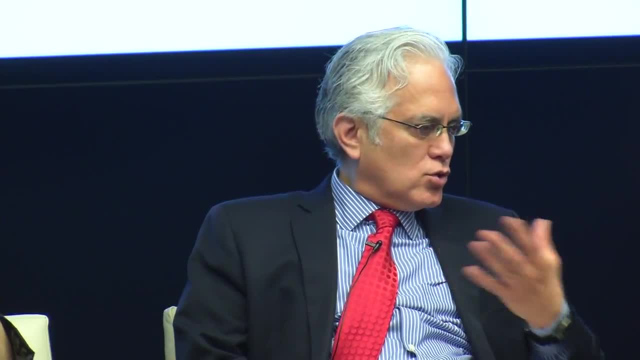 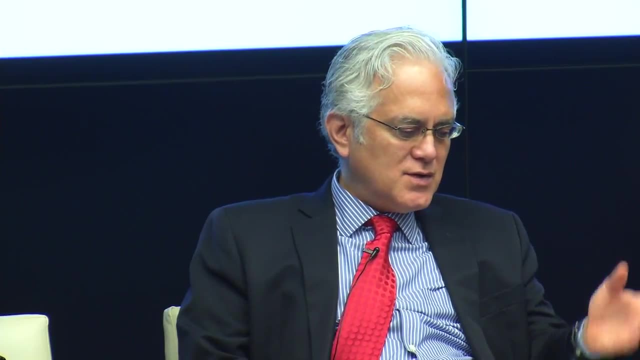 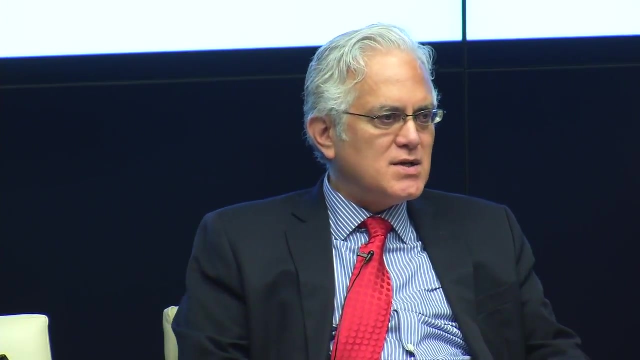 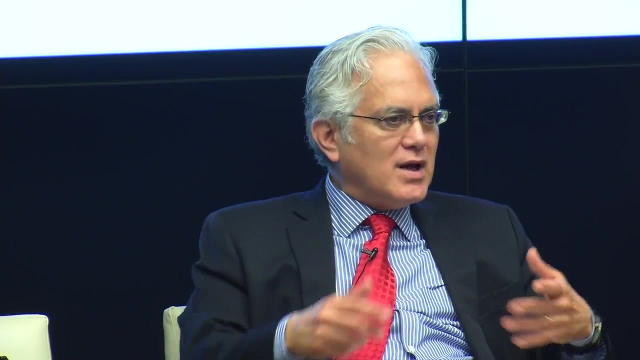 Today the demands that you know, not only in Latin America. I've heard the chief of the UK statistical office and the chief statistician of Canada essentially say that the demands they have from what we call today civil societies are enormous And, frankly, not all policy makers agree with the agendas of these different groups. 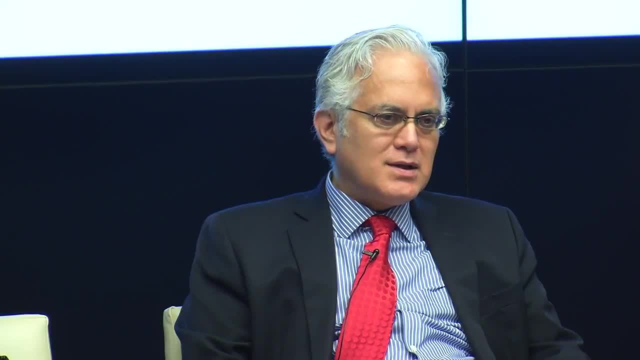 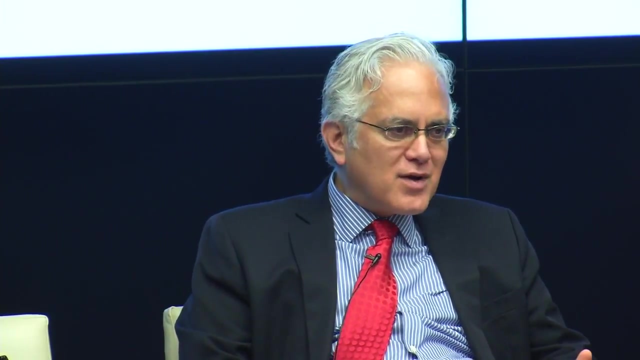 I would also postulate that Latin America is not identical to Europe, to the UK, to Canada, to Australia, when it comes to social and cultural conditions. What is possible in those countries may not be possible or preferable today in Latin America, So one needs to take that into account. 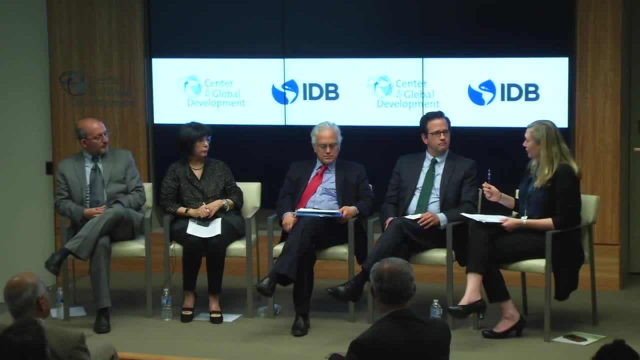 And let me push you a little bit on that, on the role of the international organizations in keeping that focus on policy makers at the center. You know it's good to have the standards and the standards themselves a protective factor against like political meddling, for example. 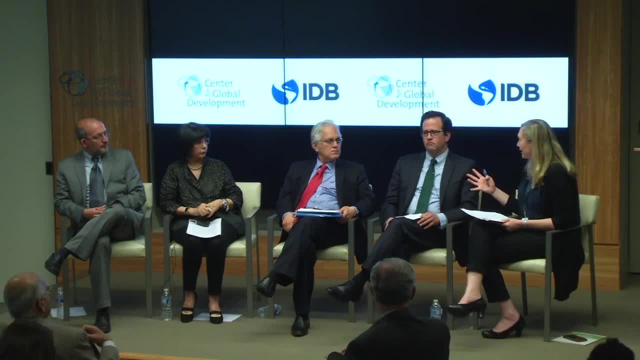 But let's take, for example, the 2011-2012 Argentina inflation. This is a famous case where sort of everyone knew there was a problem with the numbers, but it wasn't the international organizations that came out and said something about that core statistic of total value to policy makers. 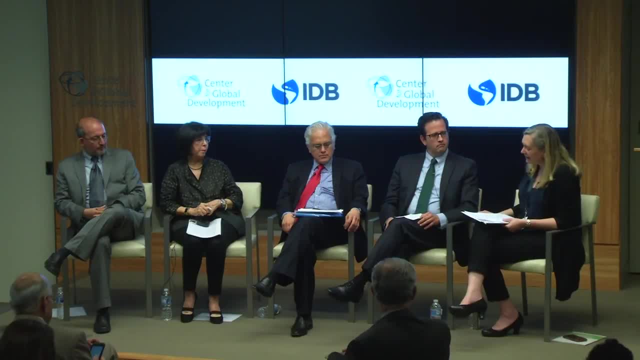 as well as other groups in society. So what is the role of the international organizations when it comes to this kind of data? Has it changed over time? I would say that both the case of Argentina and the case of Greece are very notable in the last ten years. 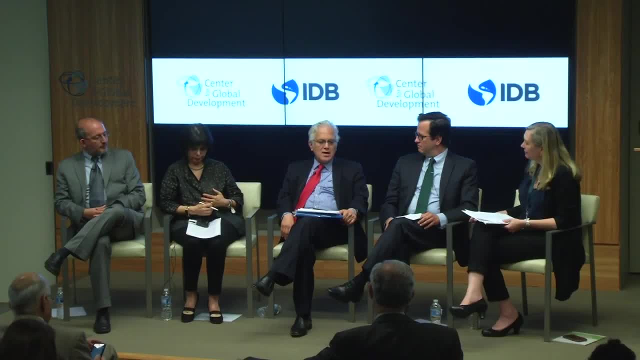 In both cases the statisticians were not doing what they should have been doing because of political influence. And so I completely agree with the postulates in the book that professional independence is essential, But professional independence has to be framed in the broader context of you know. 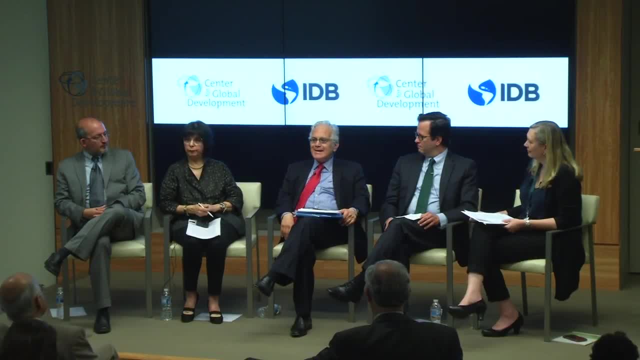 the politics and the culture of society. You know, in the case of Argentina, it was not, or even today it's not, an independent agency, and we know what happened In the case of Greece. it was a prerequisite for accession to the EU. 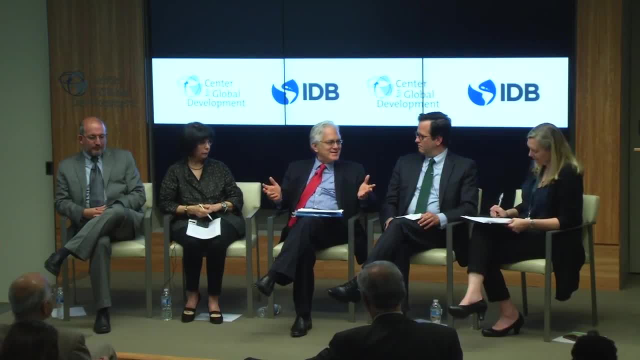 to have an independent statistical office. But in both cases, regardless of the independence of the agency, the statisticians did not do the job they were supposed to do. I mean, I'm not talking about the technical people, but the agencies as a whole. 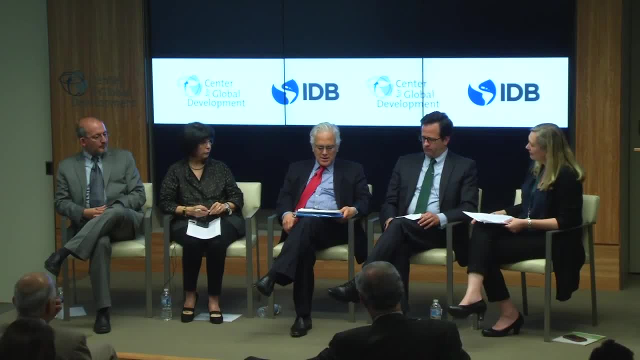 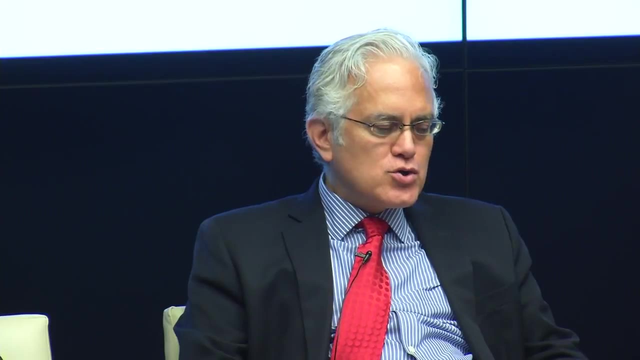 So what is the role of the international institutions? Well, apart from continuing to provide capacity development in the case of the IMF, I have to say that we played an important role in the case of Argentina. We censured Argentina, And also in the case of Greece. it was a key element of the program. 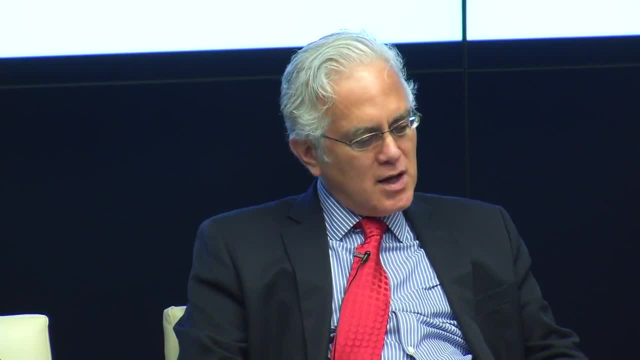 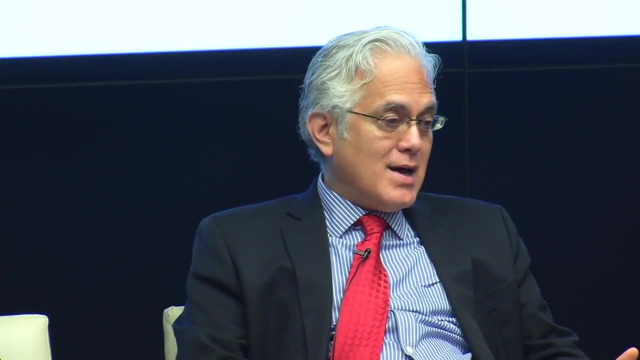 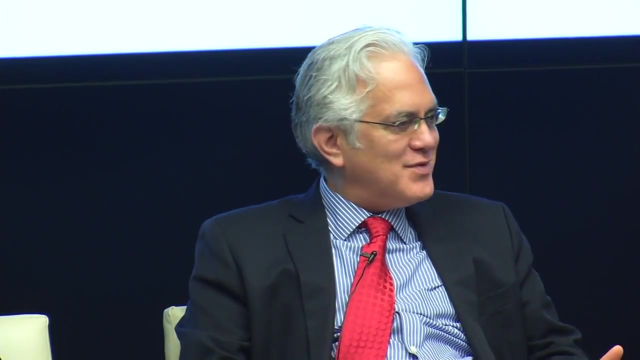 whereby we, together with the Europeans, gave resources to the government to eliminate this political interference, Even though that is in the program. you know, we were not totally sufficient in changing the minds of the politicians, particularly because the new head of the statistical office continued to be. 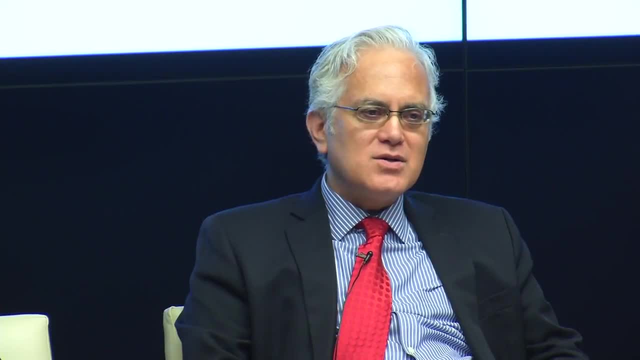 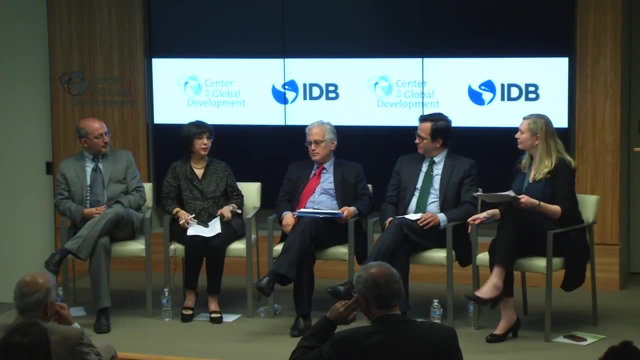 and even still today, is fighting accusations that, in our view, are not well-founded. Can I add something? Yes, go ahead. Just adding something. Going back to what you just mentioned, I think the international organizations have a very complex but very important role in this ecosystem right now. 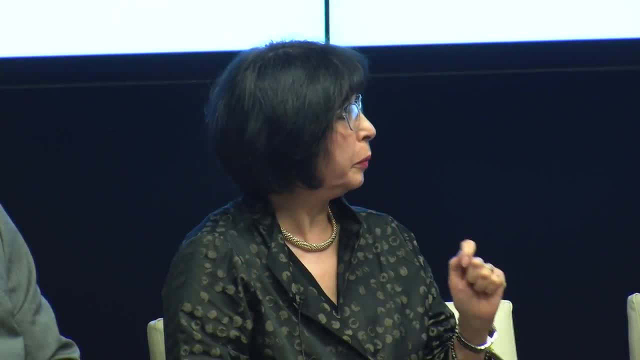 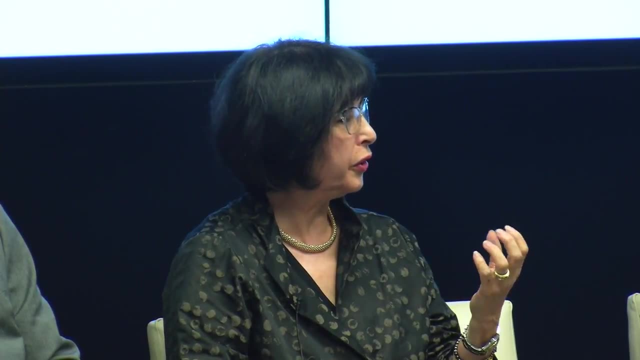 And for me, first and foremost, is for them to be very good, responsible users of data. A lot of organizations that we from the CSO side, we monitor usage, the usage you know, and it's not really obvious whether some of the policies that are being made. 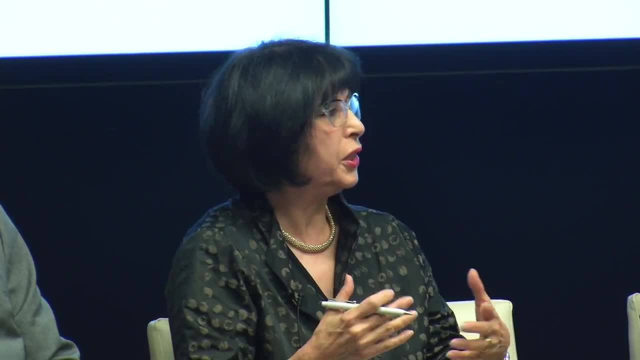 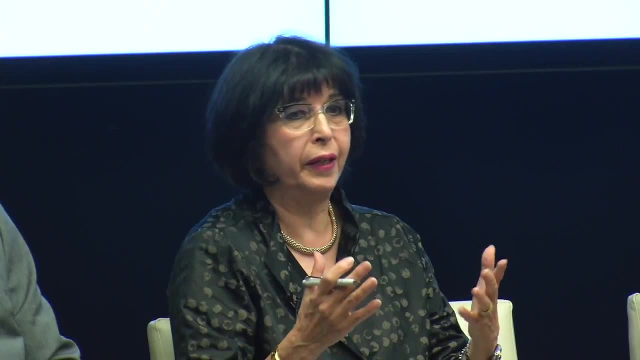 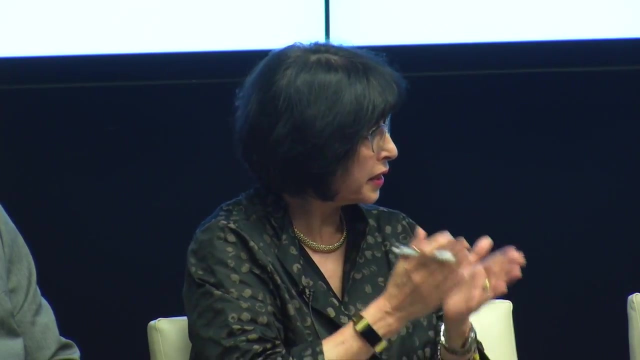 or decisions being made is based on what information and making that information also available and open and accessible. So that's being responsible users, I think goes a long way. The other thing is that more and more we see that the private sector taking data really seriously as a sector in their you know. 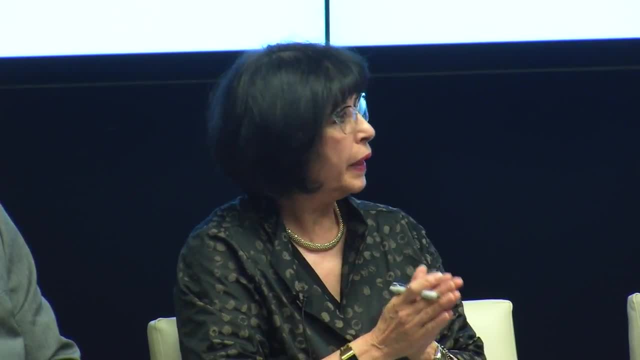 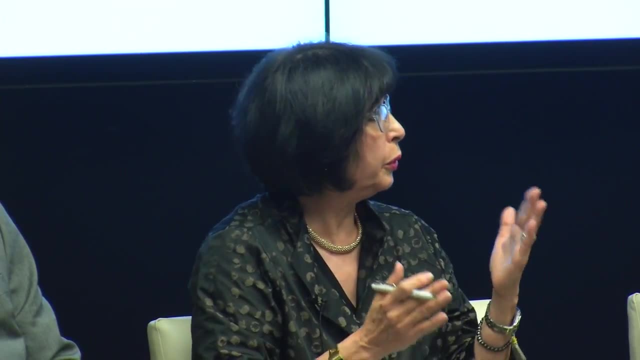 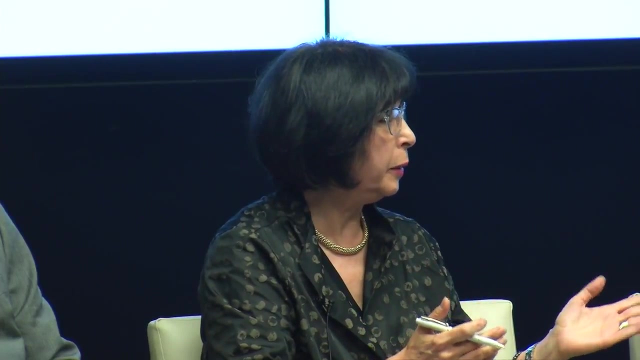 you know best, But international organizations have not yet taken development data as a serious sector in their work. We don't even trace it. It's not even a marker for the data, For statistics and data Hardly any of, except for IMF maybe. 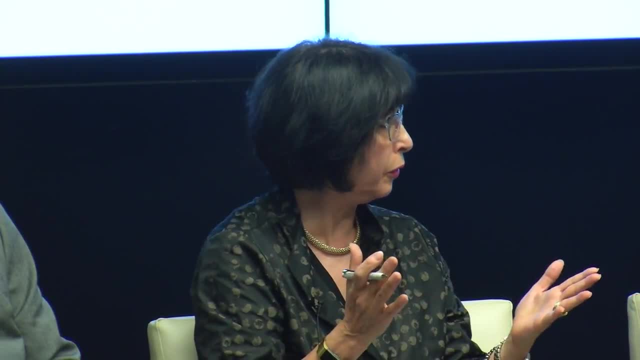 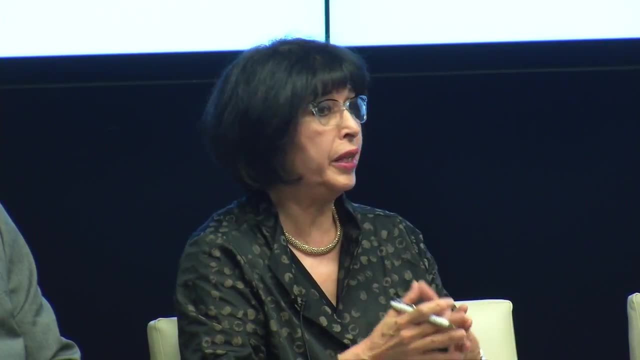 any other organizations talk about data at the board level at you know sort of a strategy for data. So data is still sort of a backroom kind of operation. So development data needs to come to forefront and needs to be part of the strategic decision making. 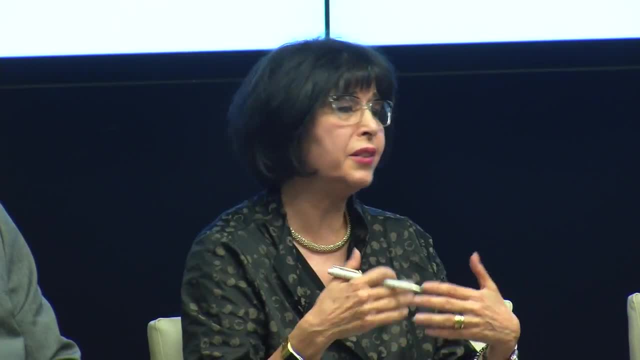 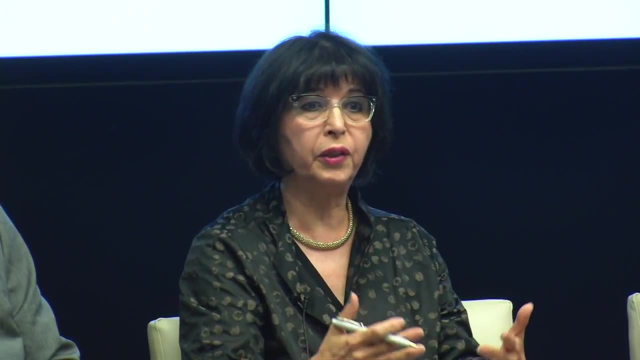 of the organizations. And finally, it has to be part of the discussions with the countries. IMF does that. from time to time, IMF in their dialogue with countries, data is brought up. But you know, I was at the World Bank for 36 years. 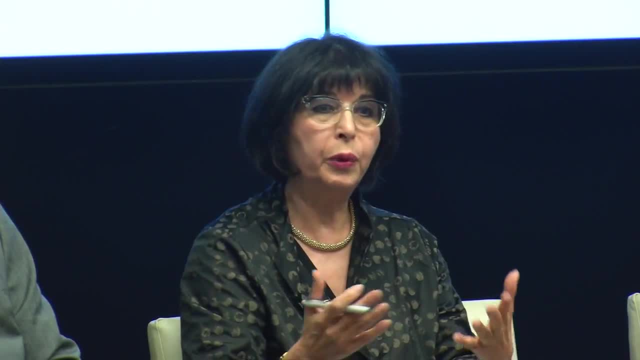 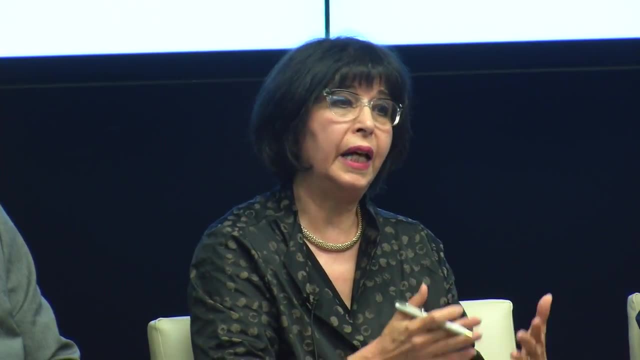 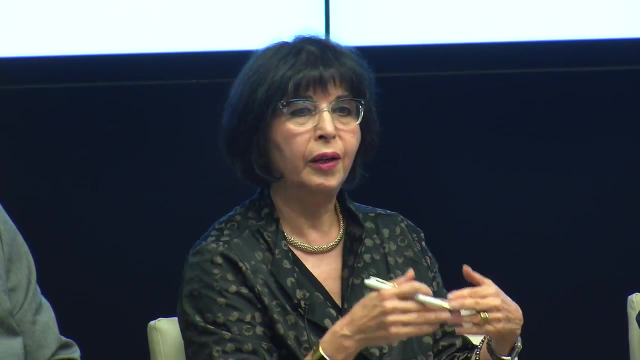 It's not really discussed very seriously with the country operations And built part of the capacity building. I must say at the end of the day the five key donors for statistics do try to bring data into their operations work And you know, some of you know that the top donors of course change. 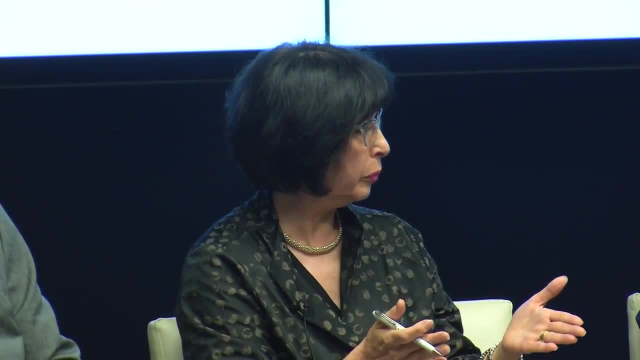 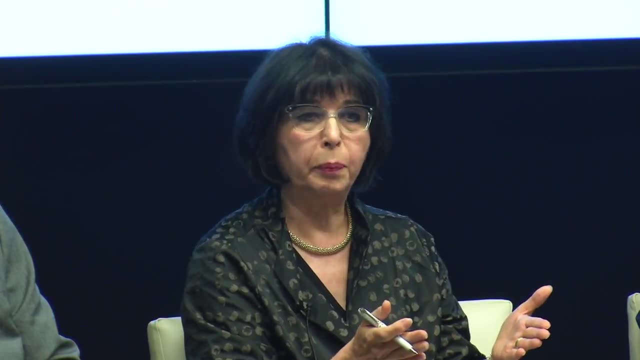 Right now they are the World Bank, European Commission and Eurostat, UNFPA, Canada and African Development Bank. You know some of us are surprised not to see the UK in that list. They were there, but it's just been shifting. 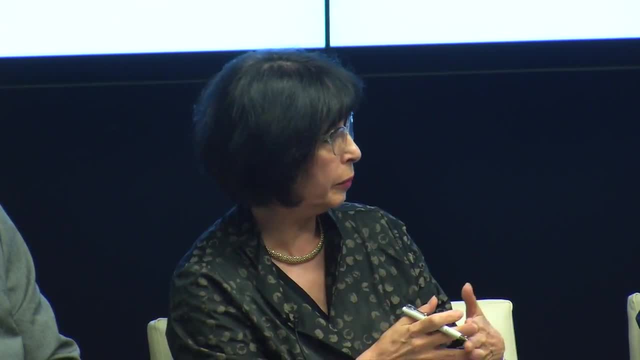 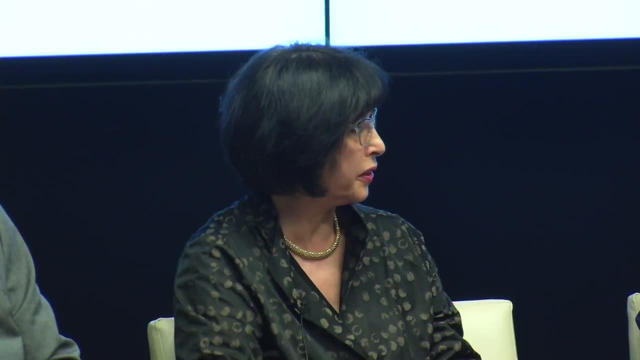 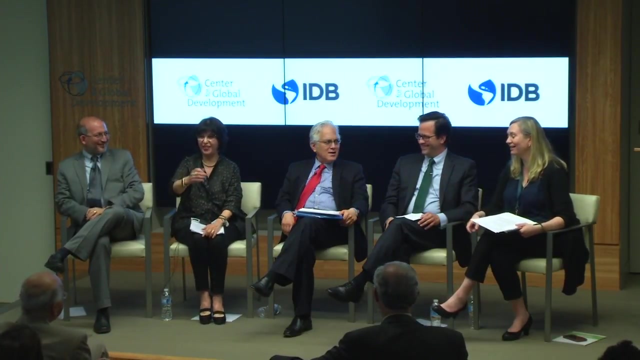 So there are, you know, efforts to increase the resources, But we have a long way to go for data to become part of the DNA of these organizations. Can I just compliment that Because Masoud is here? You know, a few years ago I was working at the MF. 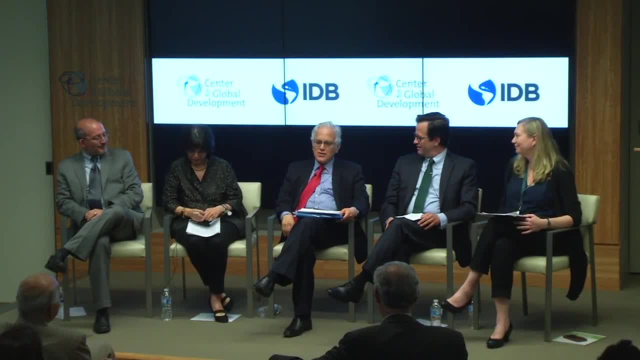 as head of the Technical Assistance Office, And we invited Masoud to deliver some remarks to donors. I am pleased to report to you, Masoud, that donors have been very good at providing resources, including for statistical development, So we do that. 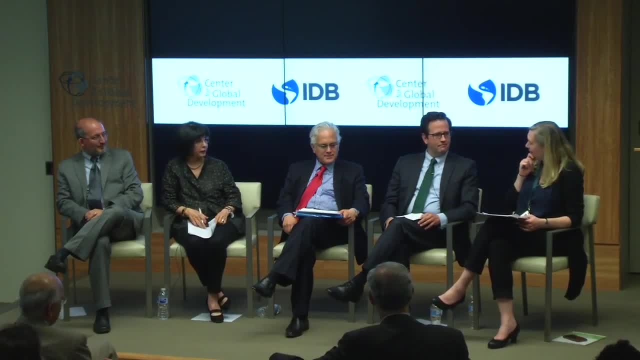 And so we've gotten this issue of resources. since the conversation has gone in this direction, Do you think that the amount of money that we are investing in good data systems right now, how does that fit with the value of data as we know it for policy and things like that? 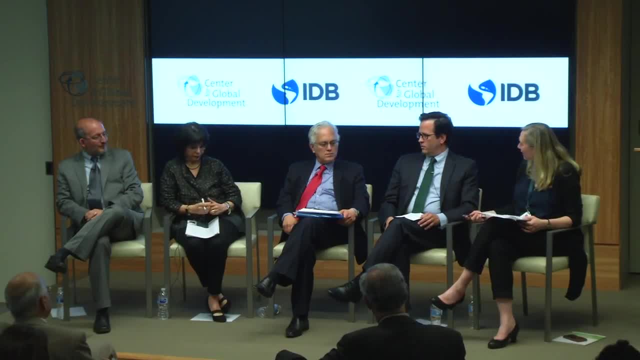 Do you have any responses to the comments that have just been made? I would just add, and I think I'll ask the practitioners to tackle this, but you know, one of the things that this book does is point out that there are a lot of ways that international organizations 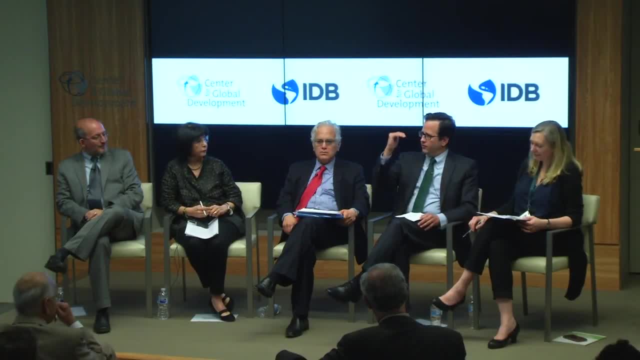 can contribute here And if you think about it in terms of a hierarchy of needs, resources is the first need. Santiago said: maybe we don't need as many resources. The case studies in this book are really remarkable. There are 10 different country case studies. 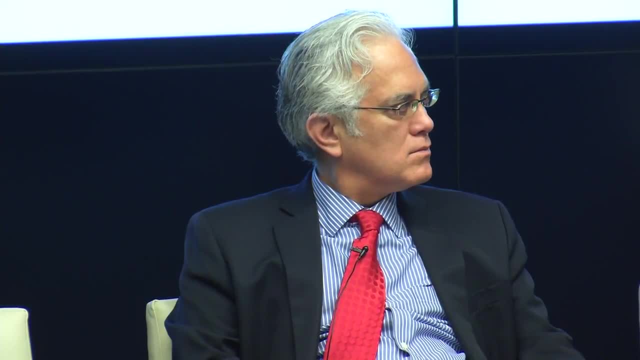 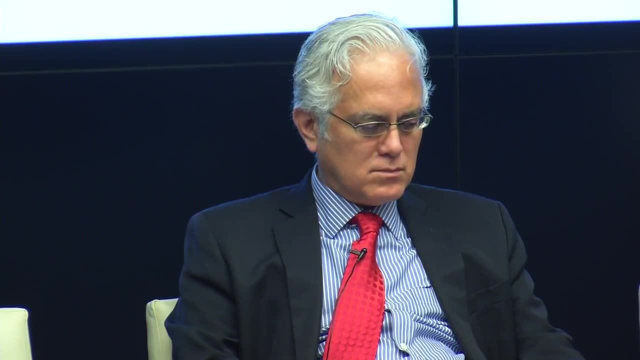 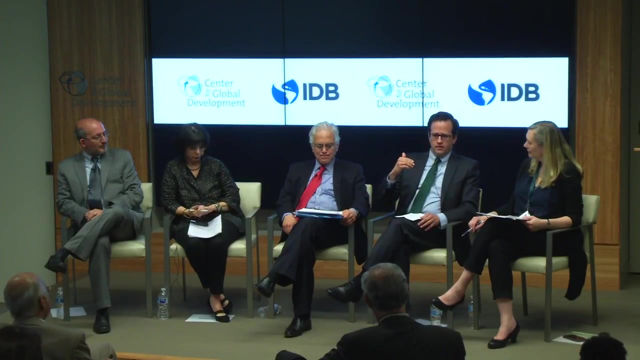 And they do suggest that for some of the smaller and poorer countries, resources are an issue. Then you move up, I think, to the second level, which is knowledge and training, which international organizations can contribute significantly to providing that, And then, third, and this is where I think, for the middle income countries. 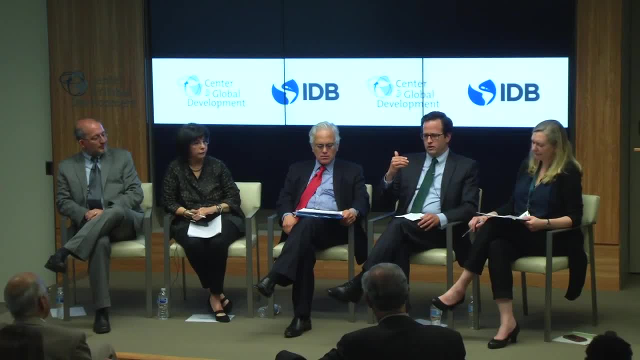 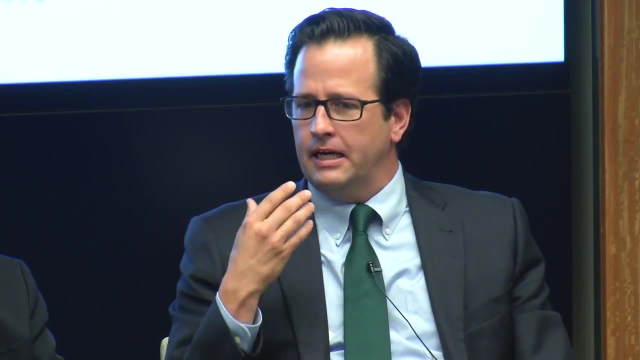 in the hemisphere. perhaps international organizations can play the biggest role. and that is the legitimacy, the legitimizing data, providing some idea of what the need is here for data. I use the term proselytizing. Maybe that's not a good term, but I do think you know. 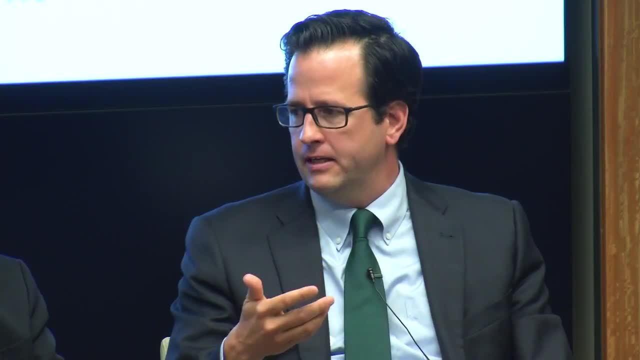 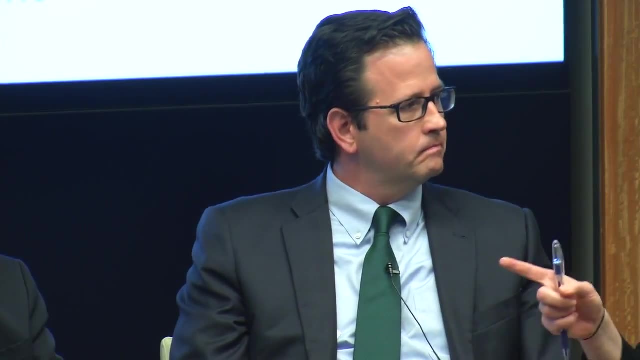 showing domestic audiences why they should care about having an independent, or at least autonomous, national data, And I think that's a good term for the statistical office. So maybe, Pepe, we'll turn back to you now. We talked about money, but what about the capacity building itself? 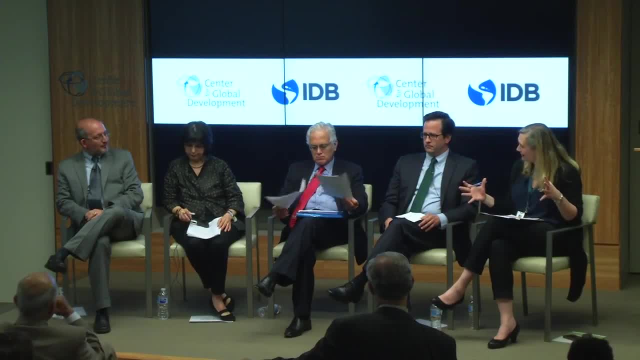 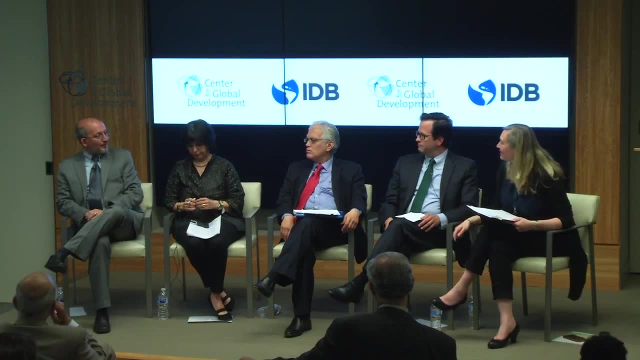 What does good capacity look like? How did the countries do vis-a-vis one another? What are the factors that you think drive capacity beyond? well, in addition to the things that you were discussing as part of your presentation, Well, you know one of the things that the 10 case studies show. 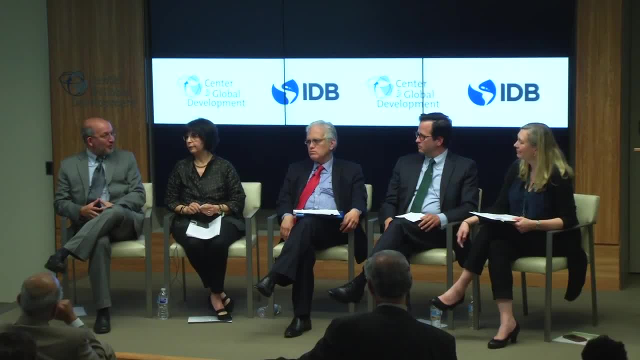 is the importance of human resources In these institutions. the level of specialization that these institutions need implies that the human resources are very highly trained and that training a lot of time is relied on two things: on experience and on the training provided by international organizations or peers. 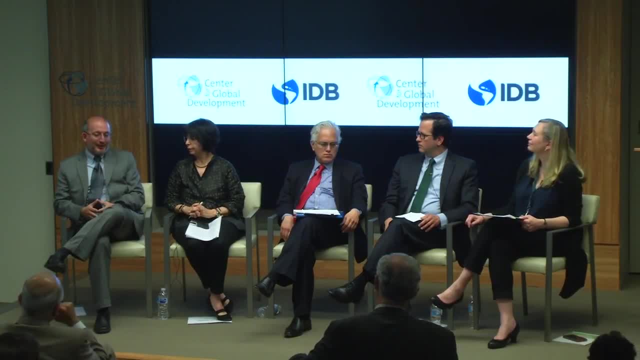 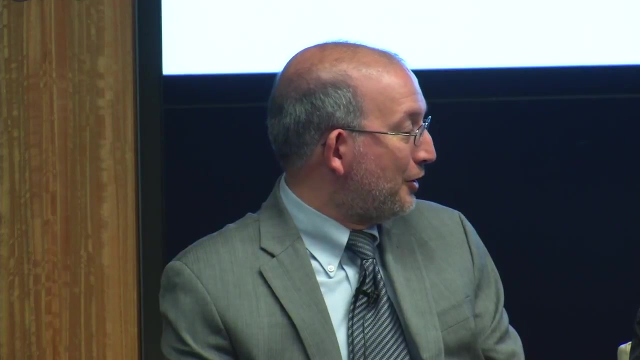 There's a lot of south-to-south cooperation. So in that sense, you know, capacity can be seen through the eye of their human resources. Then it comes, you know, an issue of the investment in technology, And we need to be up-to-date in the use of advanced information technology. 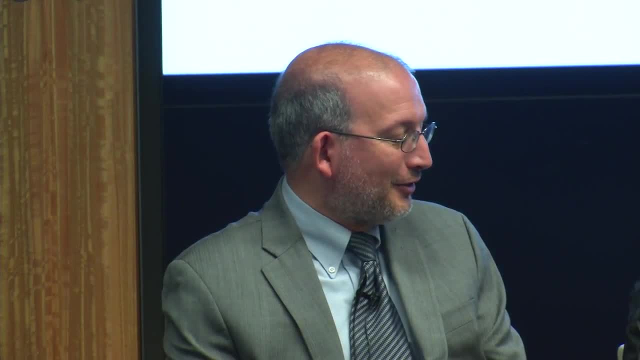 And we have seen it, you know, in one of the case studies mentions. you know the statistical offices were one of the first institutions to use computers in, you know, in the early ages. And in many cases you know we see two countries in Latin America. 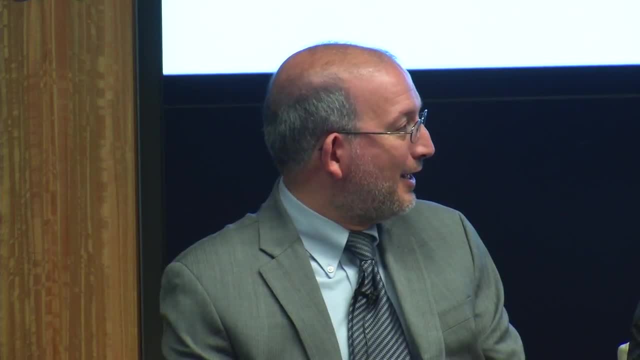 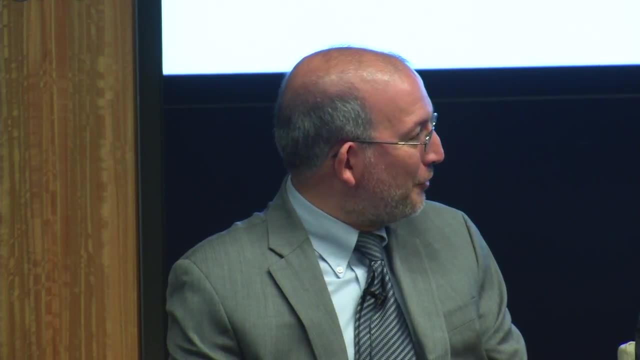 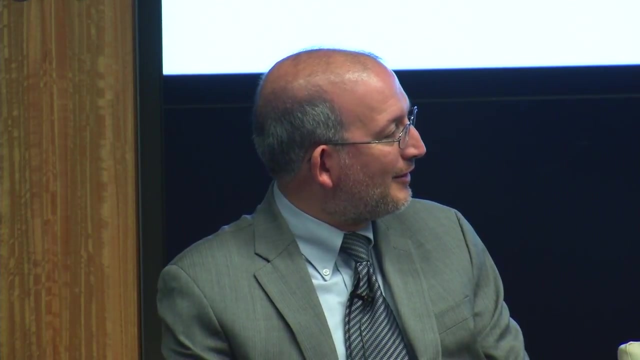 that have an eye in their statistical office because they were. one of the responsibilities was to guide information technology policy in the country You know, such was their advance on the use of computers and such that they had to provide assistance in that. Which country is the most advanced technologically right now. 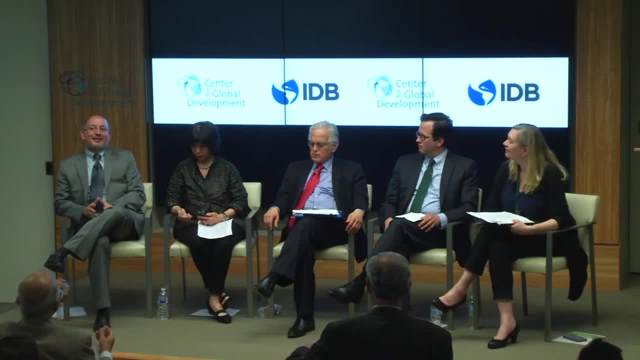 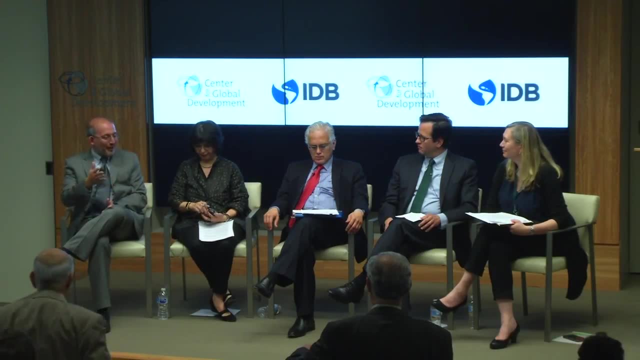 Can you give us an example of what that looks like? Well, you know the two clear leaders in the region and they have proven it. you know Cheida and Roberto. you know they have been to the Statistical Commission of the United Nations. 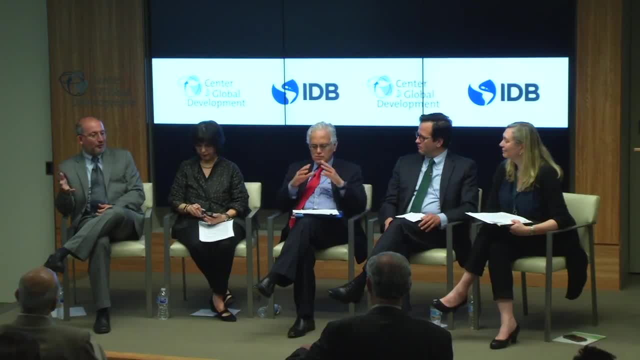 They are leaders, not only in the region but across the globe are Brazil and Mexico. But there's also, you know, this leadership not only shows in a slow movement, but also there's leadership in having, you know, in pioneering, Because Colombia has been pushing for you know. 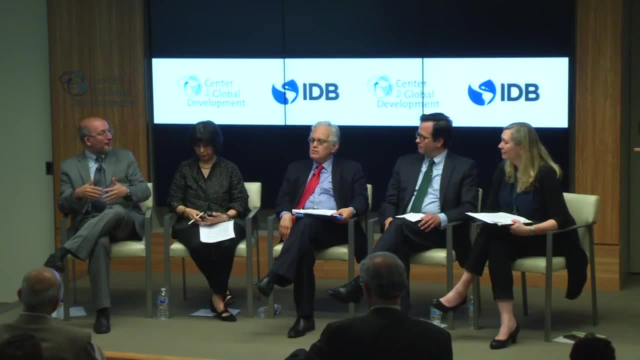 to be a leader in the use of technology. You know, in 2005, Colombia was the first country, probably one of the first in the world, to use PDAs at that moment, you know- to capture data for their censuses. 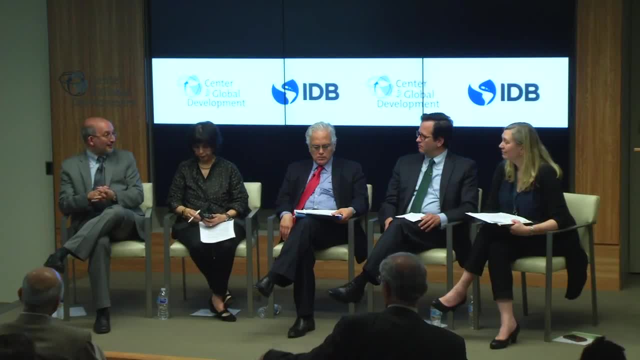 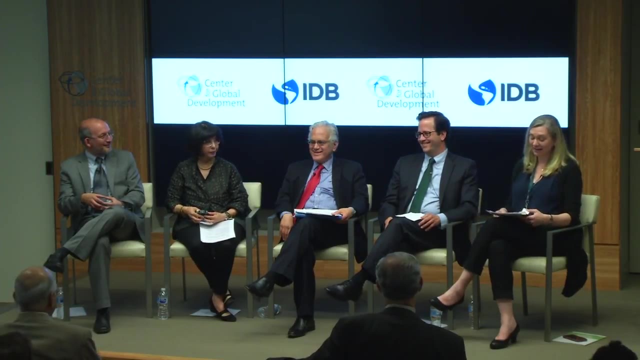 And now they are actually using internet-based census data entry. for you know, experimenting, But at some point somebody has to make these experiments in order for others to learn. Yes, Not win its World Cup match today, but they are winning on statistics, which is good. 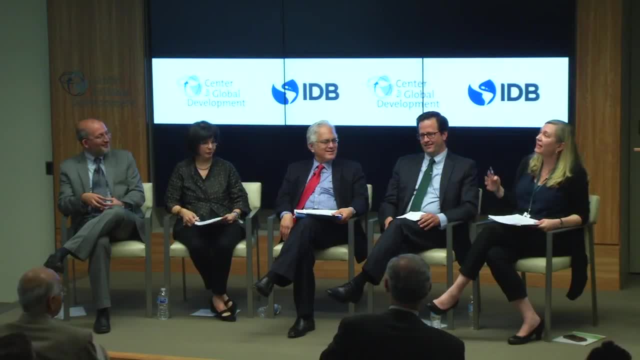 Although let me ask you this about one of the things in Latin America that has happened frequently is a lot of investment in a census, for example, And then the political authorities, whether it be Congress or other, not willing to use the results of that census to allocate resources. 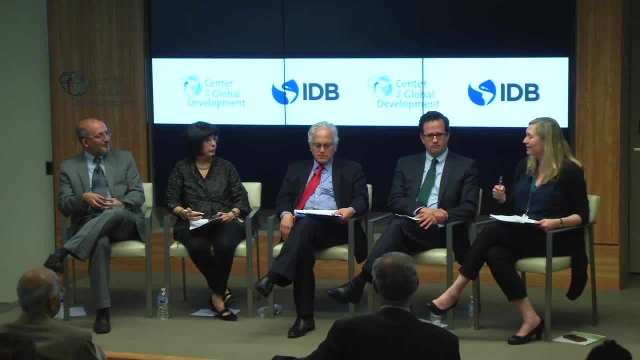 for example among states or voting districts, And that's obviously not a problem that is only in Latin America but in other parts of the world, including places where we sit today. Can you say something a little about that? You know that comes to mind when you think about a political economy consideration. 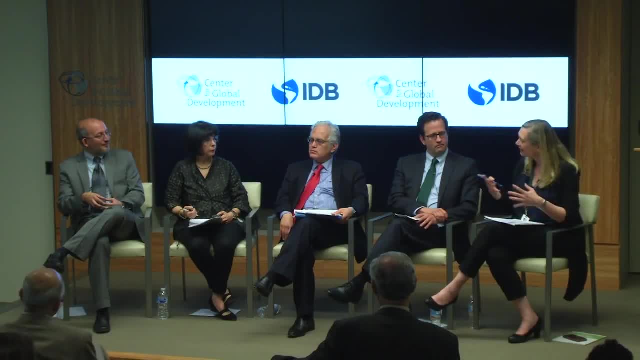 Is that a capacity problem? Is it a political? you know how do you see that issue through the lens of the case studies that you've done. Well, I think you know one of the questions that is on the table and you know not only from this research but from before. 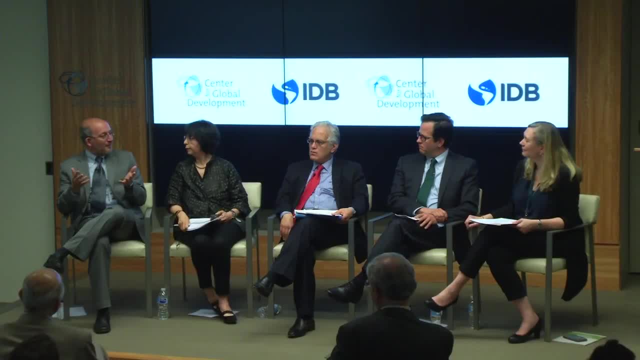 is. you know- and it's a discussion that at least we had at the IDB about 20 years ago, when the IDB started financing, or giving loans to finance, censuses- is this an expenditure or an investment? So we had to argue that this was an investment. 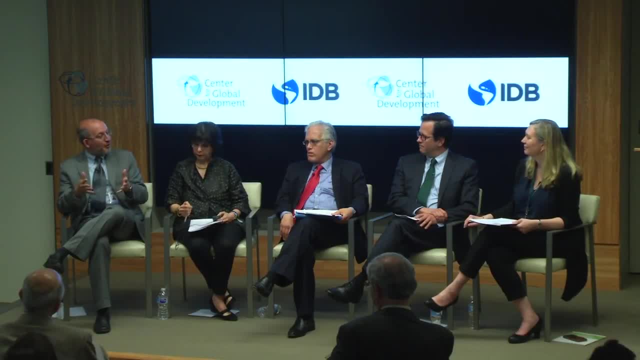 that, just like you spend on a road network, you need to spend on an infrastructure of data for policymaking, to make decisions. But now that we have, you know, argued that it is an investment, the next question that is on the table is: what is the value? 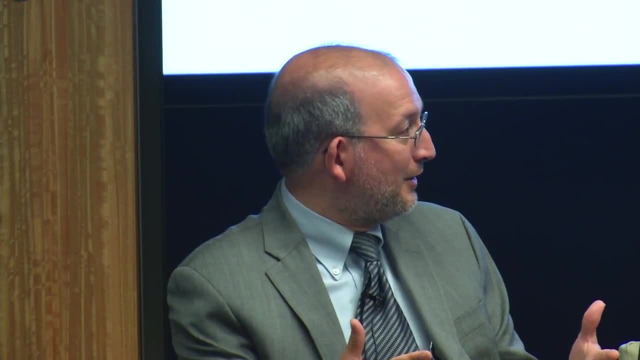 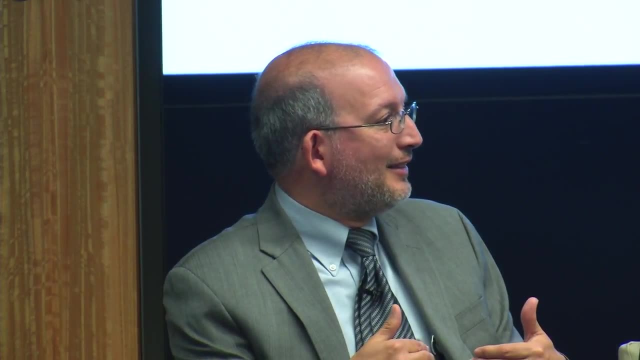 What is the return of that investment? And, of course, the return of that investment is linked to the usage of the data And I think, in that sense, you know, that is something that the book points out, and it's this promotion on the use of data. 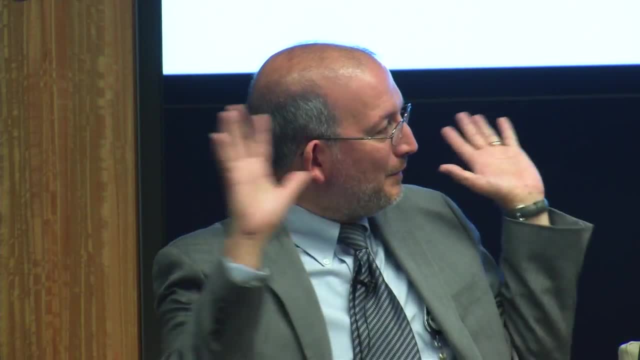 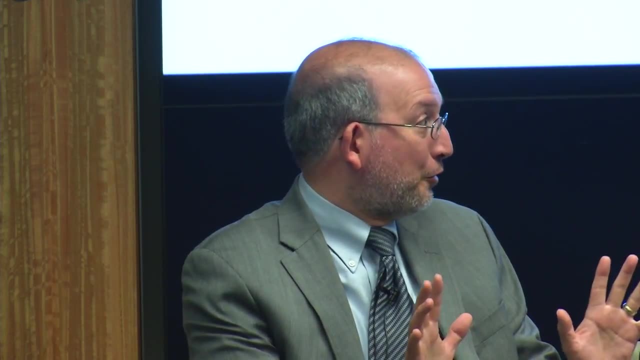 You know, sometimes the statistical offices say, okay, you know, here's the data, my job is done. I think you know there is more need and I think you know the statistical offices need the support from international organizations. 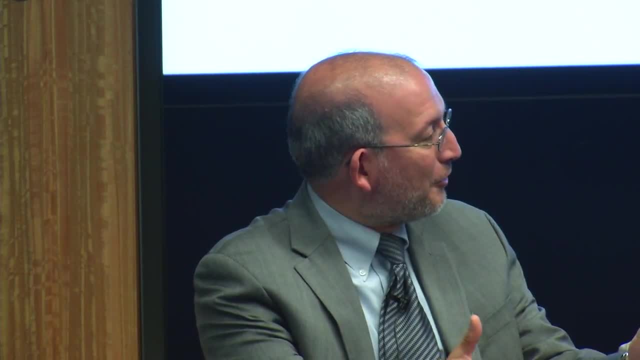 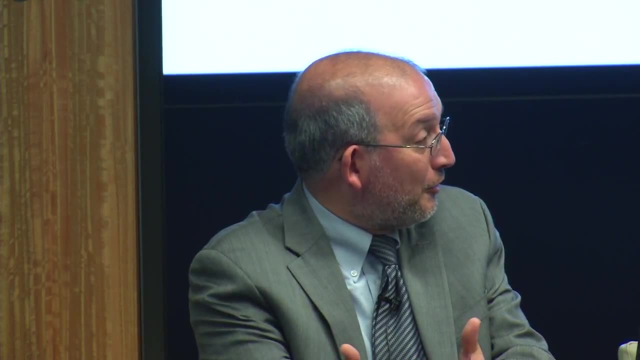 Okay, okay, look. you know you are allocating resources. you know, based on data from 15 years ago, the inequity, the inefficiency of that, and you know you need to do another census or you know to use more recent information. 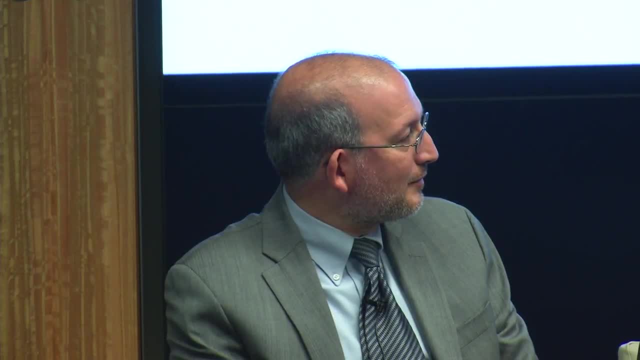 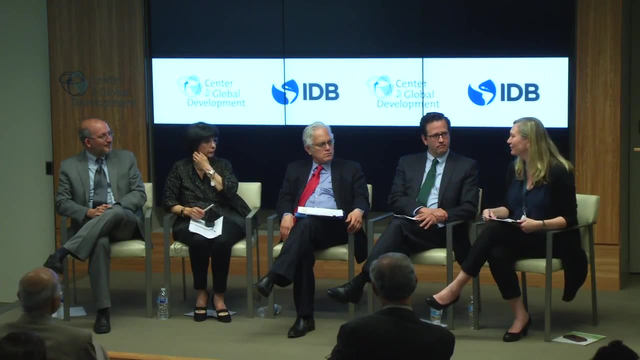 to make that allocation, But I don't know. it just always made me mad. Yes, We would spend $40 million on a lending project and then not to see that used for resource allocation. Shaina, you talked a little bit about that. 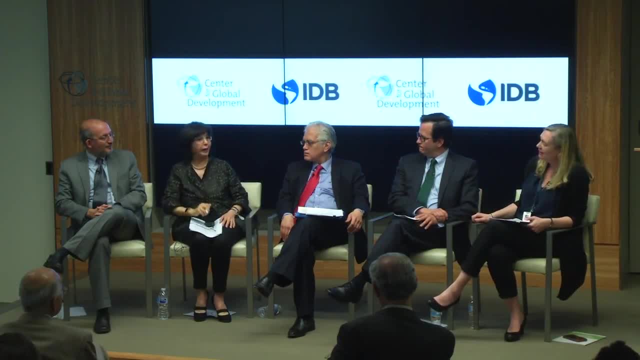 and also the civil society perspective on this Right. I think what that's really. that breaks my heart, too, and that's why I'm doing the work that I'm doing right now, because we're finding out more and more that, with all the value, 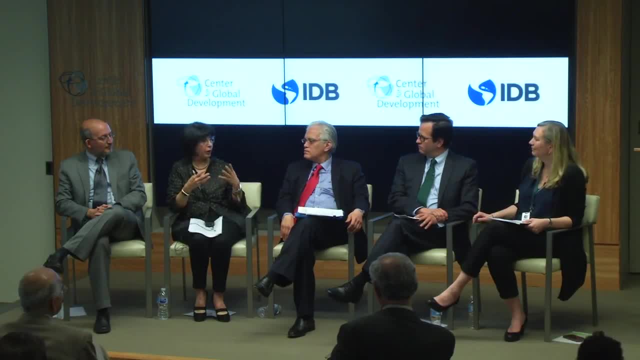 all the investments in data. they're locked up. You know, locked up doesn't mean that they just need to make data available through PDF and then they've done the job. It's really, for data to become valuable and used, you have to walk it to the users. 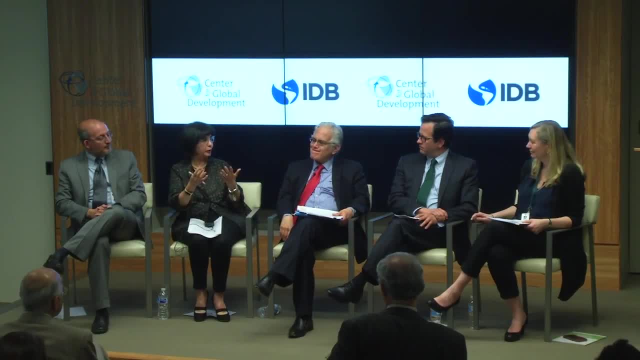 You know you have to have make the data accessible. they have visualization. there would be terms of use so the users know how to use it, what's their right and so on. What's the privacy issues? So data production doesn't end when you have the data. 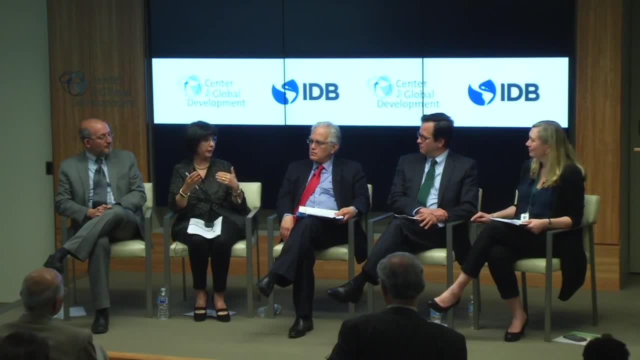 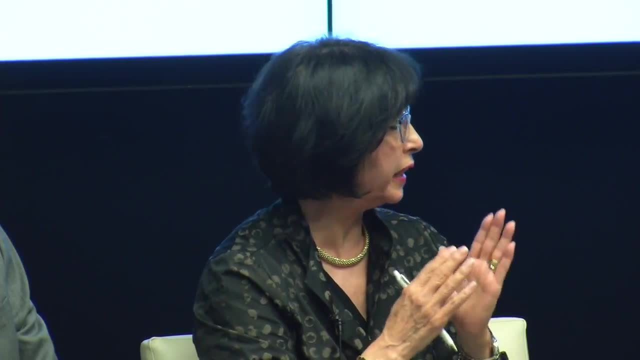 You really have to go further steps to get the data ready. And that's one of the things that in the old model of capacity building, a lot of us did not pay as much attention to. We were so much we said: build it, they will come. 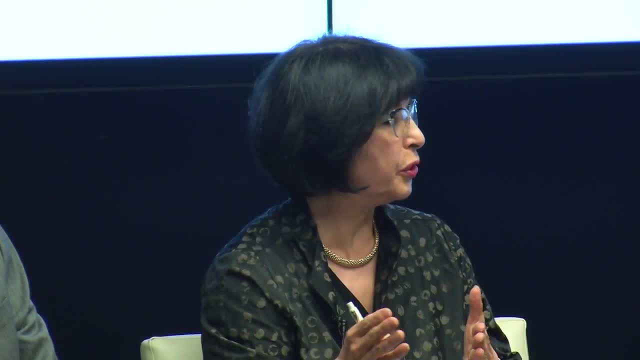 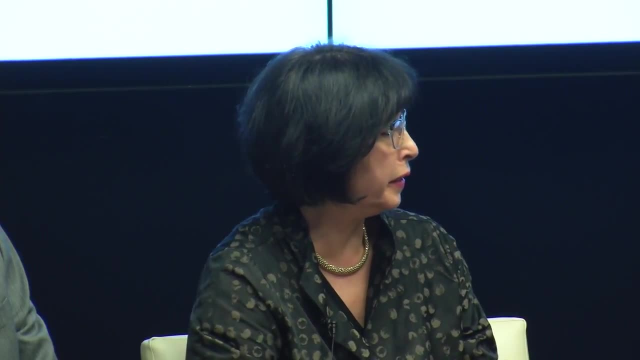 And it doesn't happen. You know, you really have to do much more. So that's one of the learnings that also the book confirms that we need to take to this new capacity development approach. Yeah, Roberto, speaking of making data available. 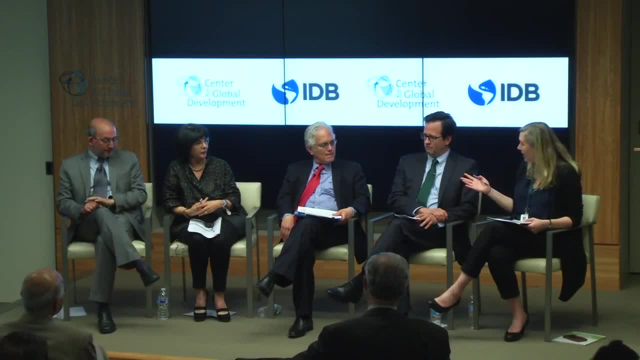 I think was it a year or more ago that you came and talked about the requirement as part of some of IMF programs to make the data open. in addition to following the standard, Do you want to talk about progress so far and any effects you've seen of that increasing availability? 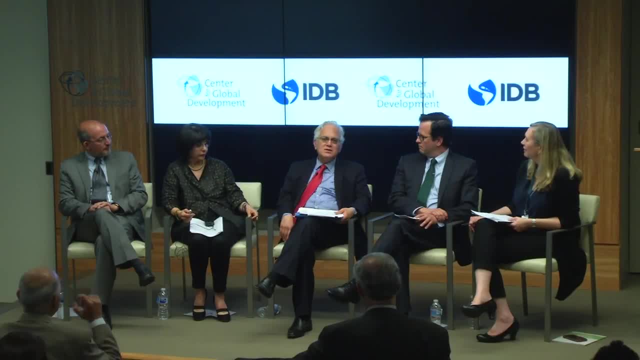 Yeah, So what I referred at that time was the approval in 2015 by the board of a change in one of our standards, the general data dissemination system, which originally, in the late 90s, had been intended to stimulate development, but it had a problem. 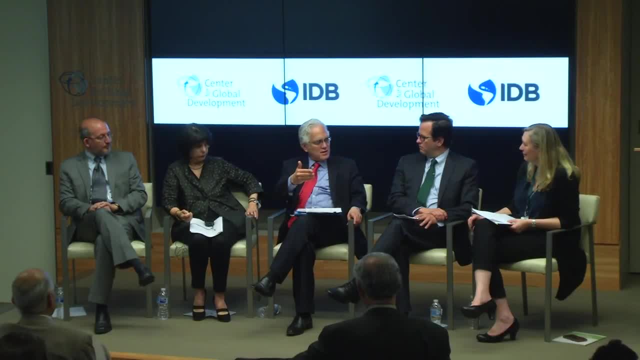 And the problem was that it assumed that once the statistical office developed, they would automatically disseminate the data. That never happened. So since I mean, we're talking about 100 countries that are less statistically advanced, So since then we have been working with authorities. 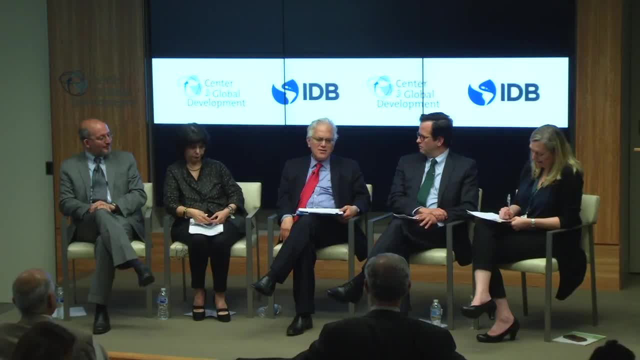 of at least 40 countries now, and mostly in Africa, but also in the Middle East. We partnered with Jose Antonio in the case of Paraguay to make sure that authorities can publish in a website first what we think is the data that are essential for policy making. 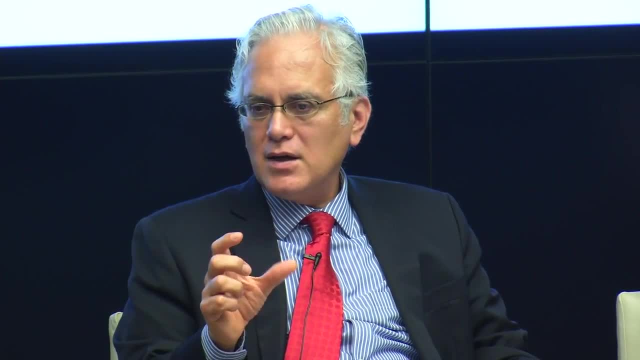 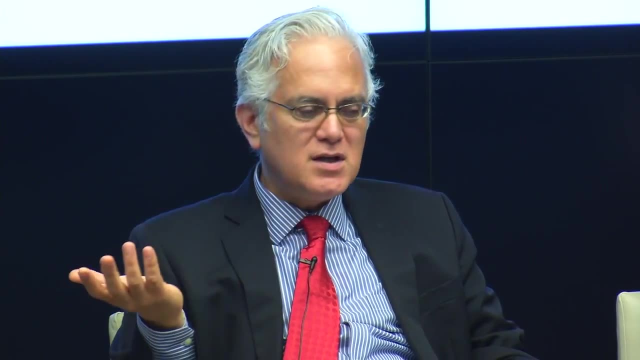 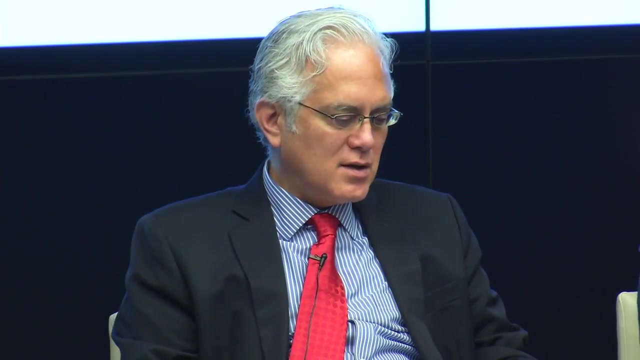 but also to allow the authorities a platform to publish other data that they might believe is important, For example, data that might be needed by the IDB or the SDGs, and so on. That process continues. Recently, in March this year, the board approved a new overarching strategy. 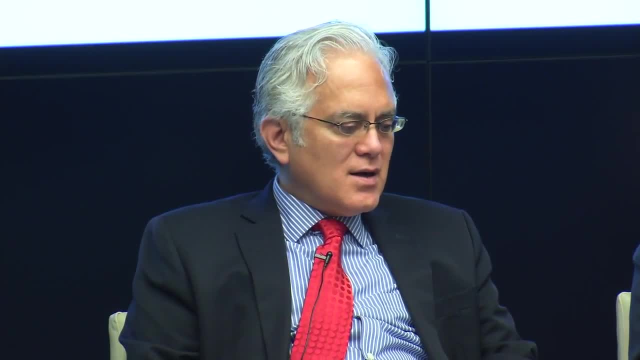 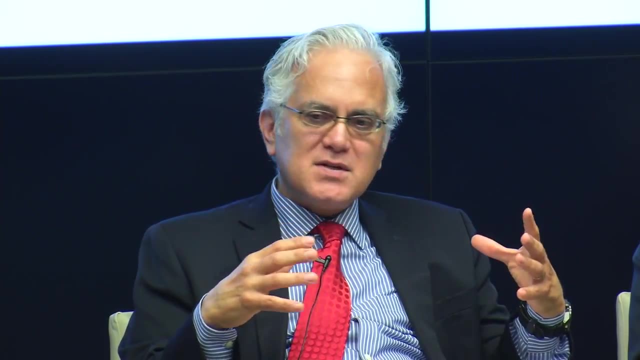 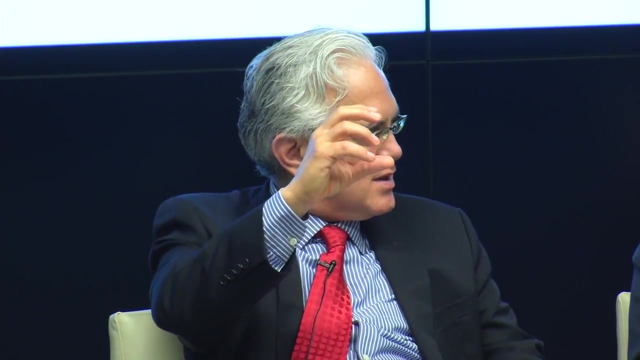 on data and statistics at the fund that has a vision that we call the Global Data Commons, which is essentially, you know, we feel that perhaps in five years we can have a network of what we call the NSDPs, these websites that disseminate data. 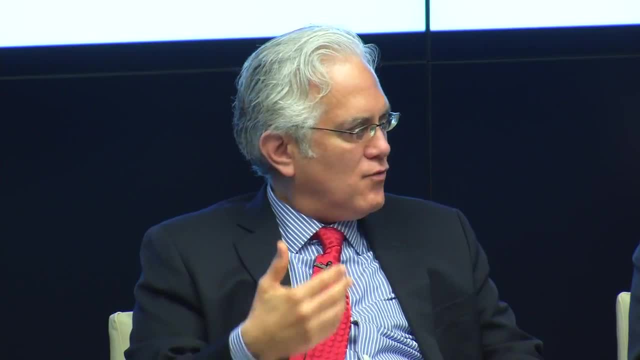 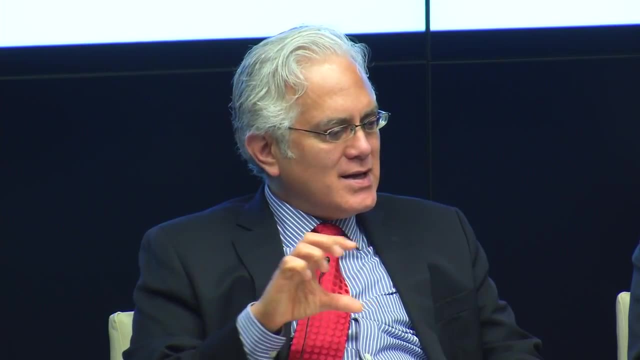 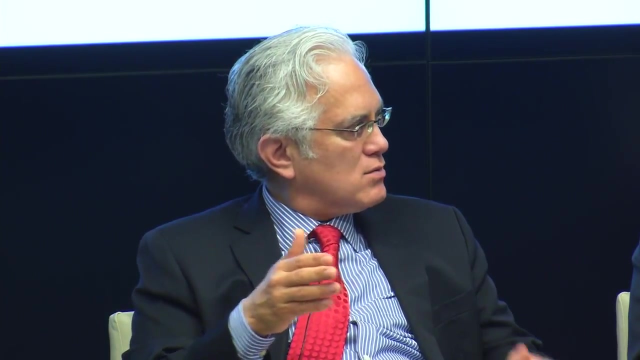 that we feel are necessary for the fund to conduct its business and for others to monitor economic conditions and policies in a disciplined manner, that is, in accordance to agreed decisions about dissemination timeliness and periodicity. We feel that, once the 189 countries of the world 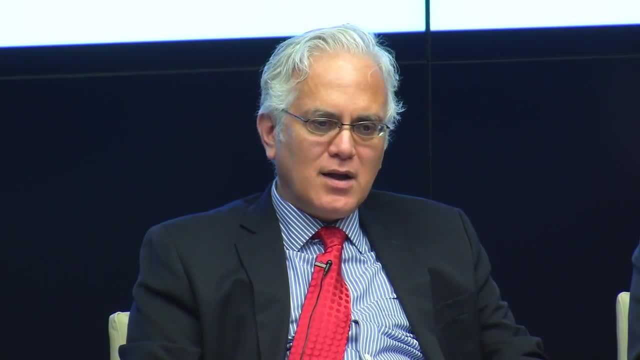 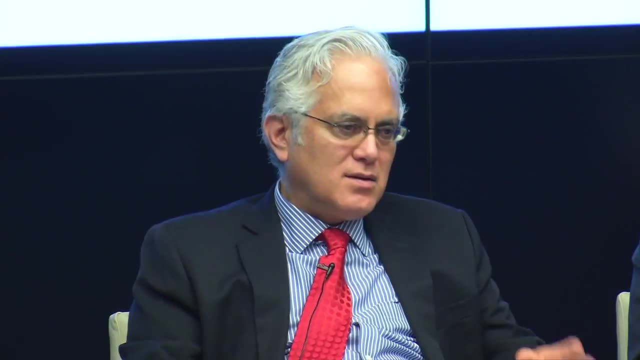 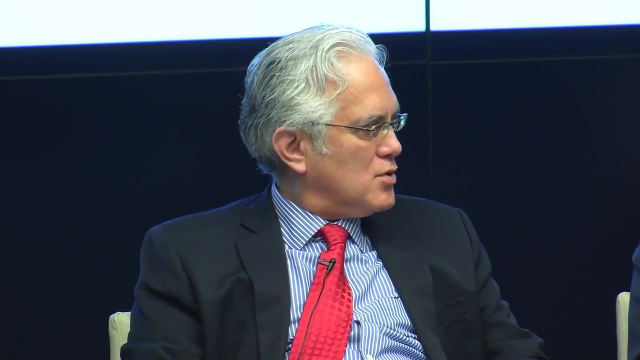 are publishing this data in nearly open release in the same format that will allow not only the local audiences but rating agencies, international banks and so on- everyone to have the best data possible Interesting. So we're about to go to you in the audience. 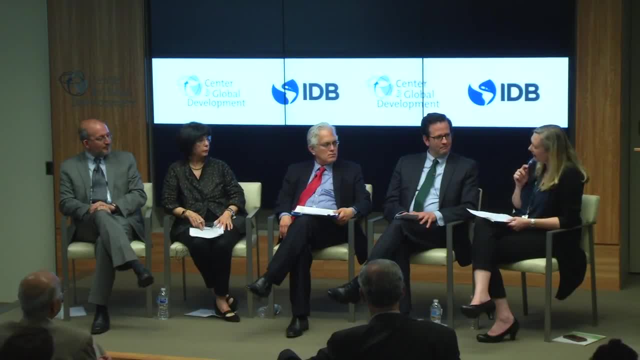 so prepare yourselves. But, Matthew, can you reflect a little bit on you know independently as an academic, I know you're also a contributor to this book, but how well do you think that the international institutions do at acknowledging and managing the political economy? 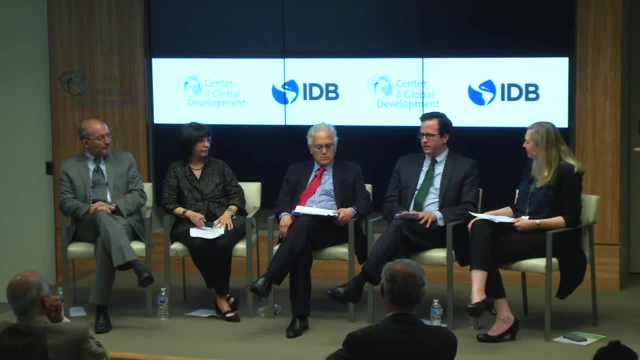 of statistics and statistical capacity building. Well, it's been a real learning experience and I appreciate the opportunity that José Antonio provided to participate in the project. I guess one of the things that I was struck by in this book and I highly recommend that everybody read. 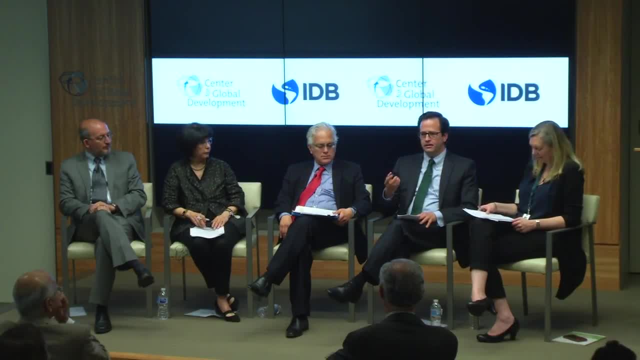 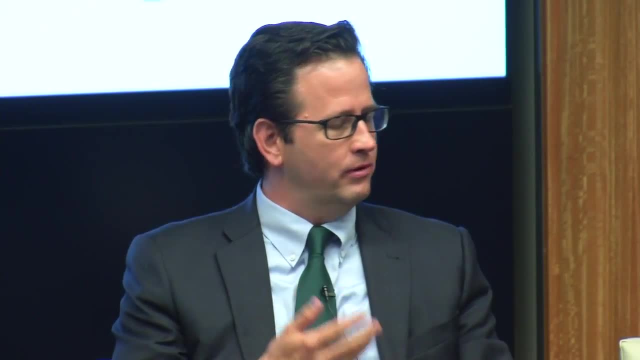 the case studies is that there are 10 case studies here, and that's something that I think only the IDB could do in such a short time period. But what's fascinating is the 10 case studies. they come to completely different conclusions. So 10 countries, 10 problems, And you know, I kind of, in the early stages, imagined that there would be 10 case studies and then we'd have a taxonomy of the problems, And instead of that there's a really 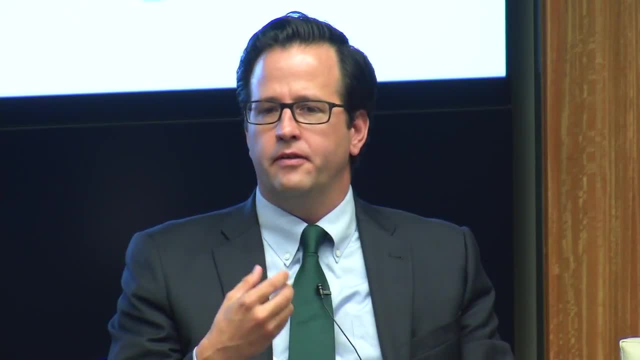 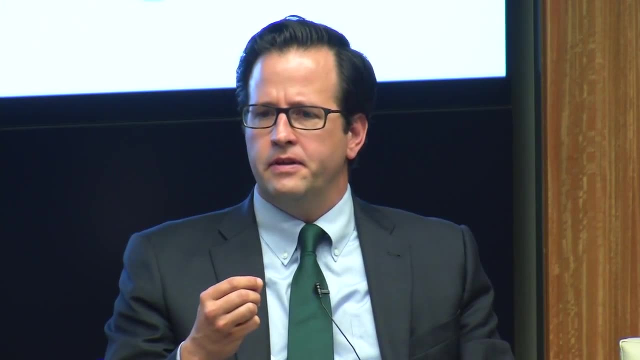 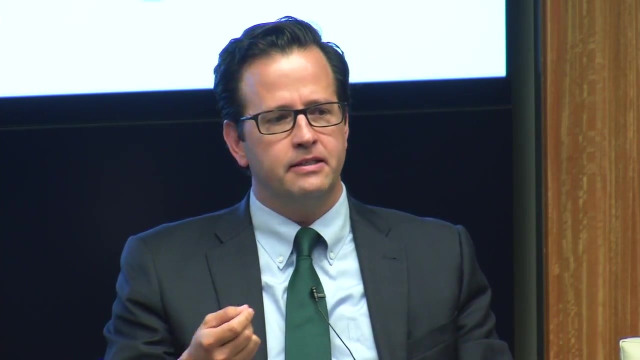 I think that the political economy is so complex that every country is different. One thing that we haven't talked about, though- that came out of the case studies- is the necessity for something that José Antonio mentioned in his talk, which is coordination, And I was struck in some of the case studies. 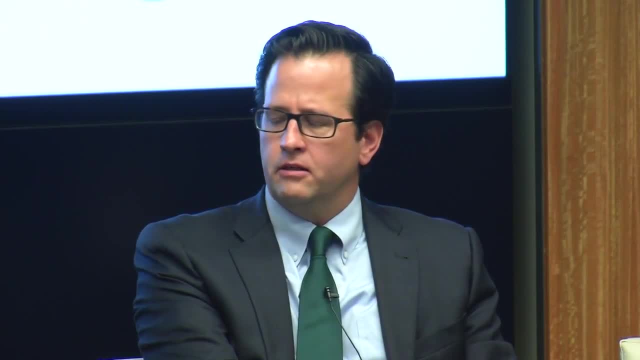 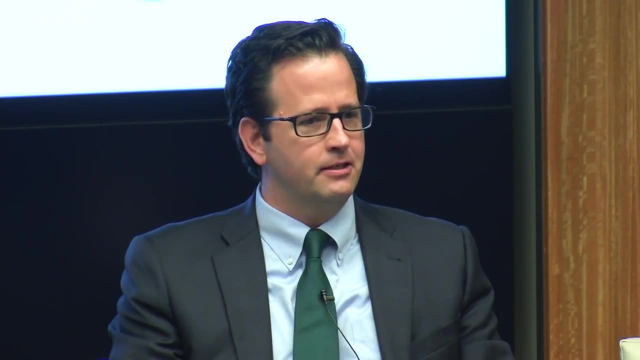 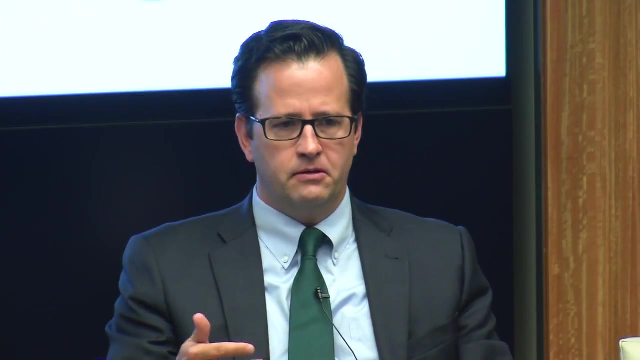 by the fact that, you know, national statistical offices oftentimes are given an impossible task of overseeing the entire national statistical system, And so this gets to issues of state capacity across the whole of government, but it also gets to very complex political issues. 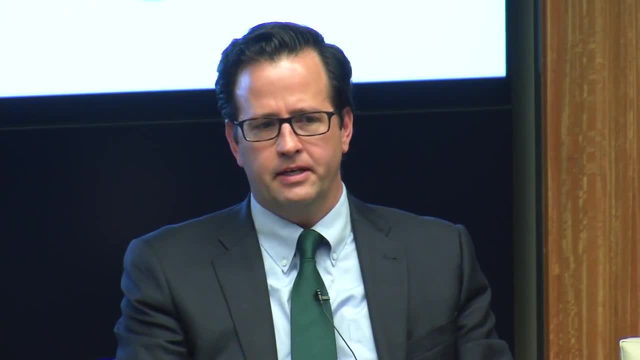 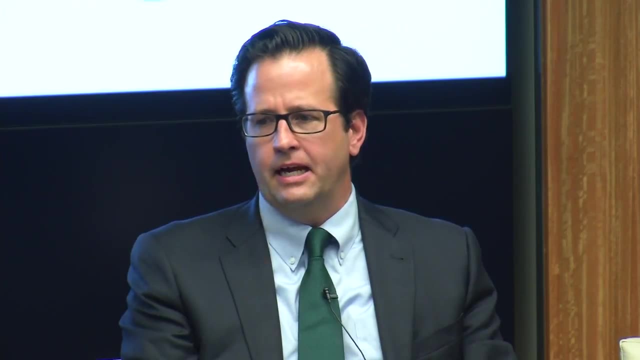 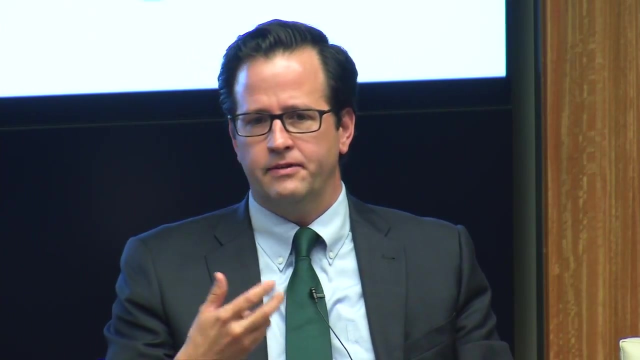 And this is a place where I think that the case studies are very rich and I highly recommend reading about them to see how some countries have dealt with that. Not all countries obviously have been able to deal with them effectively yet, But I think that this is a place. 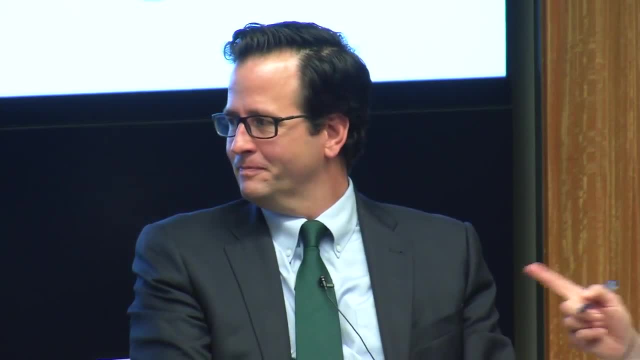 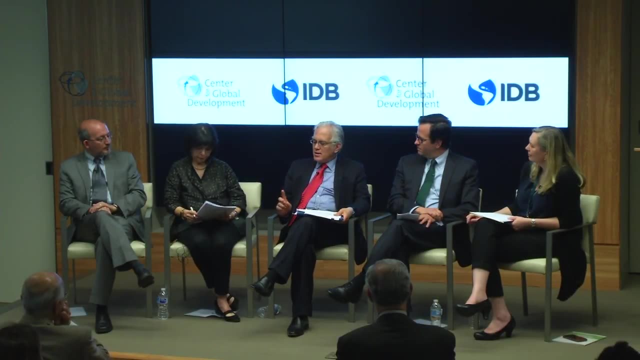 where the comparative learning will be helpful. Can I just say something? Yeah, I totally agree with what you say, But I would add the following: I remember in particular what the book says about some central banks, the Central Bank of Guatemala, and so on and so on. 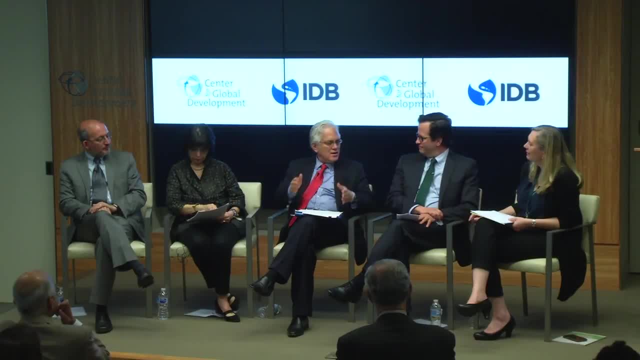 And what you say, the complex politics and perhaps the competition between the several elements of the statistical system. Here I would emphasize the point of finding ways to ensure the statistical office can collaborate effectively with the other institutions of government. This is more difficult than one would expect. 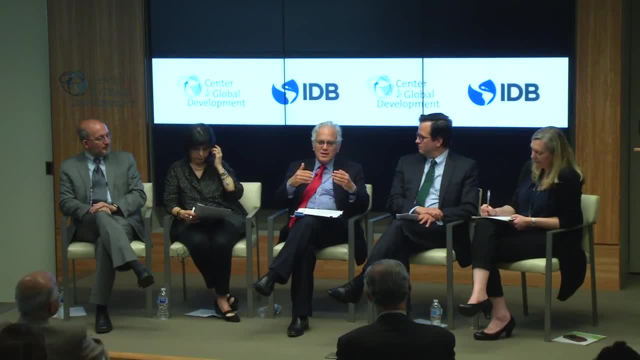 The difficulties have to do with jealousies, political competition, but also, very importantly, with the different relativities across the government, For example, the Central Bank. typically, the Central Bank has a higher level in the hierarchy, better salaries and more resources. 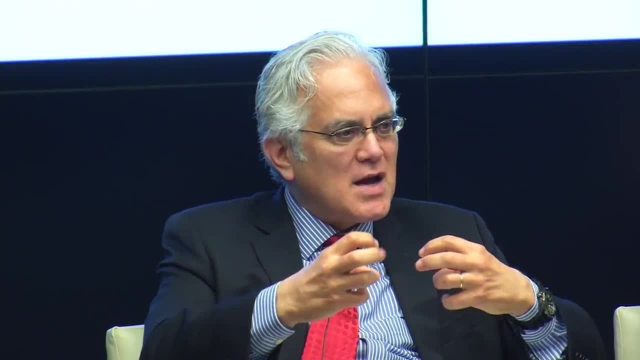 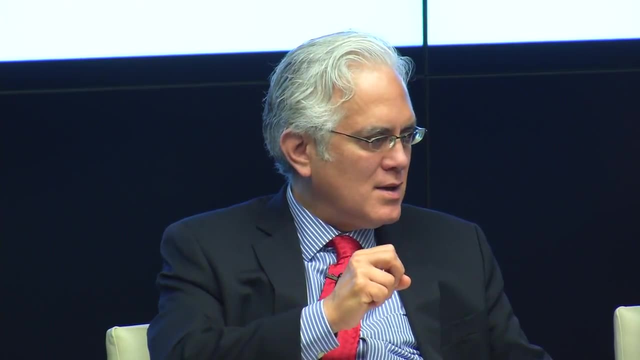 The statistical offices tend to have less, And so there is sometimes some jealousy, some problems that are difficult. What we have found is that, in these situations- formalizing data sharing agreements, ensuring that the statistical office can access, for example, tax information- 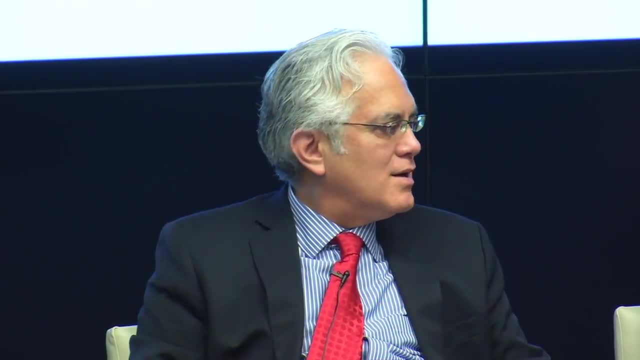 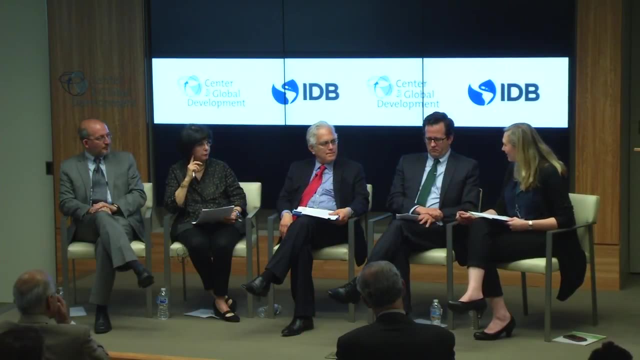 or central bank information is essential. Without that, progress is difficult. Yeah, let's just drill down a second on this issue of independence and the role of the different agencies within government. You know, as your remarks in the book points out, it's actually it's not really clear. 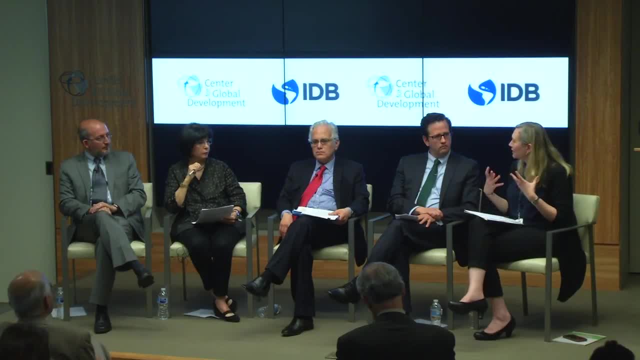 whether independence is a requirement to be able to do better on high-quality statistics or even statistical capacity. On the other hand, it seems essential and helpful in other cases. But you know, I remember when we were working on this data for African Development Report. 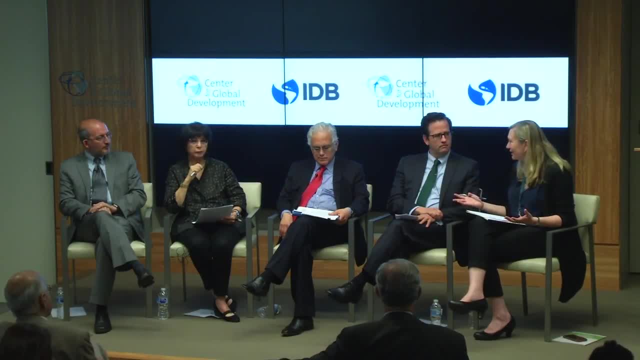 we fantasized about the central bank model for national statistical organizations. Is that feasible, or is it just a fantasy? Obviously, the Mexican case of Inegi is really interesting. The governance arrangements around it are really interesting. Do you want to reflect on that, José Antonio? 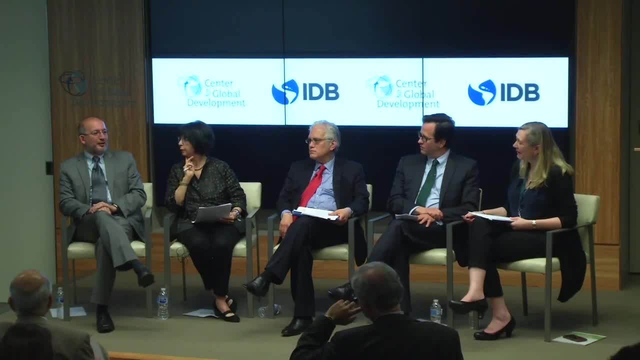 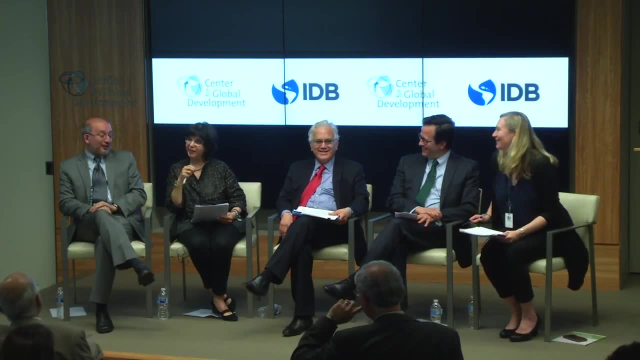 Well, I think you know the model of the central bank is always great, but the thing is that you know they have a printing press And they have money. I know They have their own source of revenue In the basement. 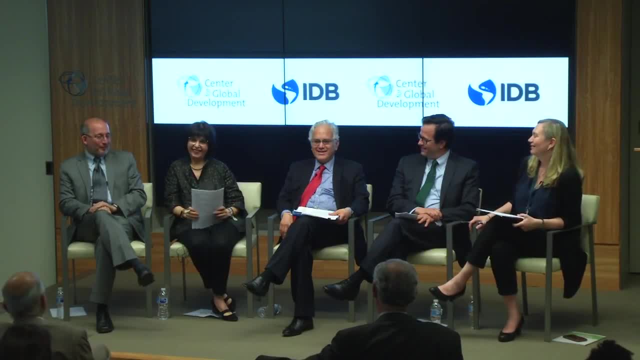 Yeah, yeah, And that does I mean. that makes a big difference. You make a reference to the Mexican case. you know when the new law was discussed. there's only one level of independence that Inegi was not able to achieve. 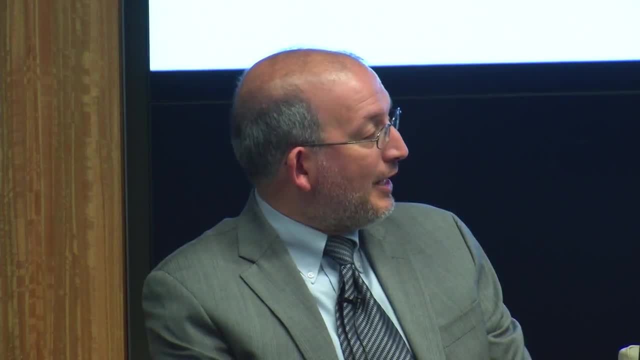 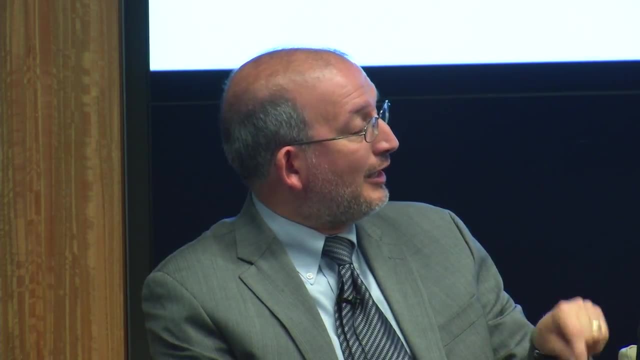 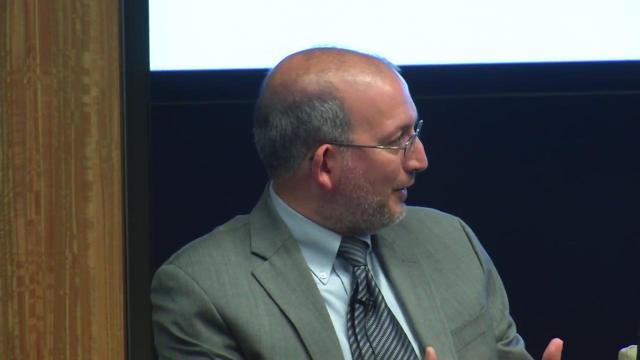 It was financial independence. You know, the budget of Inegi still has to go straight through the Ministry of Finance, unlike other autonomous institutions like the National Electoral Institute. So yes, I mean, I guess it is easier said than done. 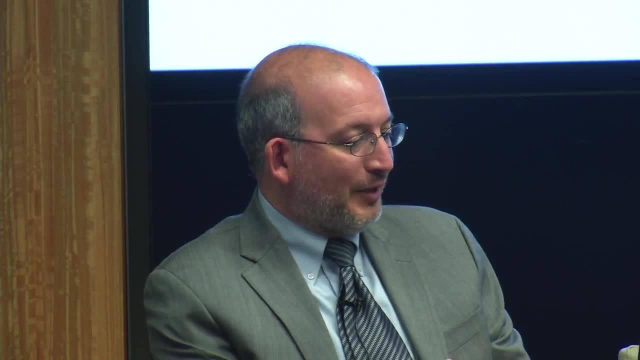 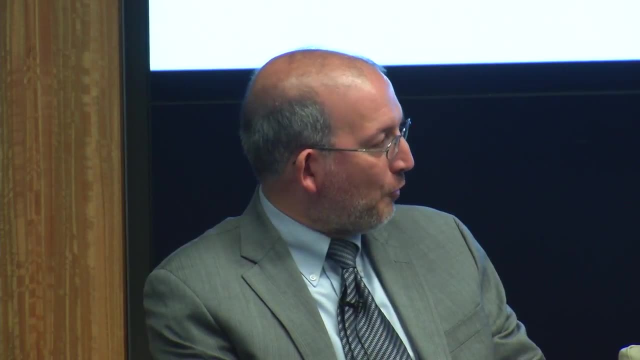 And in some cases you know when this discussion is on the table. you know people seem to confuse autonomy with autarchy. You know one thing is to work independently and another one is to work completely separately and have no, you know. 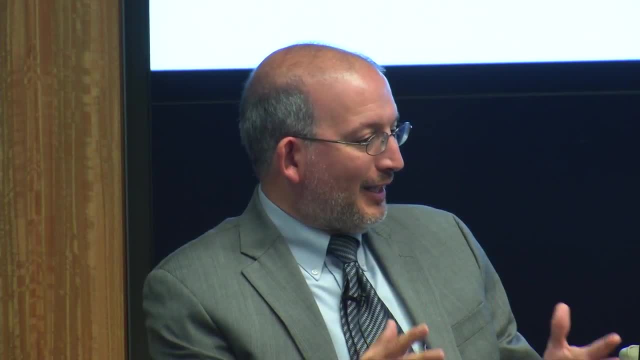 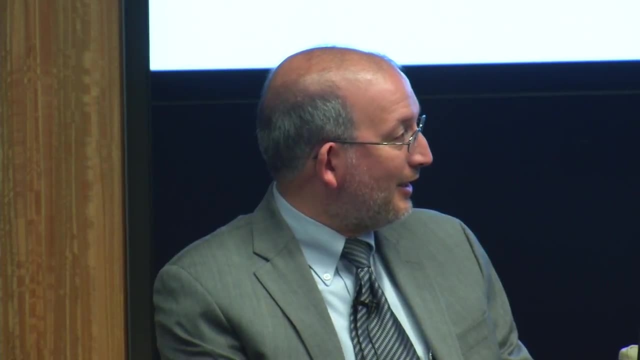 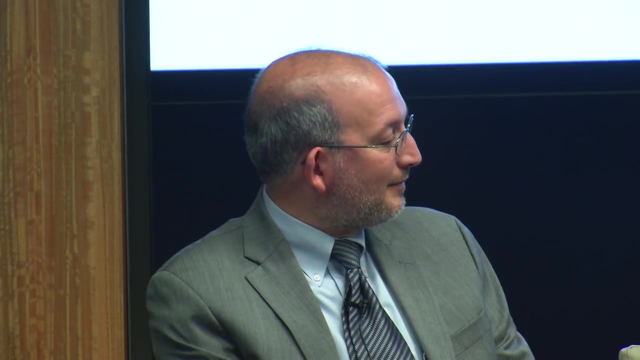 have no dialogue with the users And I think you know, as the statistical has this role of coordinating, it is important that there are these channels of communication, very clear channels of communication with the rest of the agencies in the government. Do you have any other announcements? 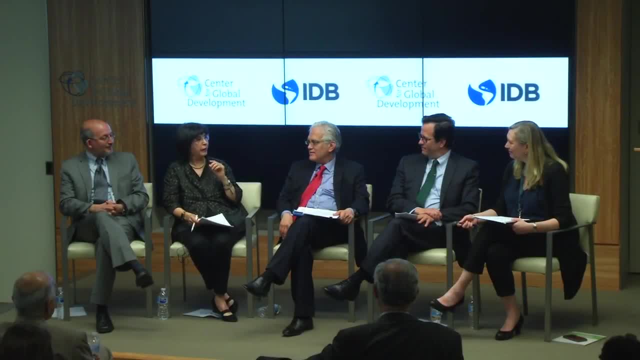 Sorry, Go ahead. Well, just one thing I think, before thinking what model works like central bank, I think the fundamentals of what to make a good modern statistical office- and the book talks about it- and one of the things that really strikes me as important is: 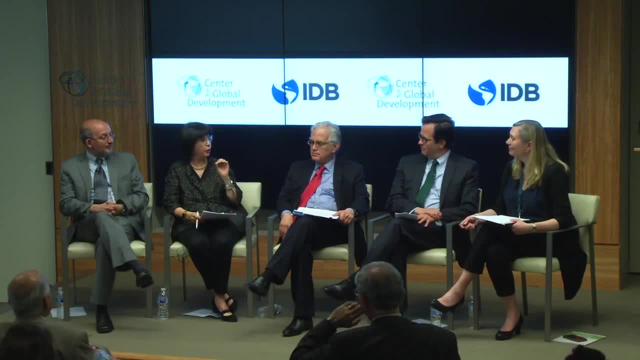 I know it sounds cliché, but increase your users base And that increasing the user base gives you a legitimacy. It gives you those informal barriers and protecting you from, you know, becoming independent, It makes you famous. It makes you independent from the changing administrations. 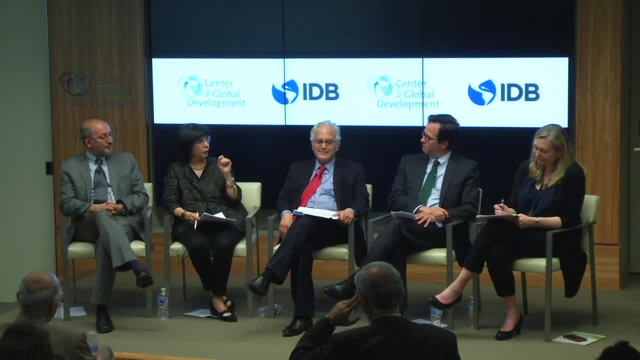 and so on. So it would be good to find those sort of important buttons that makes a statistical office really a well-functioning statistical office and then leave it for you know finding out what is how it should organizationally exist. Yeah. 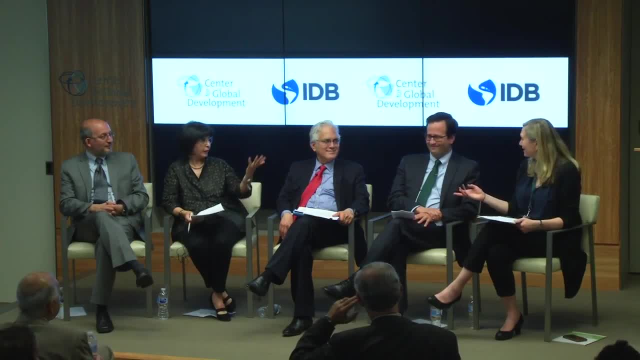 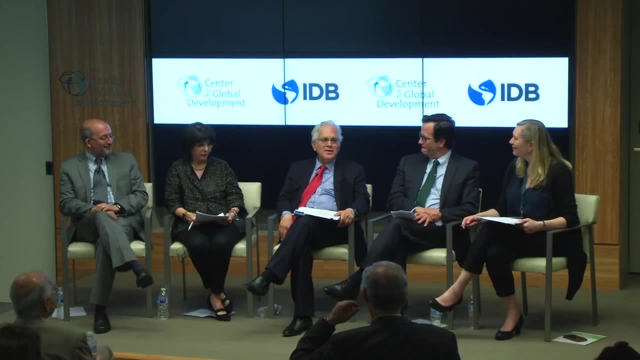 Maybe fame of your national statistician actually might be important right to protect you from Exactly And leadership as well. Yes, We've seen that in some countries. Robert, do you want to mention? talk about this topic? No, just this is a fascinating topic. 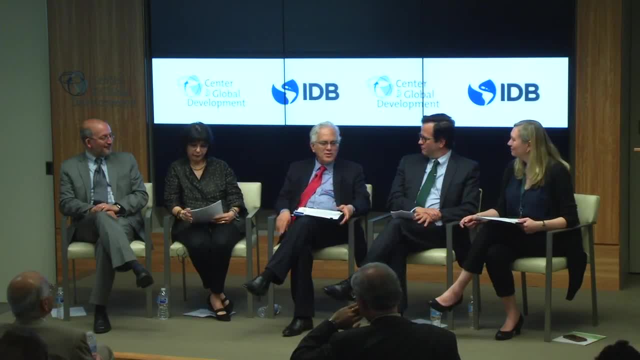 The Canadian model is very interesting. It's a mixed model, But in the end it all comes to the same thing. I think that it has to be. it is reasonable to expect that if you're this national statistician. there is a ranking of users and consumers of data. 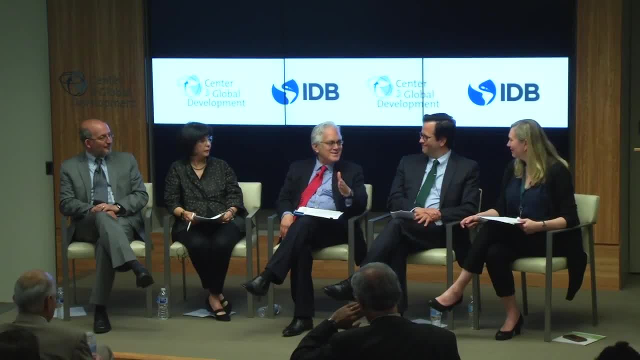 and the most important one is the Minister of Finance and the Central Bank. If you want to do something else other than what they want, you may be in trouble. You have troubles. yes, Absolutely. I challenge that. We'll fight that out later. 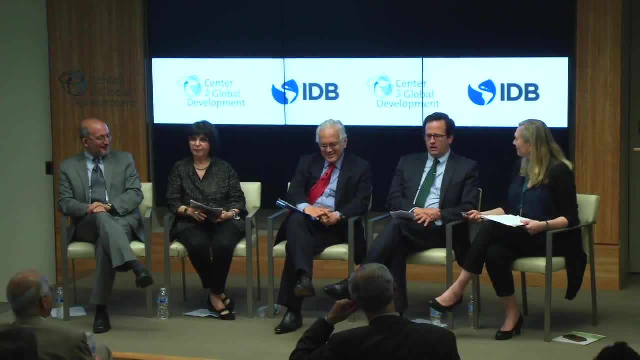 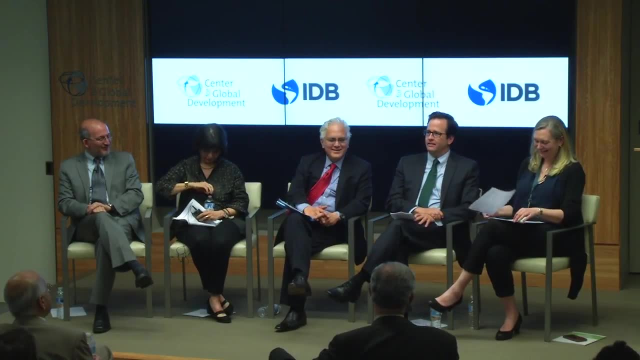 Matthew, you worked a lot in Brazil. Do you want to reflect on NPR and its role? No, All right. No, but I will say this. I mean I think, yes, statistical offices are seldom like the Central Bank. They don't have the power of the judiciary. 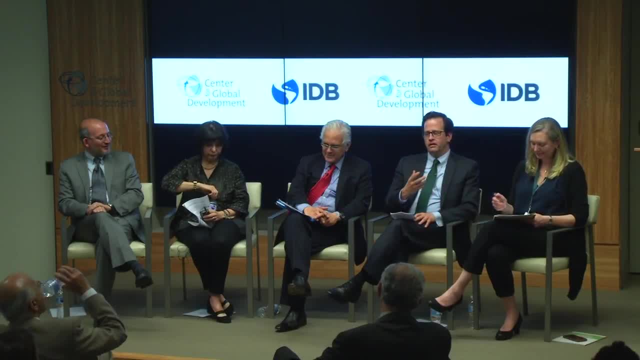 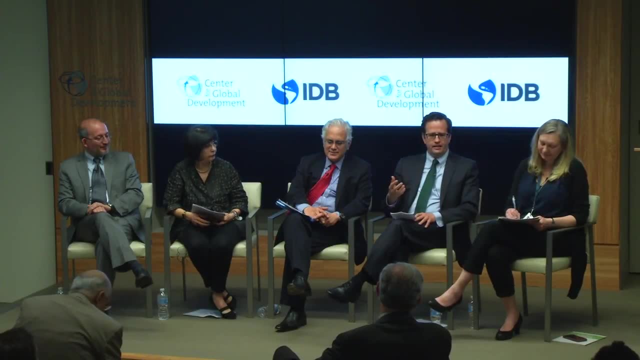 But that doesn't mean that they're powerless. And when we think about autonomy of bureaucratic agencies, oftentimes it's esprit de corps that gives bureaucrats the ability to push back against political pressure. And obviously external audiences are important, but so too are the simple de facto. 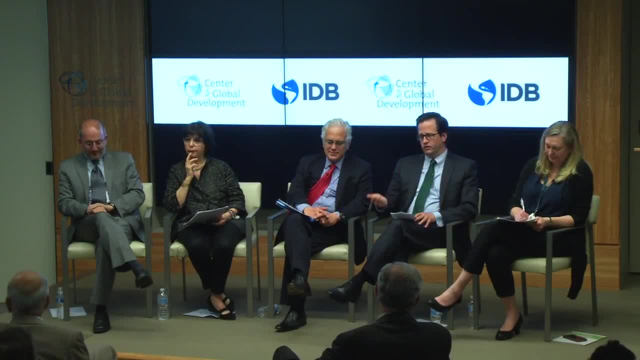 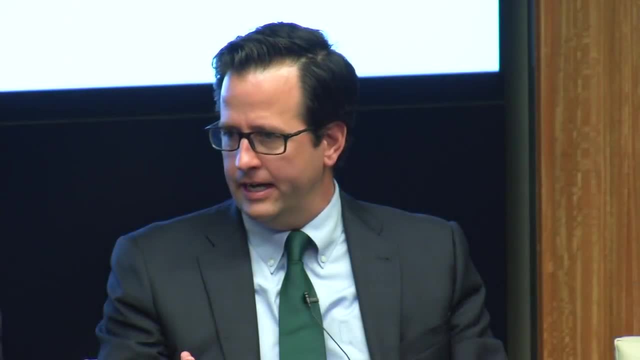 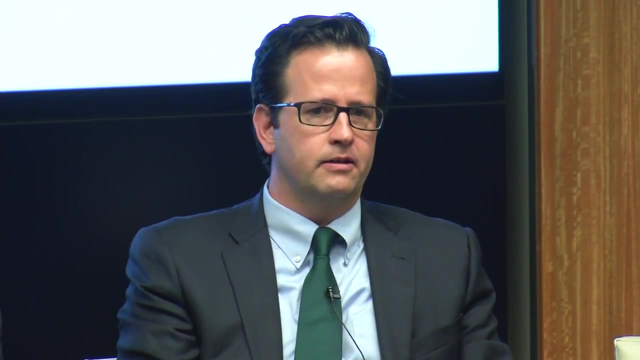 and de jure protections for civil service tenure, for civil service salaries, the things that make people stick around and turn them into experts, And so I think you know it's a combination of reaching outward but also providing the guarantees inwardly that protect bureaucrats. 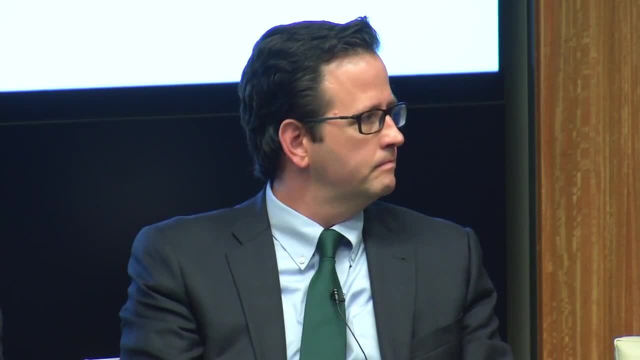 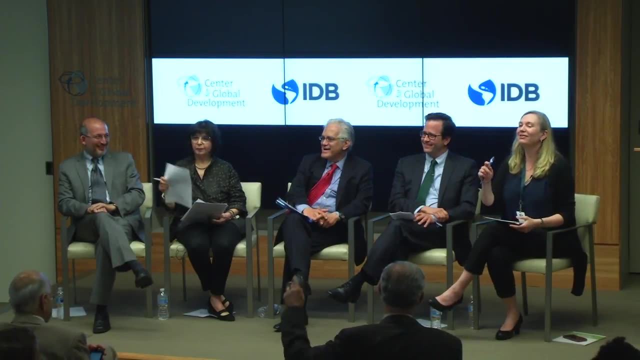 and enable them to push back against pressure. That's a really, really important point. The deep state? No, not the deep state. I was going to say that, Okay, let's go to the audience now for questions. We'll take three and then come back. 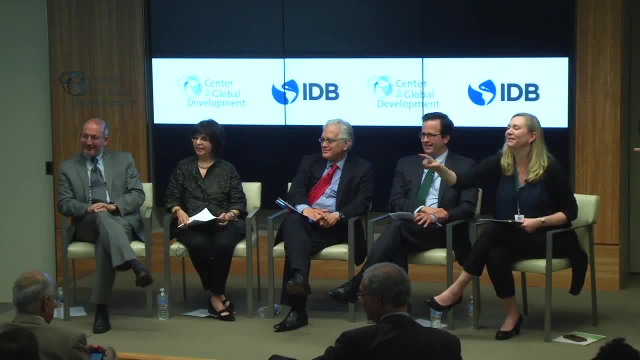 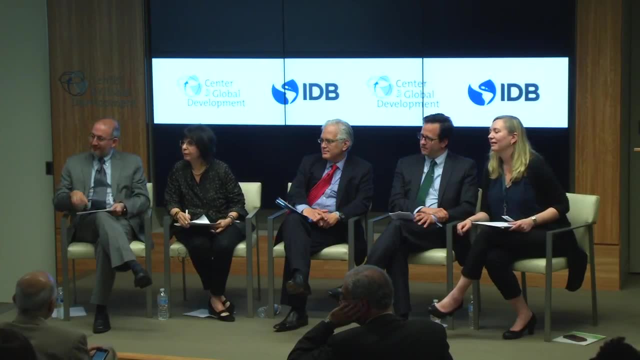 So well, you started, so we'll start over here. Please say who you are and what organization you're from. Hi, My name is Nicolas Saldeas and I work at the Wilson Center, And I have a question regarding Argentina. 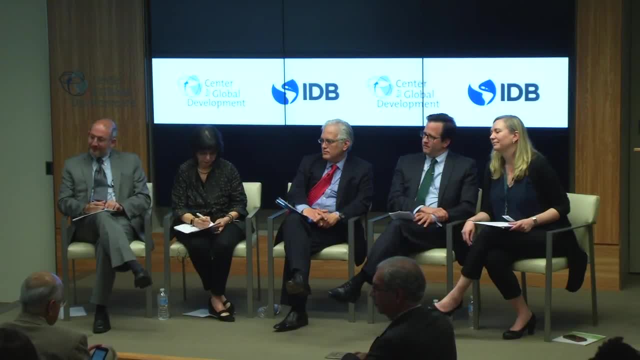 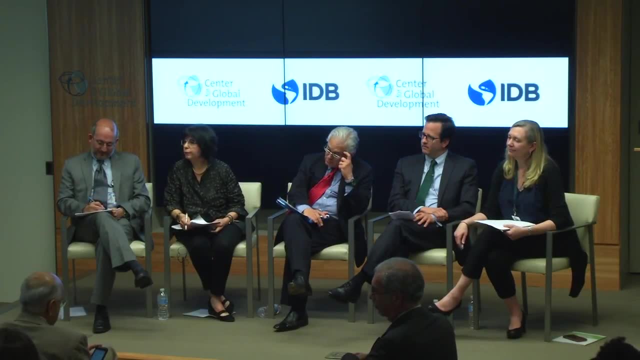 I know it's one of the case studies. Argentina was a highly politicized case of statistical manipulation and it was an election issue in 2015 with Macri, and the country went through an emergency, a statistical emergency- for the first six months, I believe, of the year. 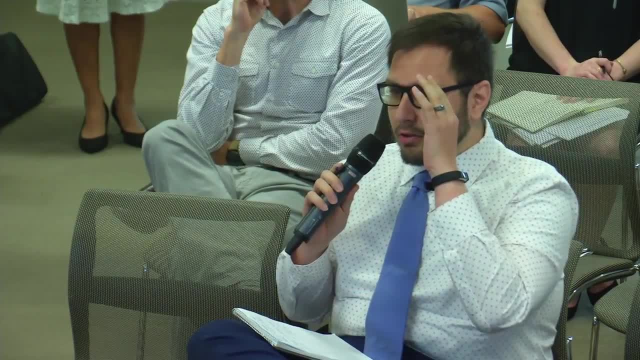 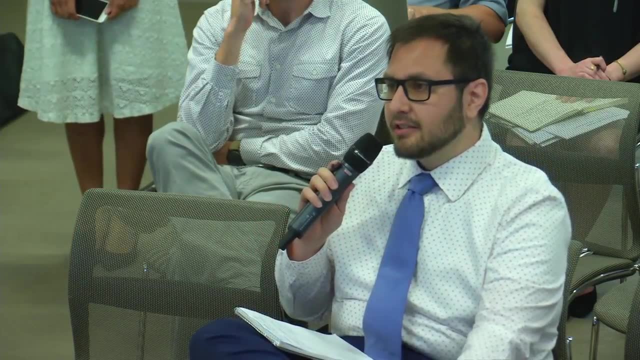 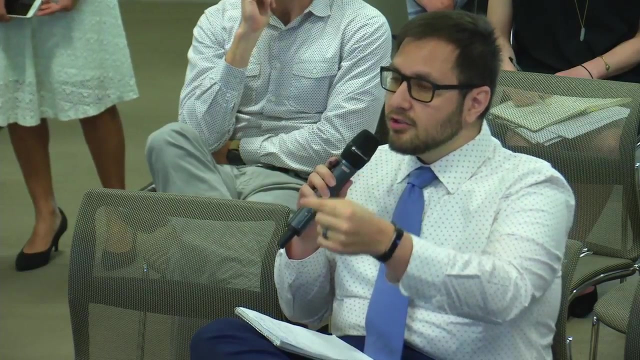 And so I wonder if any of you could talk about the role that international institutions play in helping Argentina transition back to a legitimate- I guess you could say- statistical agency, and also, what lessons have you learned from that experience for future cases like, for example, Venezuela? 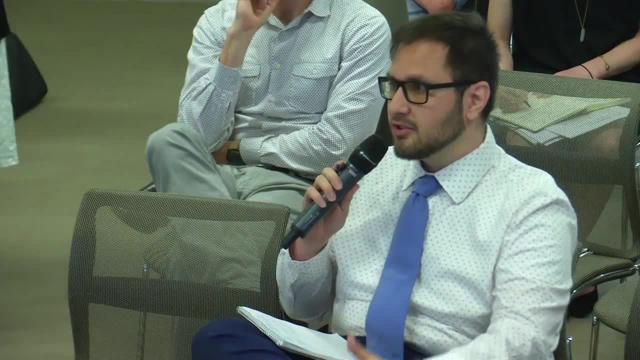 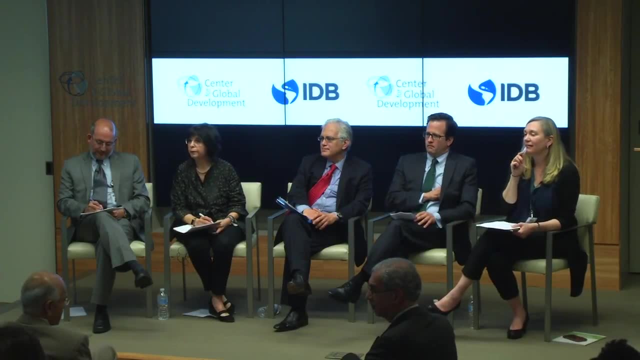 which almost certainly would face this even worse situation. Great, great, great question Right behind you and then Hi, thank you so much. My name is Ben Rose, I work at the IDB And this question is mainly for Roberto. 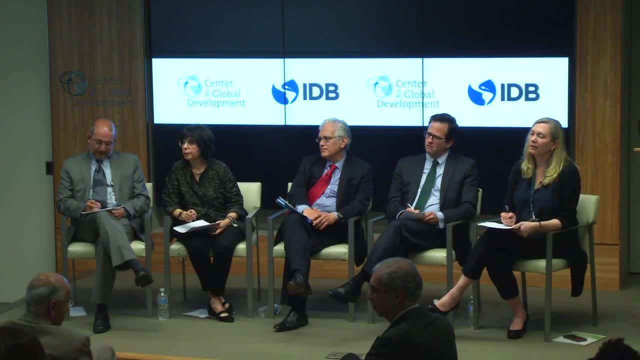 but I'm happy to hear the opinions about it. You talked about the importance of the Minister of Finance and the role that he or she plays in making the allocation budget allocation decisions and the importance that he or she assigns to official statistics. Jose Antonio and I have spent some time. 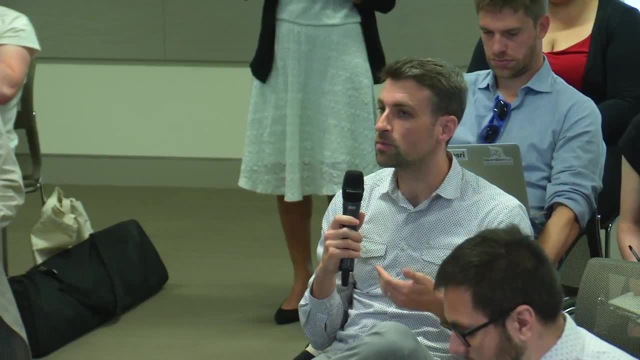 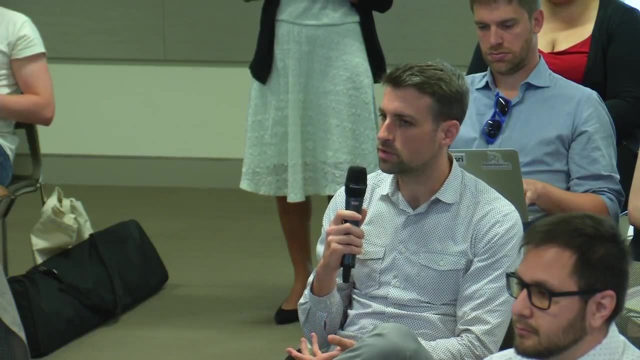 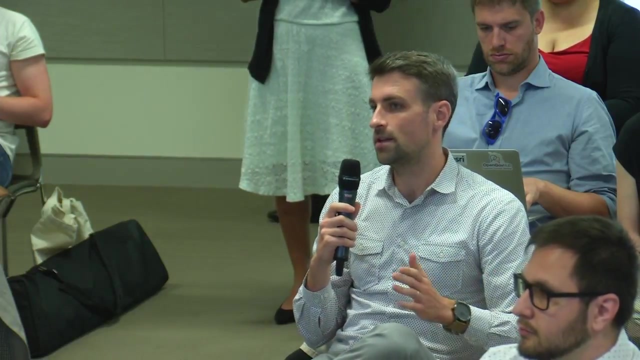 reflecting about what kind of arguments would be most persuasive to this important figure within government who, at the end of the day, is very influential in determining what kind of support is given to statistics offices and everything else in the expenditure portfolio, And I think statistics offices. 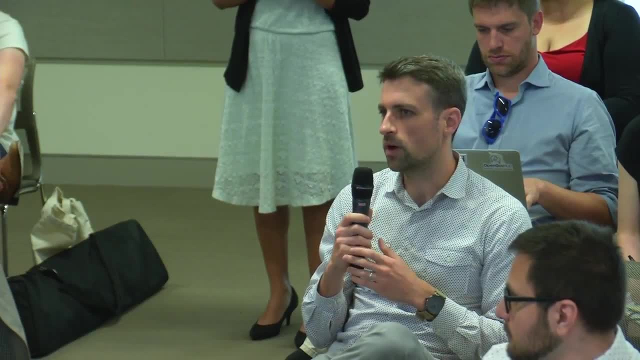 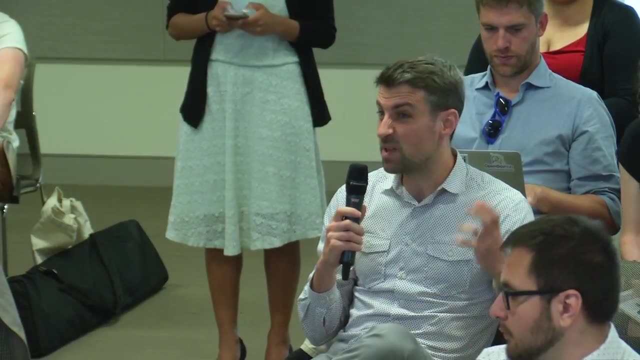 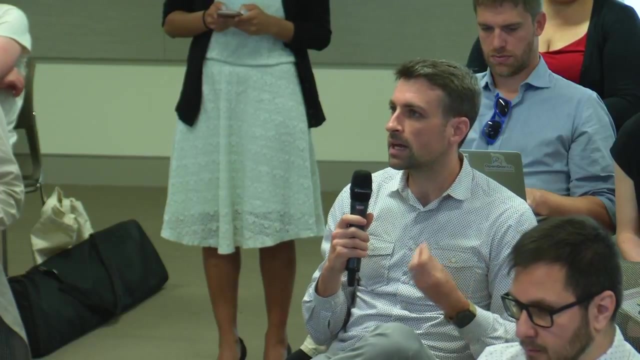 are kind of at a disadvantage when comparing to other budget items. Take an airport. The airport is really visible, It's big, It's shiny And the volume is just huge. And also it comes from a sector that is highly experienced in doing cost-benefit analyses. 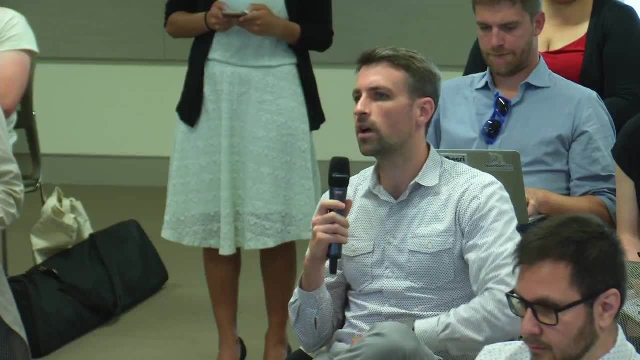 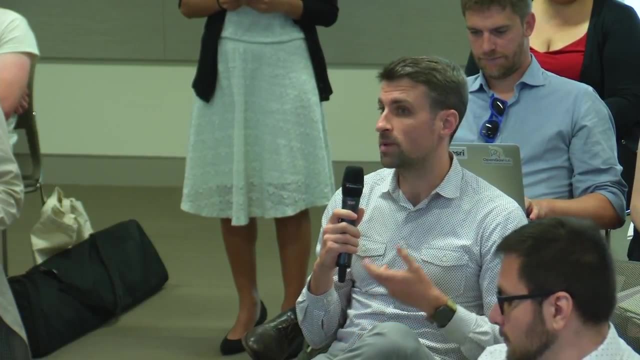 So you can hire an economist. you can say: give me a return on investment, projected ROI- for this airport, And you can get that number. And the number's going to be astronomical probably, But in statistics we don't have such a tradition. 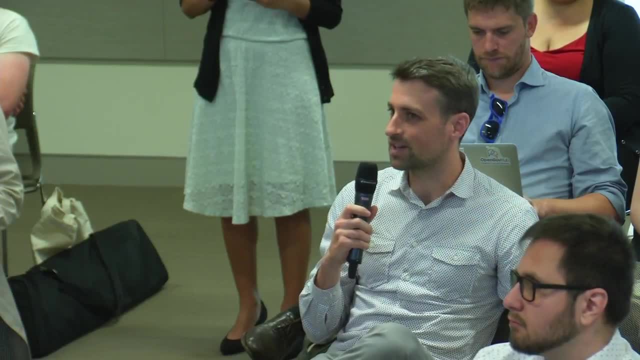 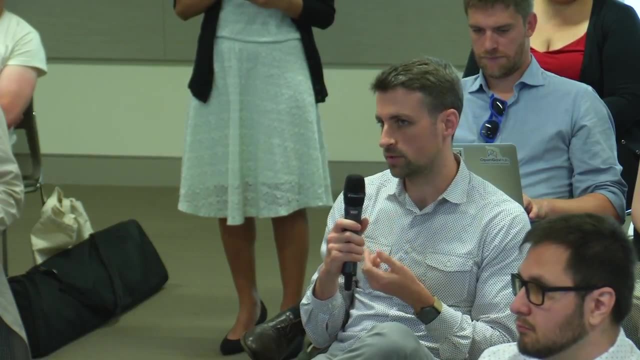 and also it's never going to be big and shiny in the same way that an airport is. So my question for you is what kind of arguments would be most persuasive to the Minister of Finance? Is the key finding an ROI kind of argument? 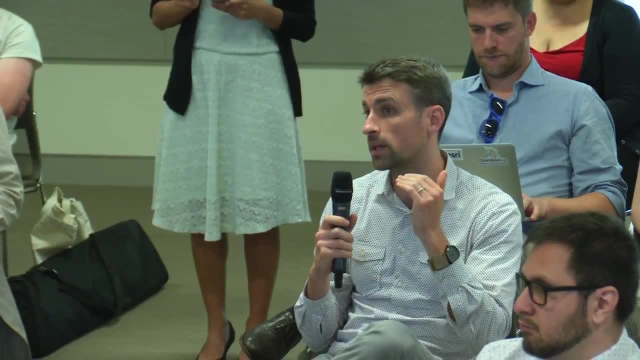 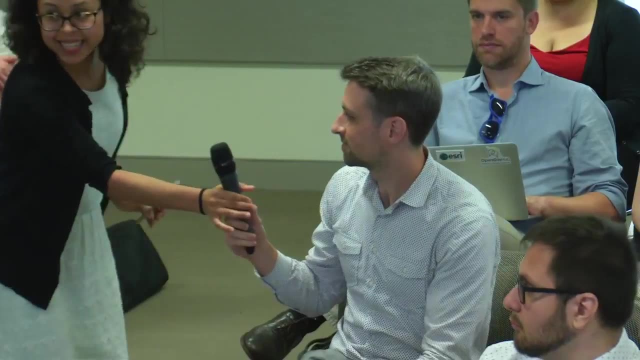 Or is there something else that would really resonate? to put it on the same plane as the airport type of case? Thank you, Is data as good as airports Over here? Sorry, Sorry, Okay, let's go. Actually, the person right next to you. 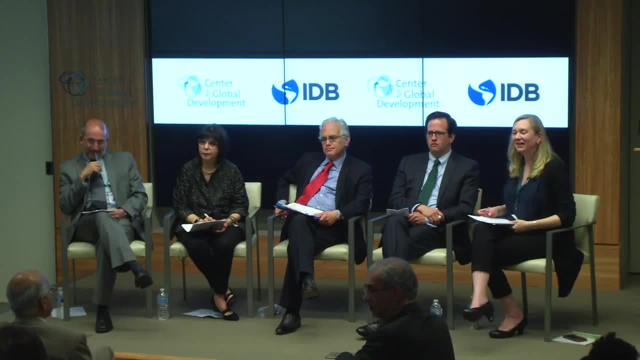 since you're standing there. Yeah, And then yellow. My name's Kenan Scott. I work at the World Bank. Congratulations to Jose Antonio. Much of what this book says resonates very well with me. We worked in this area for a long time. 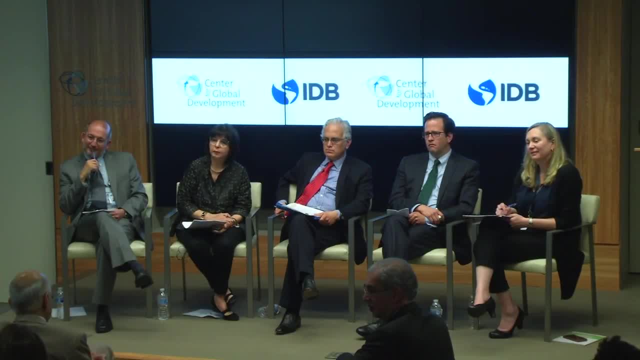 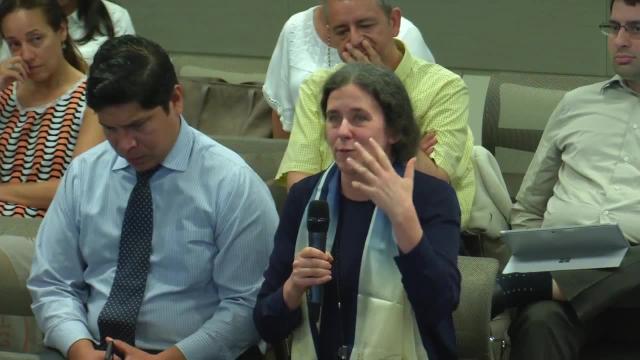 I have a comment and a question. So the comment is on the data users. Just to defer a little with the panel- is that creating that data user group is not just to create more demand for different data, It's actually to A get the data that they are used. It creates. governments come and go, Some are more open, some are more closed, et cetera. If you create a community of data users, they don't let you shut the door. I mean, I think that the data users aren't creating more demands on the system. 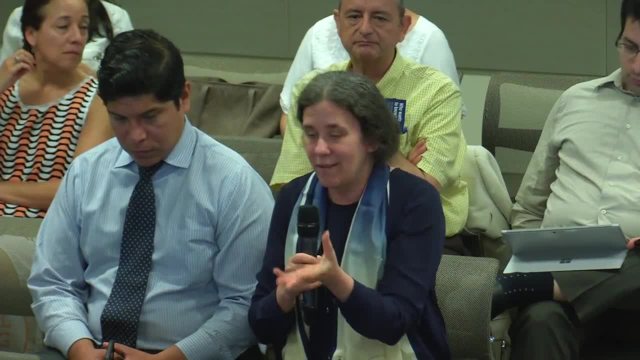 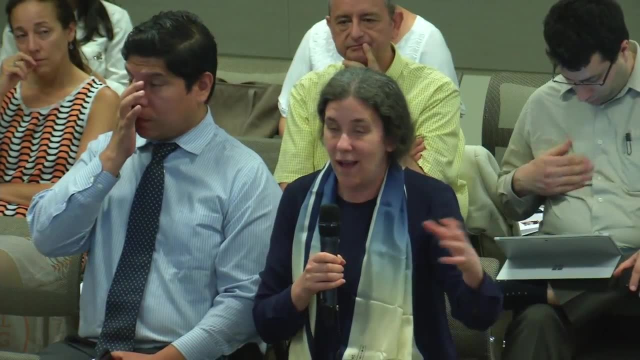 to create this database, that database, the other one. They actually just want to see the basic data, That, the same data that the Minister of Finance wants to see, The same data that the Ministry of Education wants to see. I think, if you create that group of people, 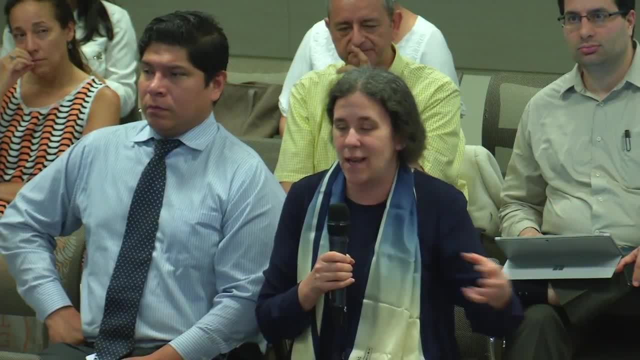 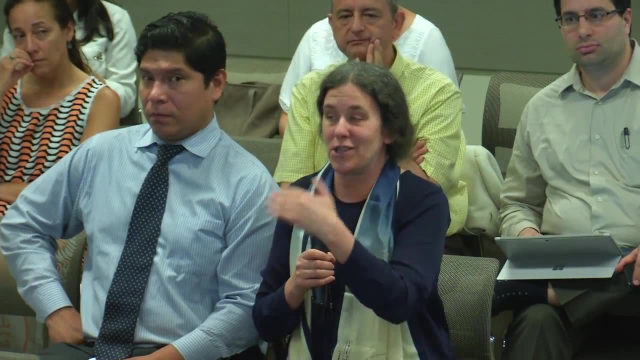 those you know- the academics, the think tanks, civil society- you create something that will do better at pushing the conversation with the Minister of Finance going forward than just chatting On the question. in the Africa region there are four, I think. 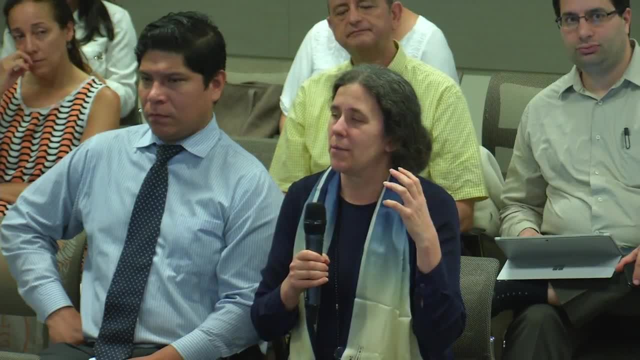 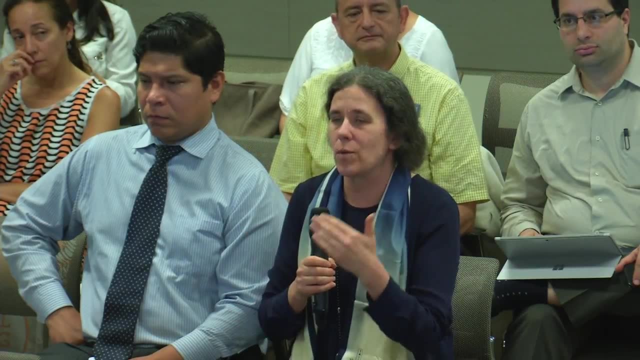 or five statistical institutes, training institutes, not national statistics office, but institutes that their job is to train other statisticians, And I've always wondered why they do it at the you know sort of short courses, technical training courses. They have bachelor's degree, master's, 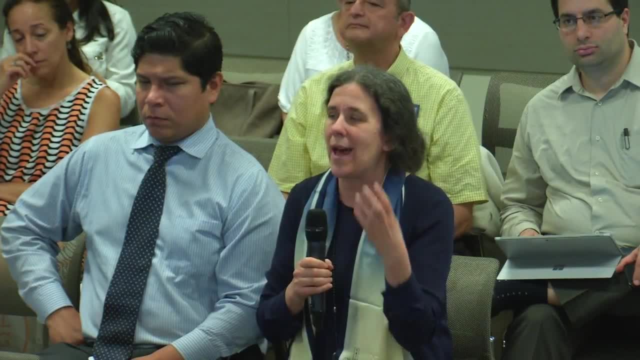 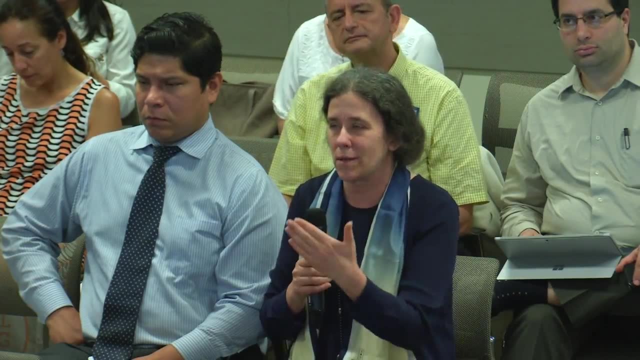 some of them now have PhD level courses And I always wondered why Latin America never generated that kind of a system. Inehi plays the role a little bit, but not really. They don't have programs of their own. They're just sort of a center that other people use. 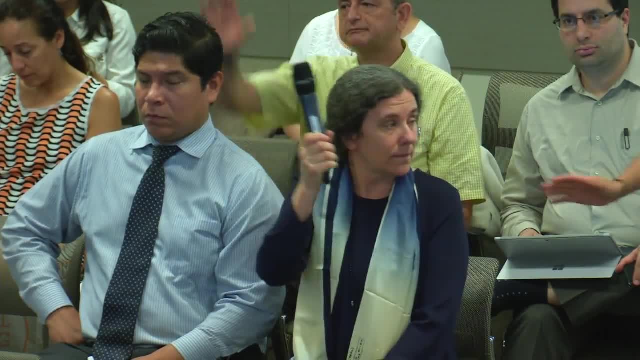 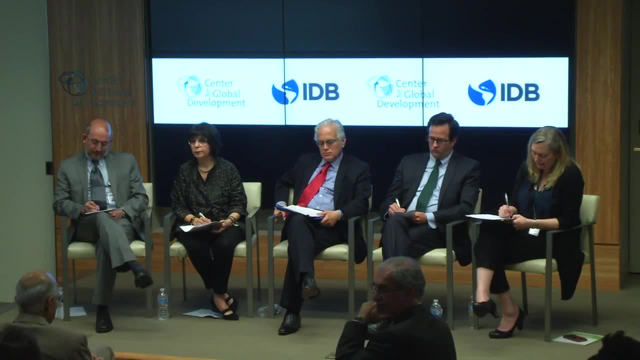 So I was curious if anybody has any insights on that. Yeah, that's a good question. Right behind you in the yellow shirt- Congratulations. My name is Jose Antonio Escamilla. I'm kind of representing PAHO, the Pan American Health Organization. 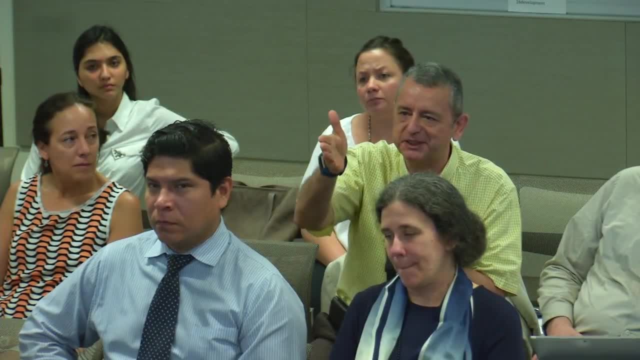 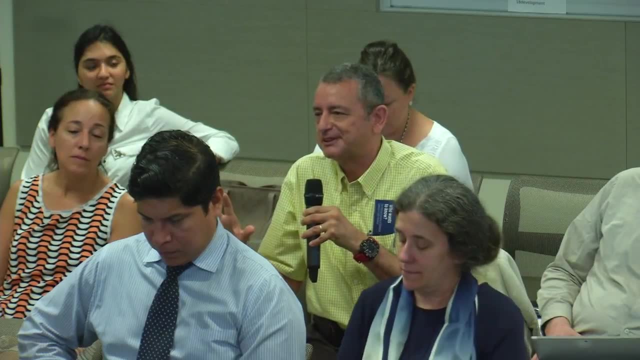 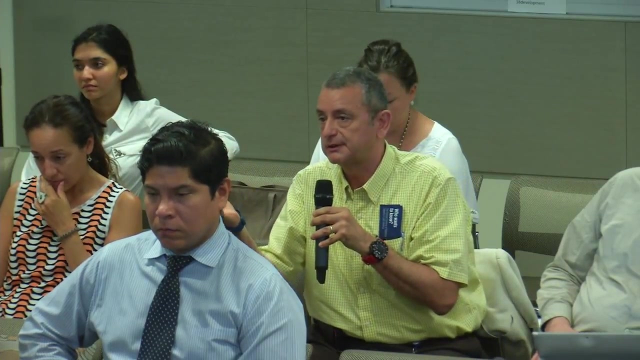 I like many things. First of all, I like your analogy of the DNA And in that regards PAHO, this year kind of did some surgery there and we have now trying to push up all the issue of data and data use also for health analysis and stuff like that. 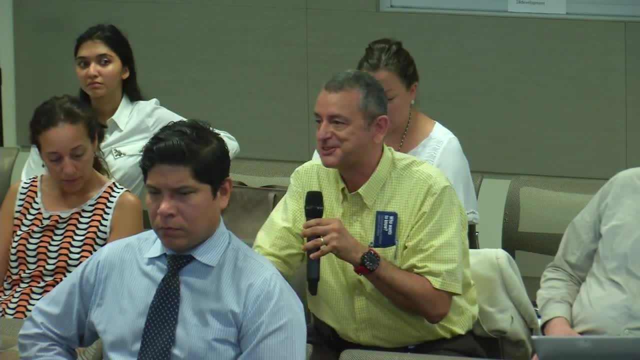 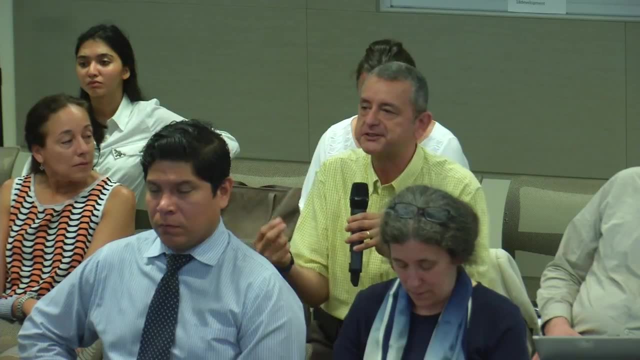 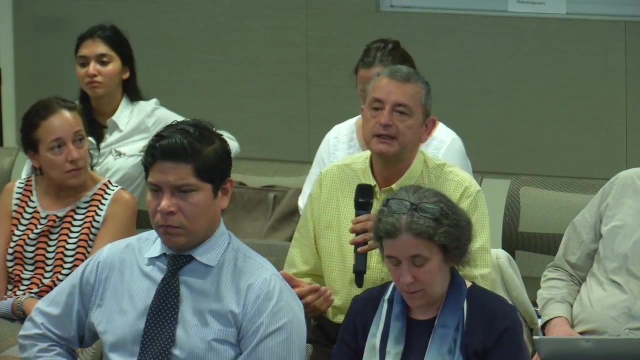 So I'm really hoping- I'm dying to see the book, the case studies, because probably I'm going to find some clues on how to increase this constant questions on how the role of international agencies can be working together and improving all this, not only data availability and quality. 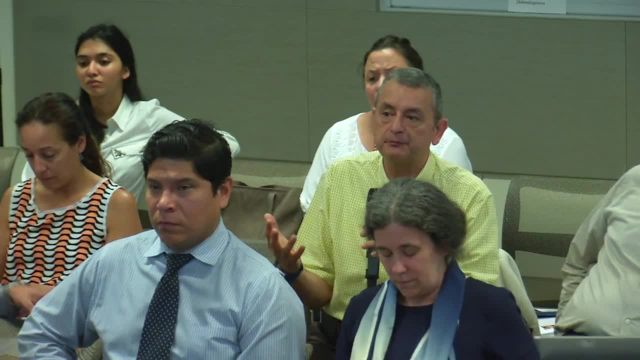 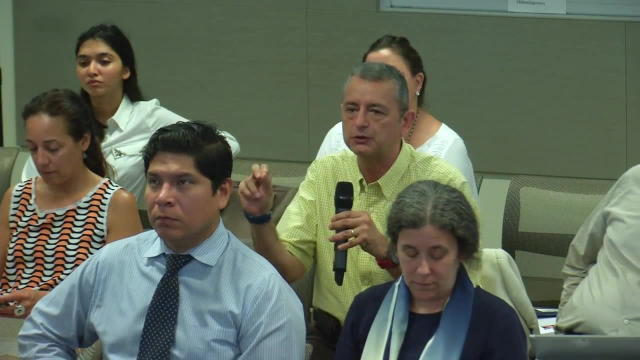 but also the use of that. So my question very quickly is: if you- because I haven't seen the case studies- if you pay some- look some specific look at the health sector. I don't know if you can mention something about this. 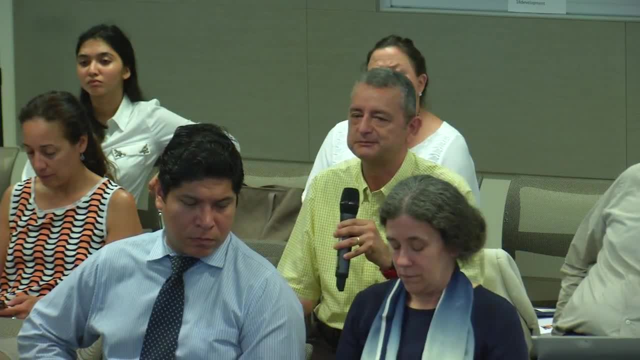 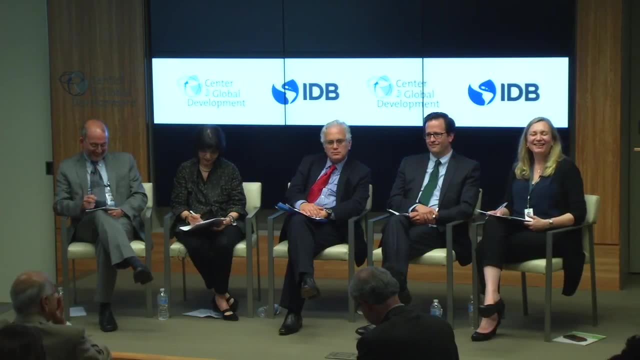 because of course for us it's kind of our main counterpart in the countries. I am happy to answer your question later. Yeah, thank you. My name is Tina Faulkner. Thank you so much for the presentation. I work for the Department of Labor's. 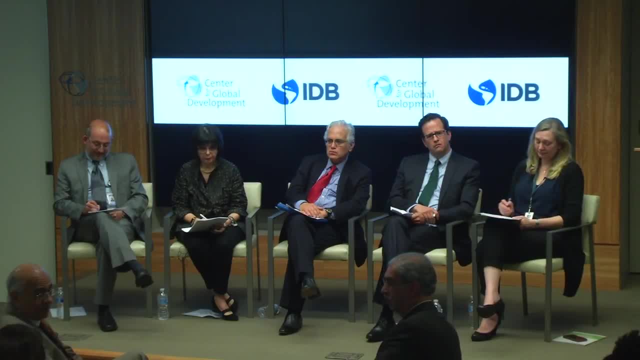 International Bureau, specifically the Office of Child Labor, Forced Labor and Human Trafficking, And we don't have a lot of money but we have been funding supporting sort of stand alone and modular surveys on child labor and forced labor in some countries. 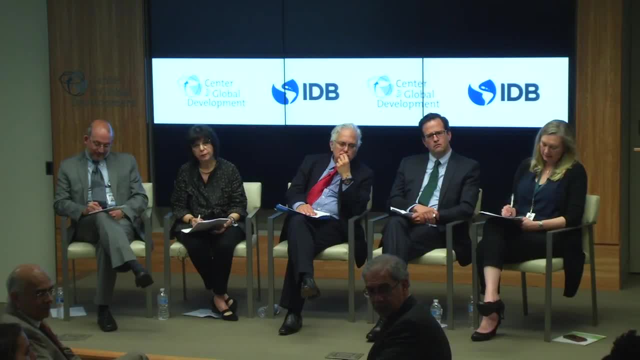 And I was really interested in the comment that you made during your talk, Jose Antonio. You said that sometimes it can be difficult to get the data published and get it out there because it might make people look bad. It might be difficult for the government. 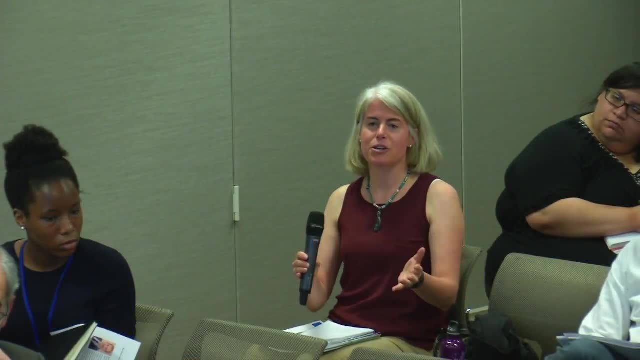 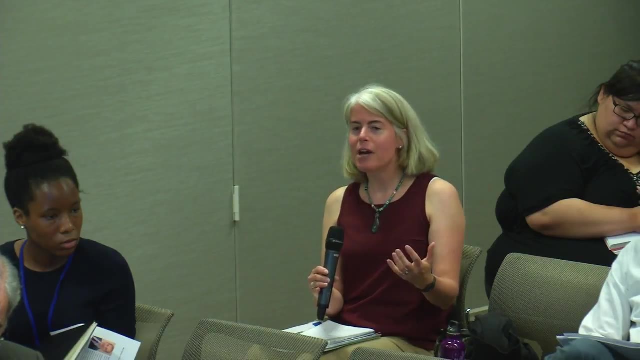 to want to sort of show its dirty laundry. This is obviously an issue that we deal with a lot, And so I would just be interested in hearing any more thoughts you have about that, if you had any examples of successes in sort of convincing that in the long run. 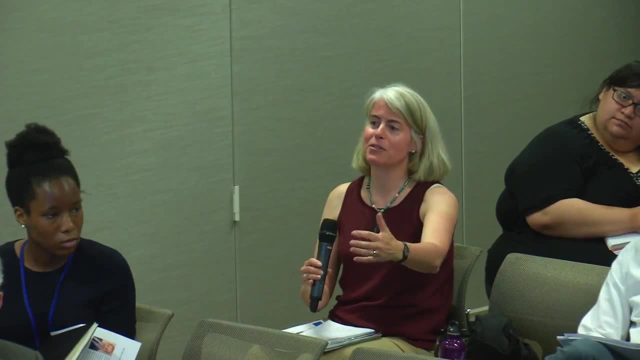 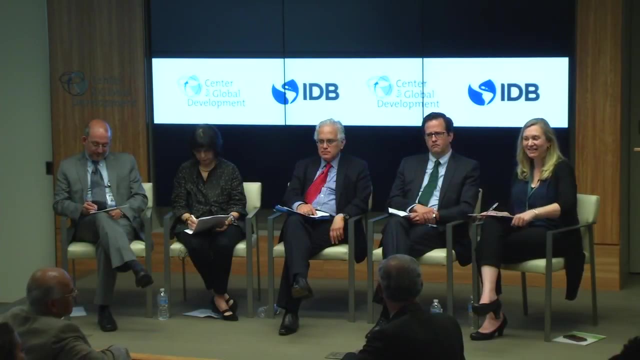 having that data out there would be beneficial. Thank you, The bad news question. And Santiago, do you want to give the last comment and then we'll go back to the panelists? Sort of a comment on the expanding the base of demanders or the demanders. 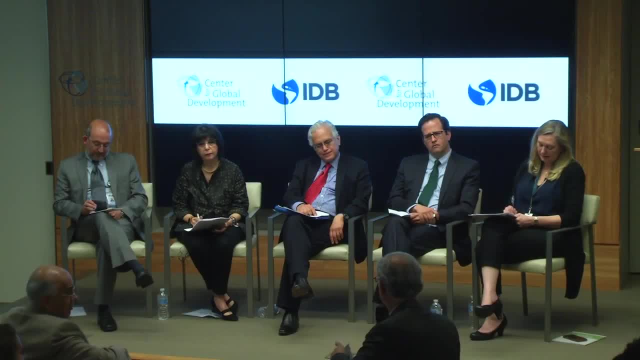 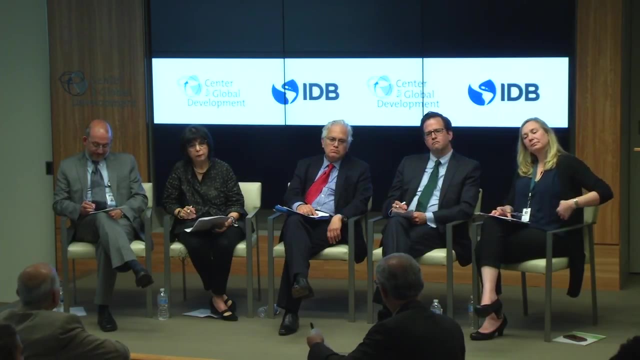 I think in the region there is a lot of demand for data. I think an important factor in the region is the role of Congresses, Because now many laws have rules for distributing resources, like revenue sharing formulas on a per capita basis, depending on the population. 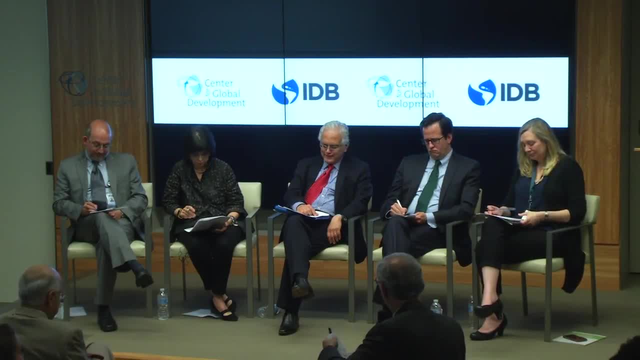 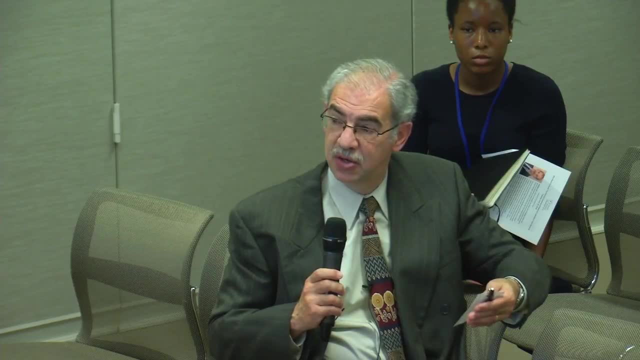 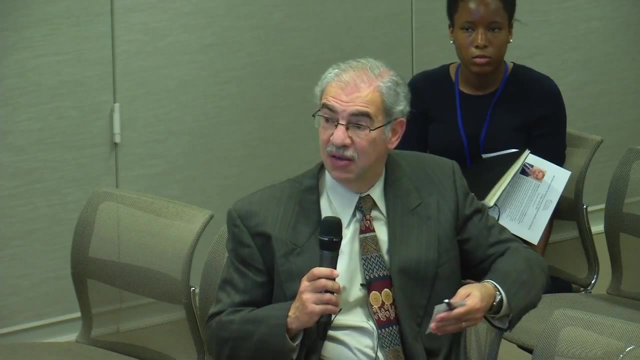 or the income level of the states. So clearly, Congress has a stake in having good data to apply these revenue sharing formulas, And many countries also now have mandates to measure social indicators, to measure poverty and to allocate some resources on the basis of poverty indicators. 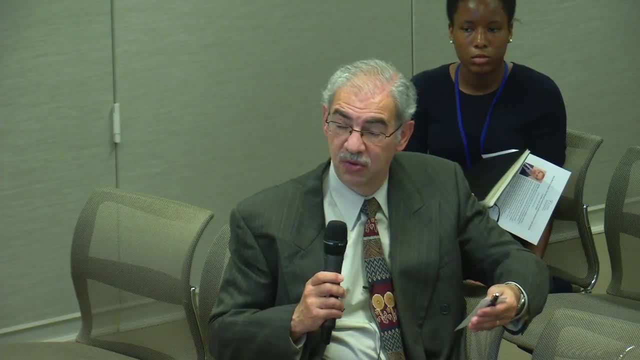 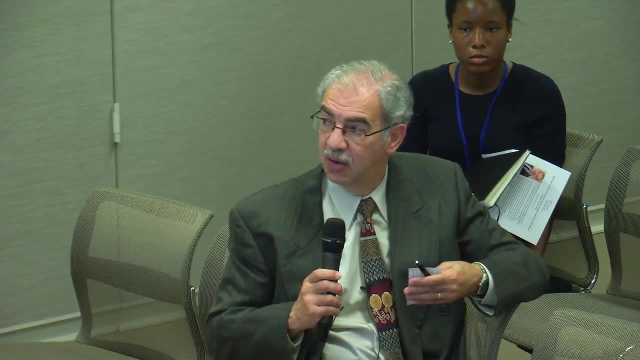 So the more this is done and the more this filters into other laws, the more now there's an ally in the state, not exactly the finance ministry and the central bank, but also in the state, which are congresses which are demanding that better data is there. so they 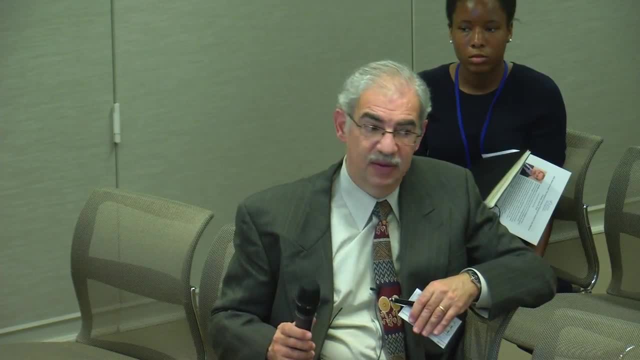 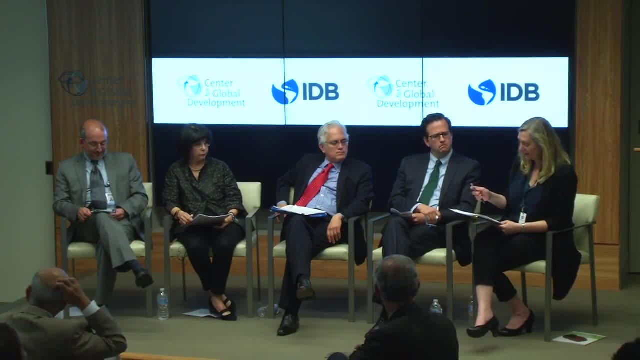 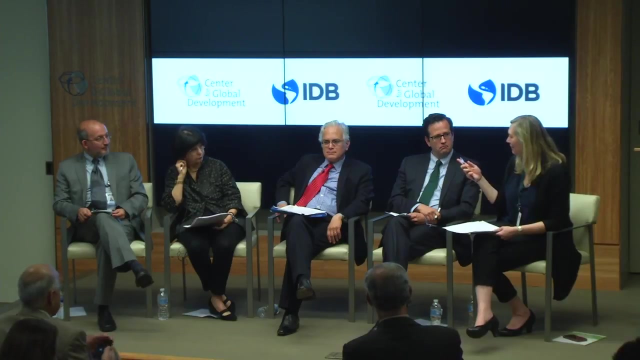 can sort of apply all these laws. Yes, That is also a very interesting political economy issue. I hope you'll Okay. so we have the very interesting question of the statistical emergency and what was done to support the Argentine authorities in their transition. 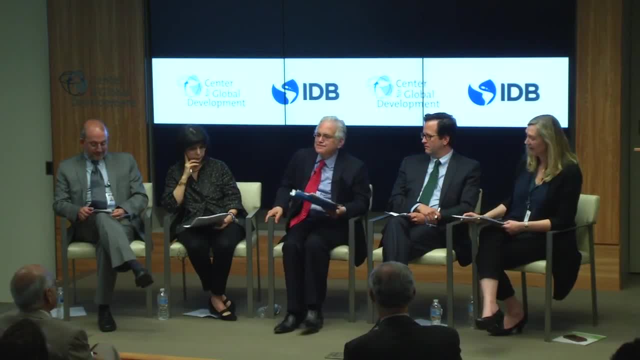 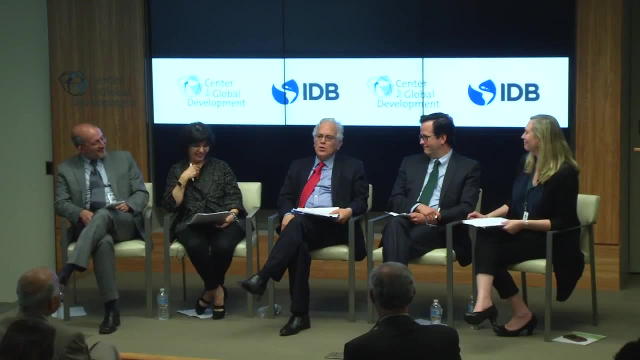 Maybe Roberto will start with you, then ask you Pepe? and then you know what about Venezuela? You know, in 2014, I went to work for the statistics department in the fund and I told my wife: good news, there are no statistical crisis. 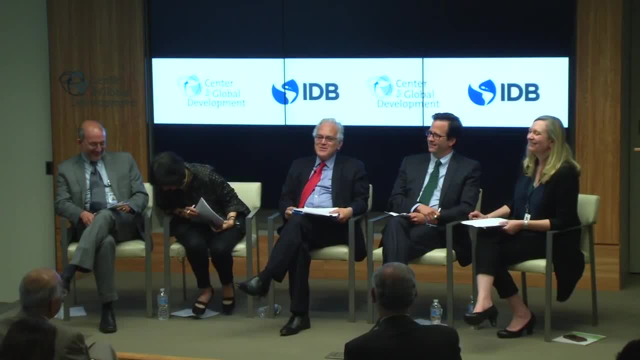 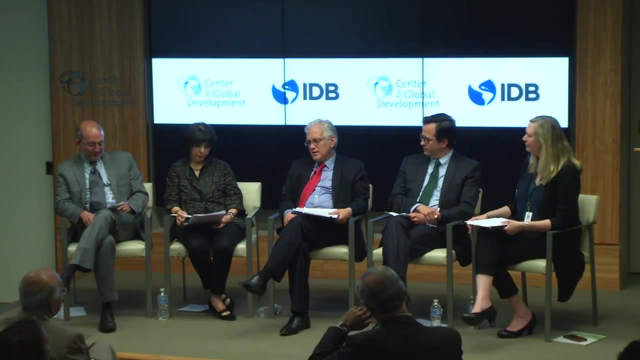 I was wrong? No, Because there was one in Argentina. Yeah, so what did the fund do? The fund has some constraints in a situation like this, because this is the case of the public, the international community, even political parties accusing the government. 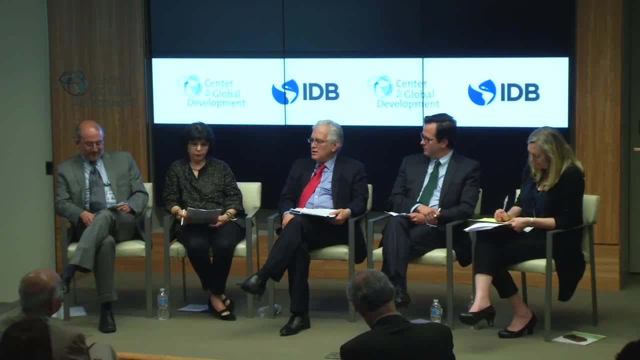 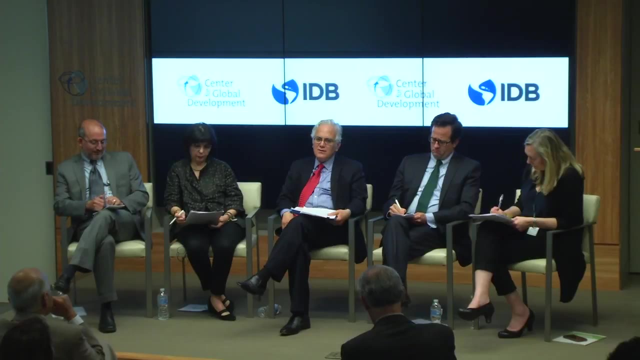 of lying and you know manipulating the data And you know the government, like other international organizations, work with the government. We don't work with anyone else. We go and work with the authorities And so it's a difficult, sensitive matter to say: you know we suspect you're lying. 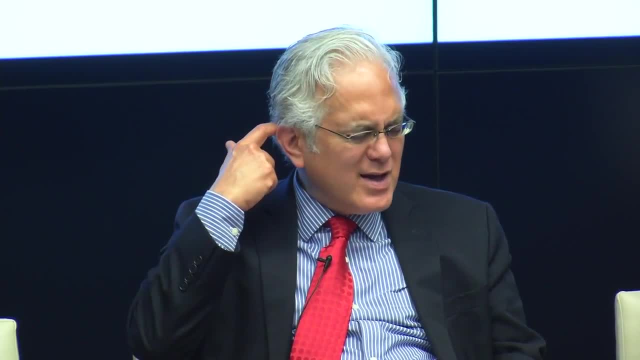 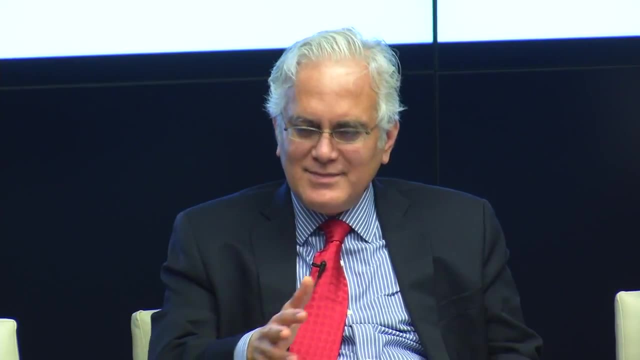 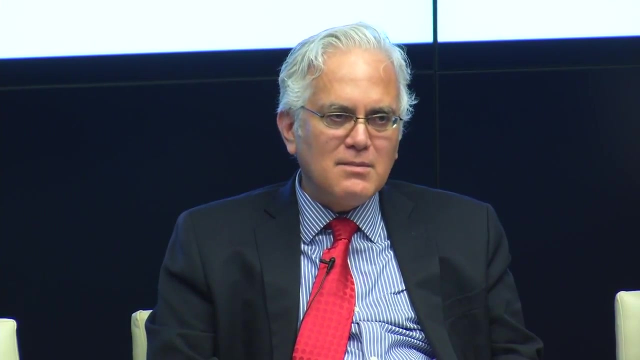 open the books so we can check. In that particular case it was very. It took seven years, six and a half, for the authorities to let us look a little bit at what they were doing And even then, after You know, working with them to the extent that they allow us working with others, we 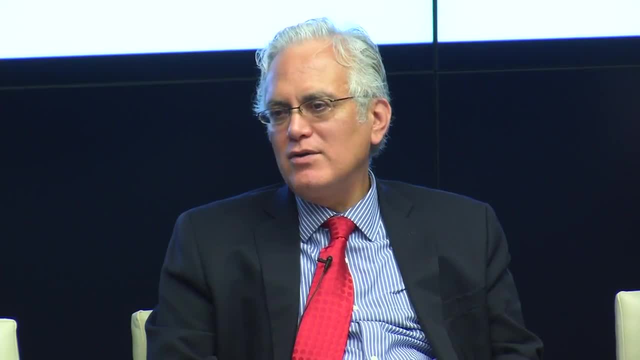 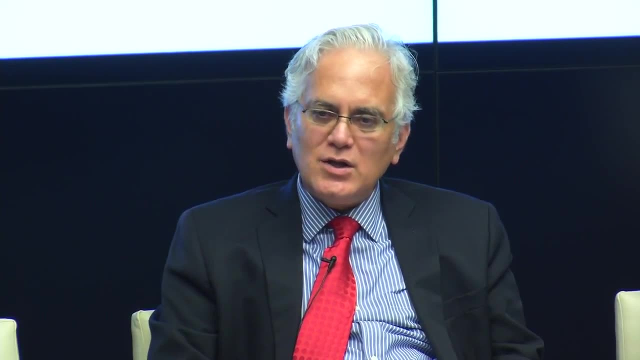 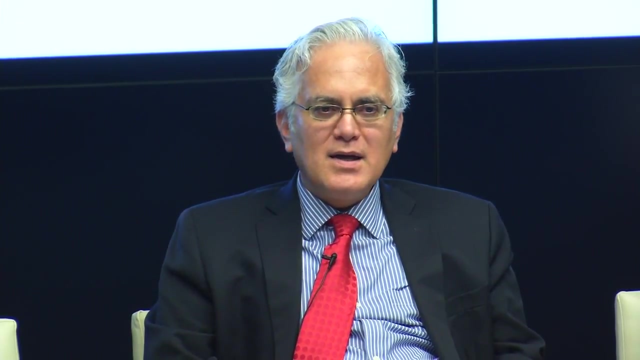 could not find how they were doing it. We realized it only once the new government came in And you know I have been arguing in the fund that we need to learn a lesson here. My colleagues are still not where I am in this area. 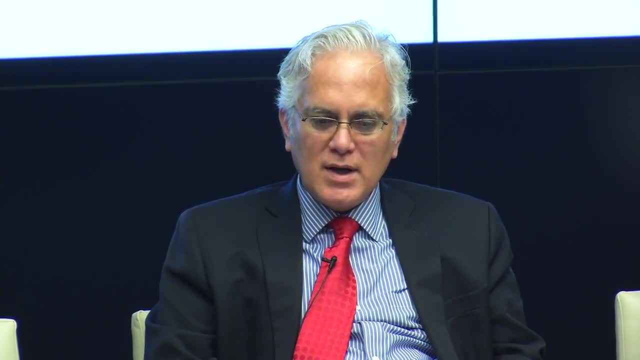 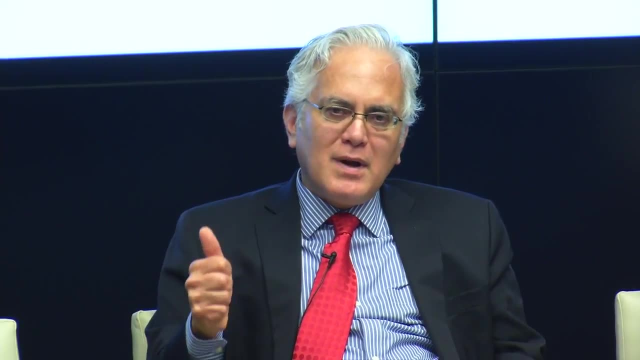 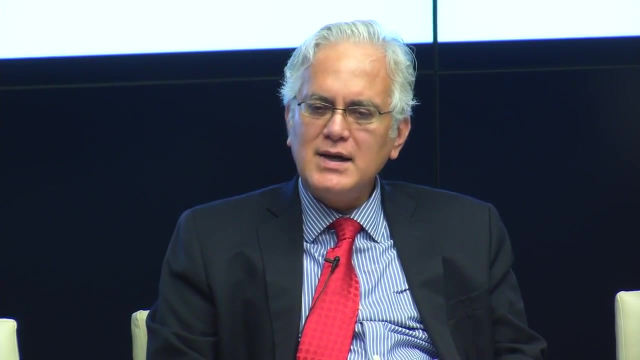 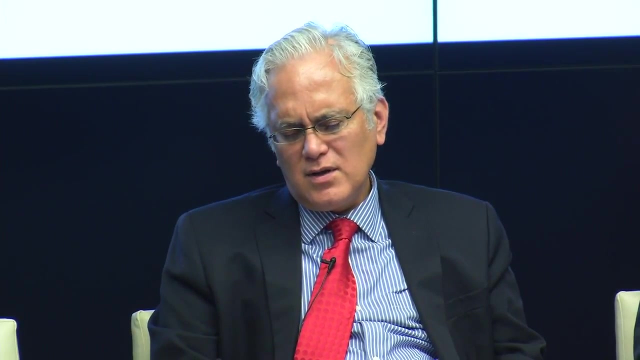 I think that there are situations. There are situations where the onus of proof should not be with the fund staff but with authorities. Now one specific, The only specific lesson that is being applied today is that users are very important, and we recommended to Todesca, the new head of INDEC, that he should form a council of users. 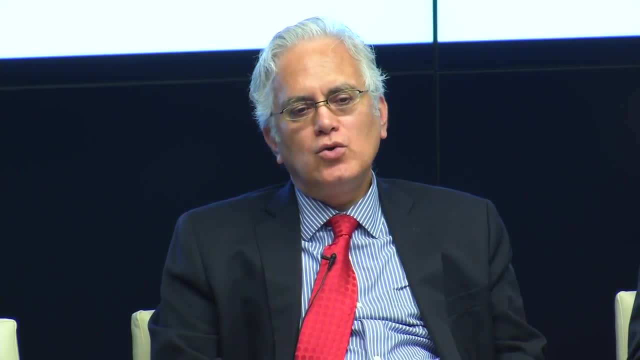 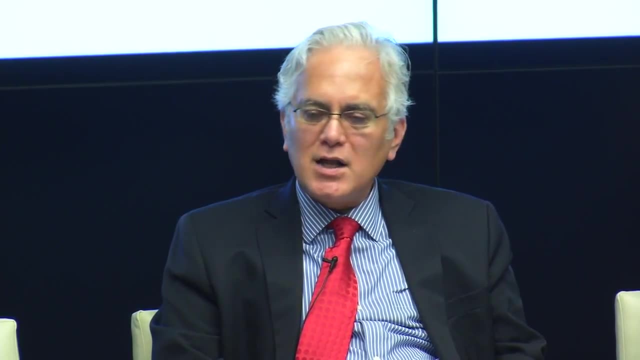 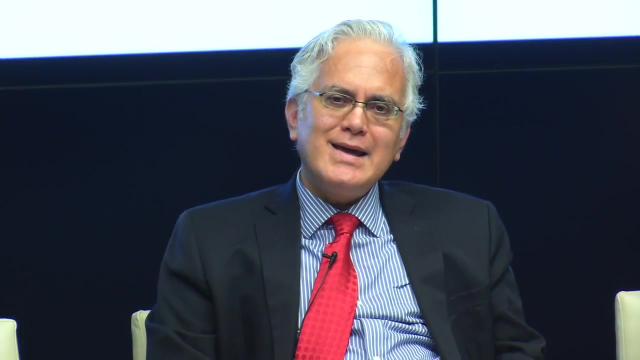 that will enable him, Mm-hmm, Mm-hmm, Mm-hmm, To get an informed and perhaps even powerful view of the quality of the statistics and the credibility of the statistics. One other lesson that I would take from Argentina is the following: 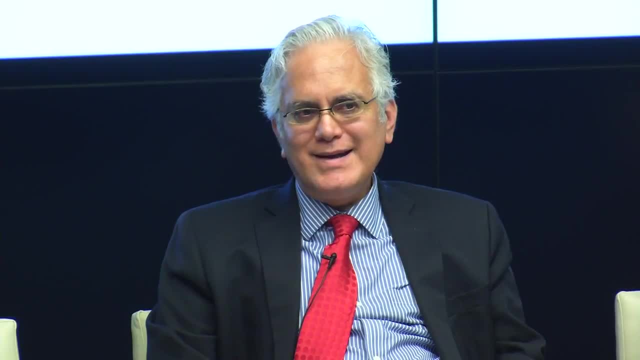 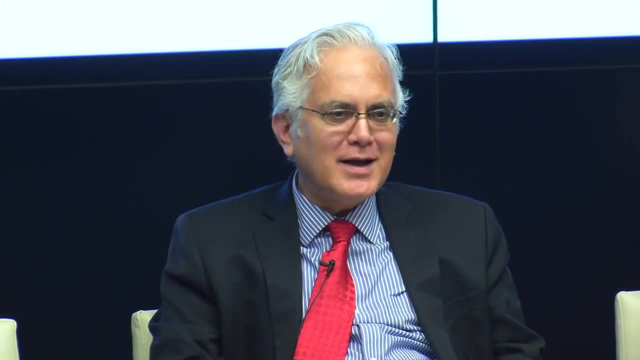 If you see in any country that there is a competition for the CPI or for GDP, that there are others producing data and that people are paying for that data, there is a problem. That is the. There is a market problem, There is a market test here. 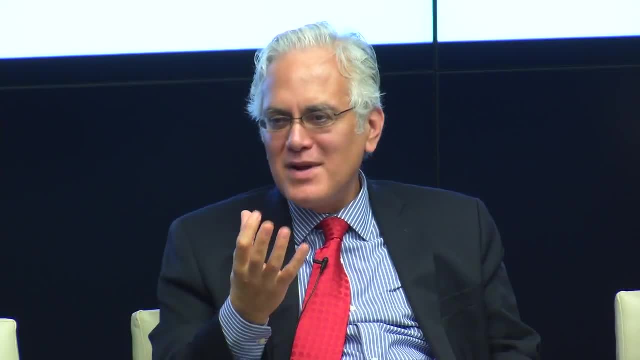 Yeah, If the public doesn't believe you and they are buying the data for someone else, there is a problem. That is interesting. Maybe we can add that to the index, Although I think in the US we have a lot of groups that do that. 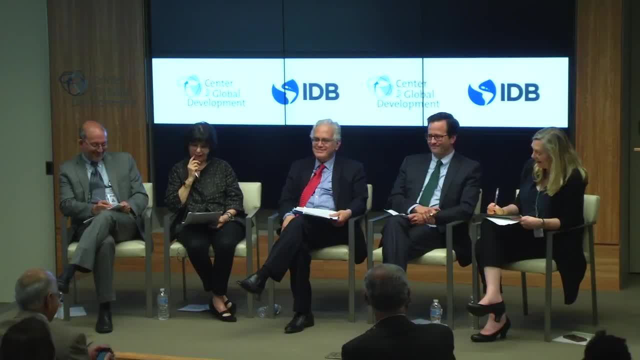 Pepe, do you want to? Yeah, No, I think when we started, when we were looking for the case studies, of course, part of the possibility was the agreeability of the country to be subject to a case study. Mm-hmm. 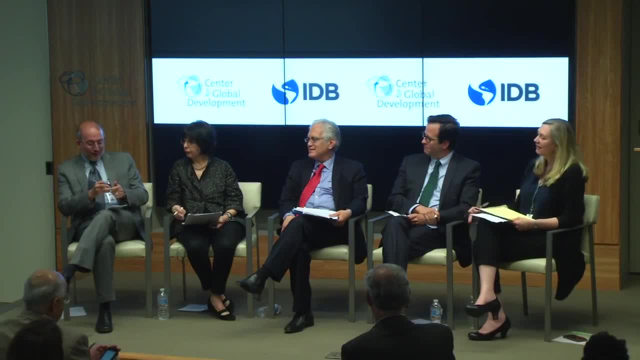 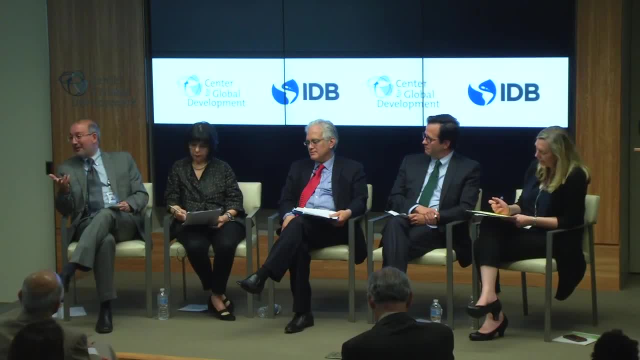 Mm-hmm, Mm-hmm, Mm-hmm, Mm-hmm, Mm. As I said, the case study- And in the case of Argentina, it was the new administration that was willing to be a case. But as we were working on the case study, the professional stated that look, now we 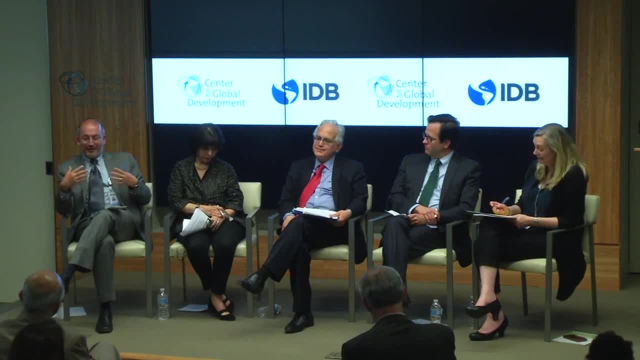 need a second. We need to do this again, Because Argentina truly became a success story of how things can turn around quickly, quickly. Now there were no crises in the other nine countries, so things are the same as they were. Here. we really do see a big change, and I think that the role of international 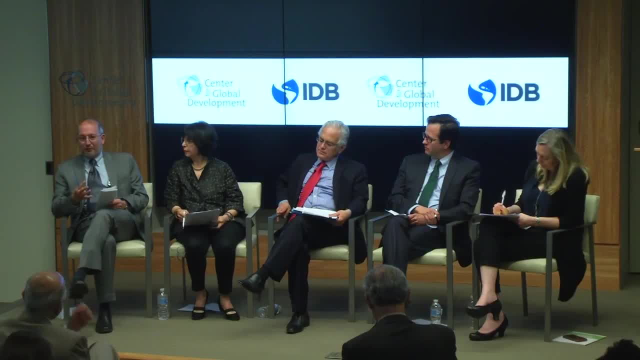 organizations was essential. Of course you need the political support and I was lucky to be there at the 50th anniversary of INDEC in January and we had the president opening the ceremony, but we also had the head of the statistical department of the IMF, the 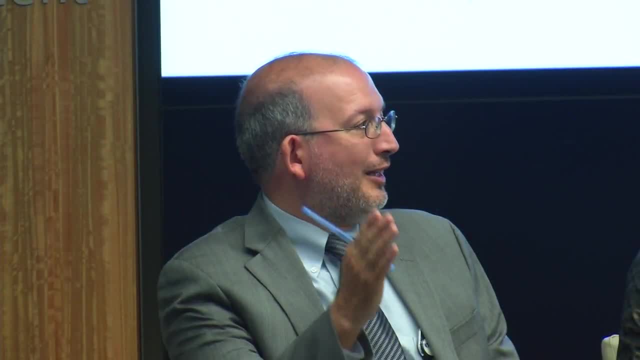 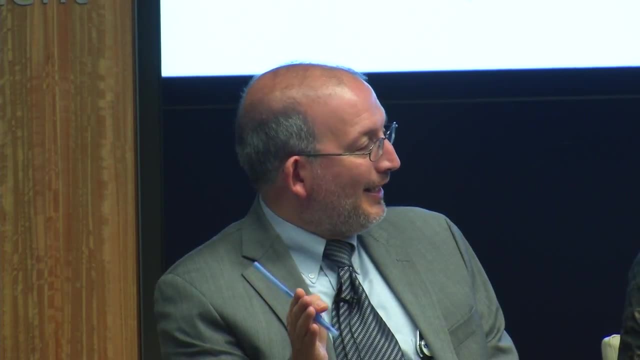 head of the statistical department of the World Bank and the head of the UN Statistical Division, and not only that, but also the head of the statistical department at the OECD. There's a saying in Spanish that nobody's a prophet in his own land. I think, of course. 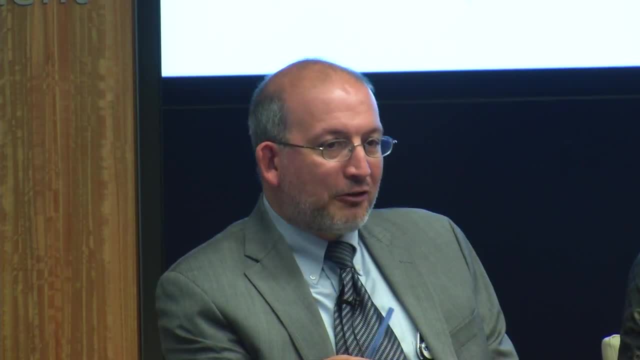 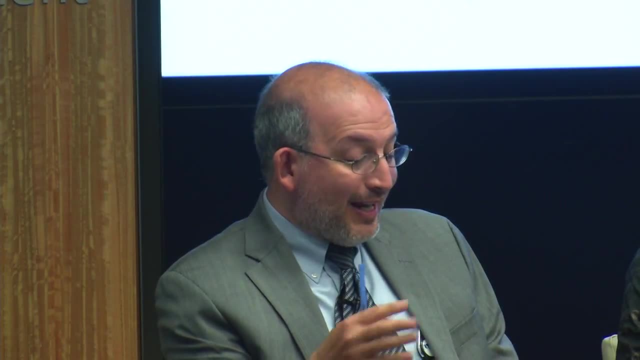 these people came to say the same things that the director of INDEC was saying. but it wasn't the director of INDEC, It was the head of the statistical department of the OECD saying them and in that sense, and going back to what Roberto was saying, you know it was. 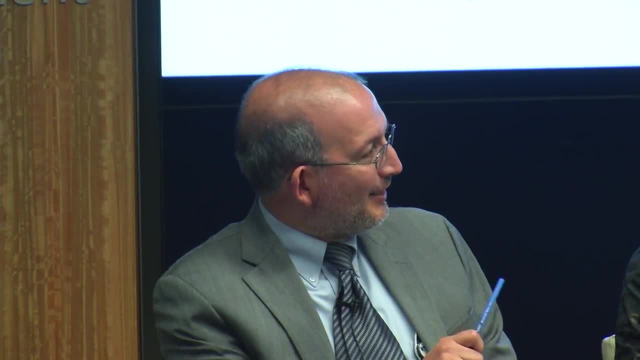 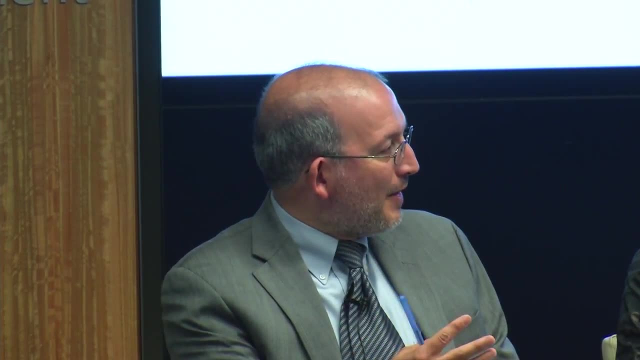 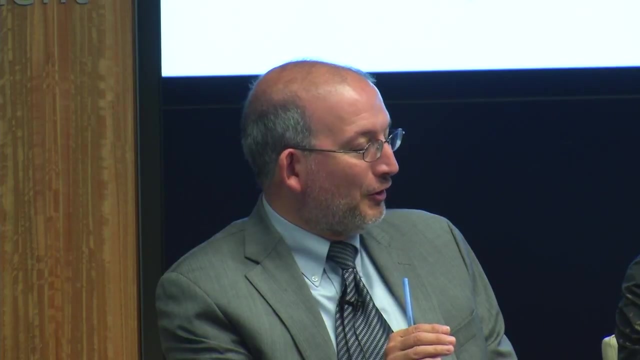 the role has been more relevant for the OECD in Argentina because they don't have a stake. You know they are members of the World Bank, they are members of the IMF, so there's always that political sensibility In the OECD. they want to be members of the OECD. so INDEC has 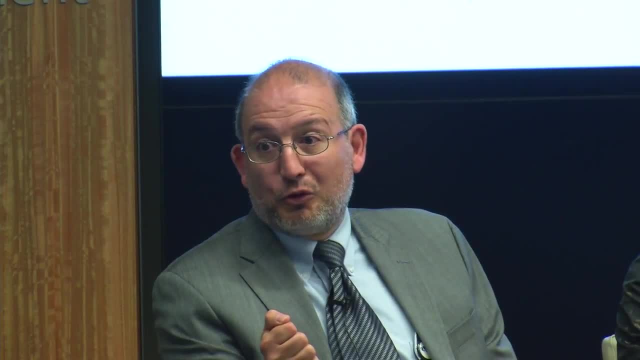 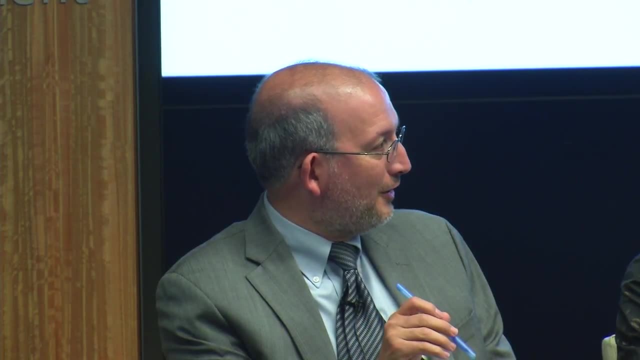 really used this as a leverage, for example, to push for a new law. And here I'm just going to, if you don't mind, quickly jump to Santiago's question About the Congresses. you know, one of the things that we found on the case studies is: 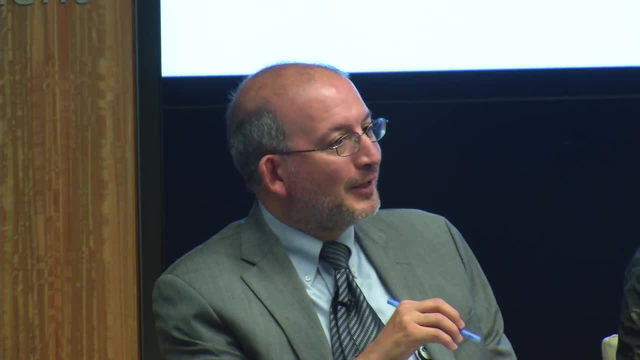 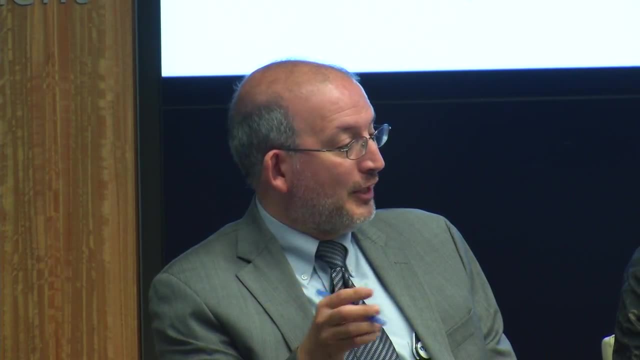 that Congresses in general do not play an important part. You know they should, but they don't. I mean. what we do see is a country that I'm not going to name, but it starts with a G and it's part of the 10 case studies. that, where the census, you know, is the country. 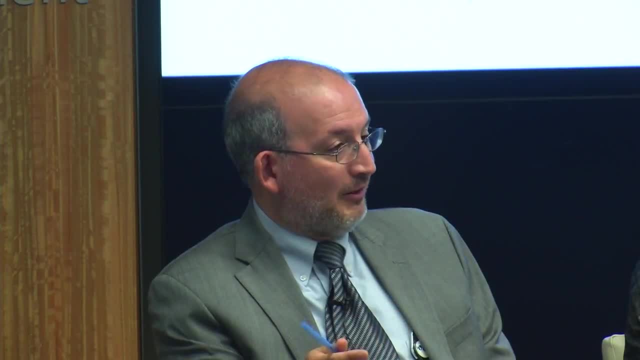 that is the country in Latin America that is more late in the urgent census, And one of the reasons that Congress did not want to allocate resources because that will mean different districts and it would mean that some of the members of Congress will lose their job. 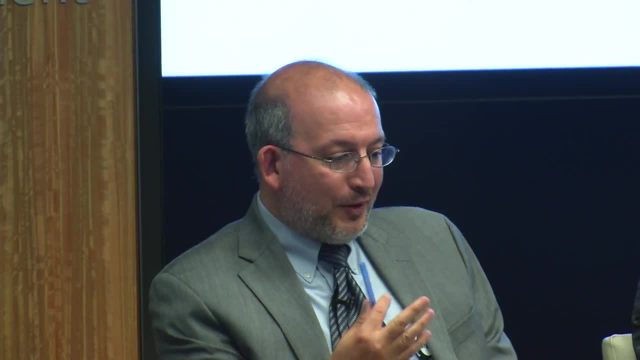 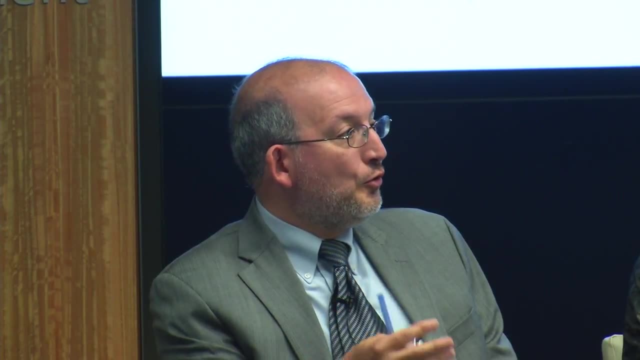 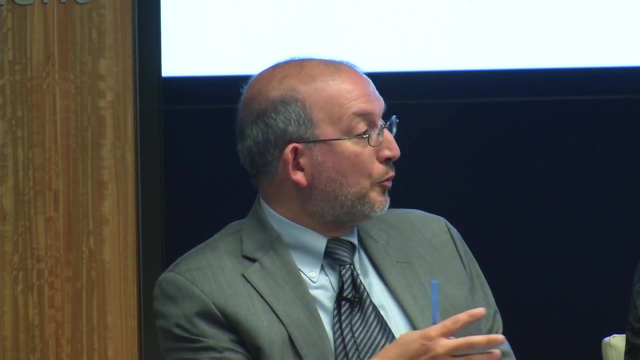 So no, and of course you know there's relevance, because I think one of the main things that needs to come out is that we definitely we need new legal frameworks that are, you know, that are modern, as I was saying, that have ways to protect the institutionality. you 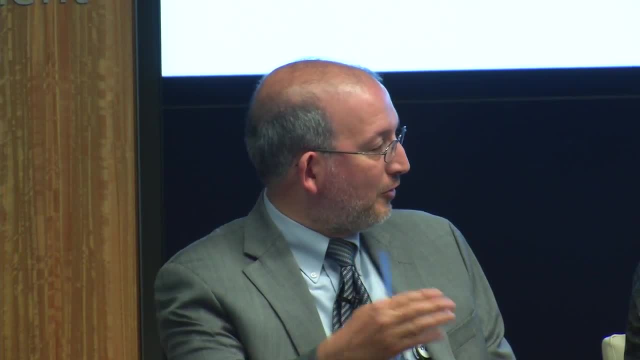 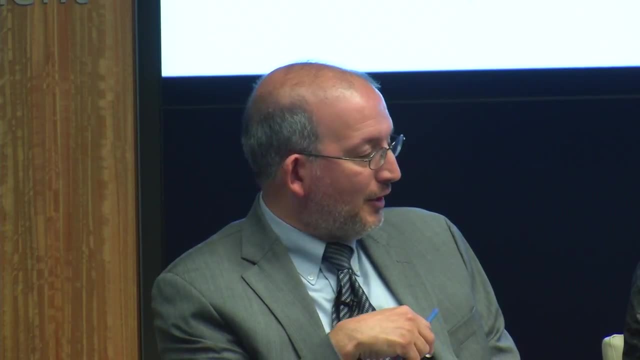 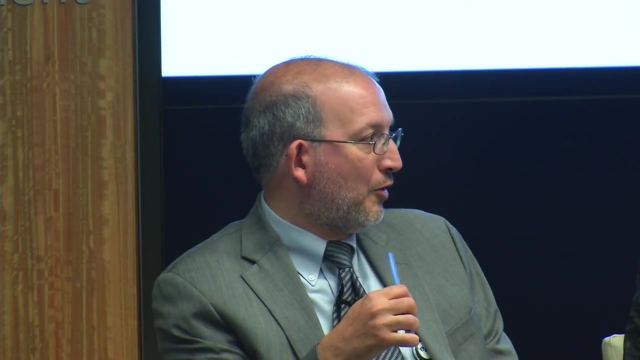 know, with a lot of periods, you know serving periods for the directors of the statistical offices that do not match the political, the political, the political terms of a of presidents, But you know, we don't see that much action, unfortunately, in the legislative brand as we should, we would. 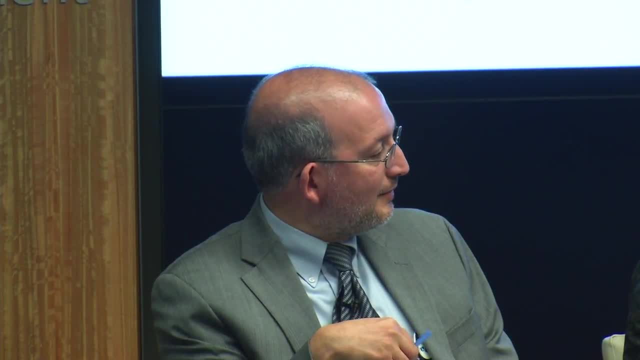 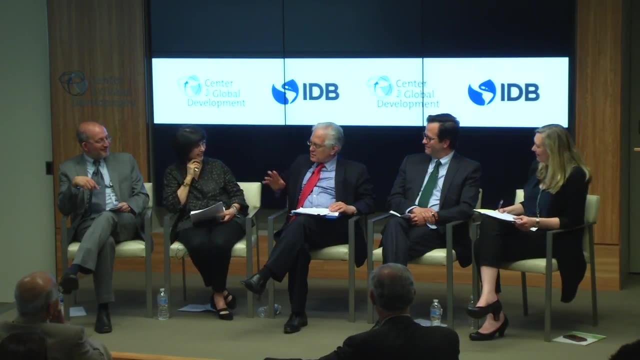 like to see Mm-hmm. Did you want to say something on that same topic, Roberto? Well, if I think I know what country he's talking about. The issue of it's, and I agree with everything you say, but the issue of security. 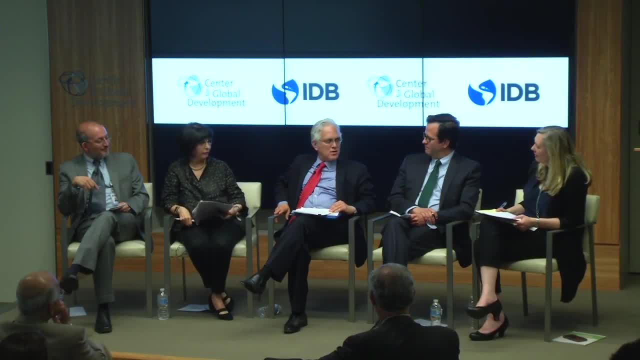 is also important. I was in that country about 12 years ago and, on the one hand, the private sector was saying we want better statistics and I would say, well, in that case we have to respond to the questionnaires. and they would say no, we are afraid we could be kidnapped. we 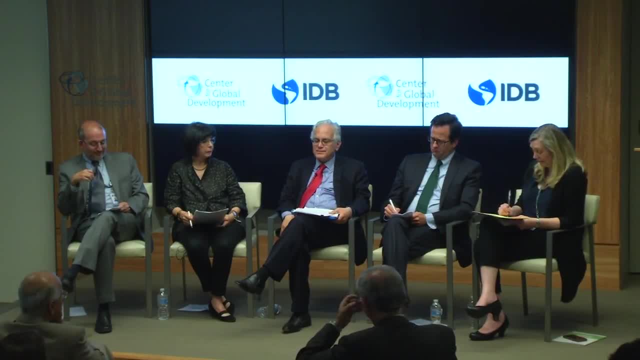 could be so the question of security is also an important question Interesting. What about the Ministry of Finance? What are the arguments that would be most persuasive when speaking to the Ministry of Finance? You earlier mentioned that having a constituency on the outside helps with budget negotiations. 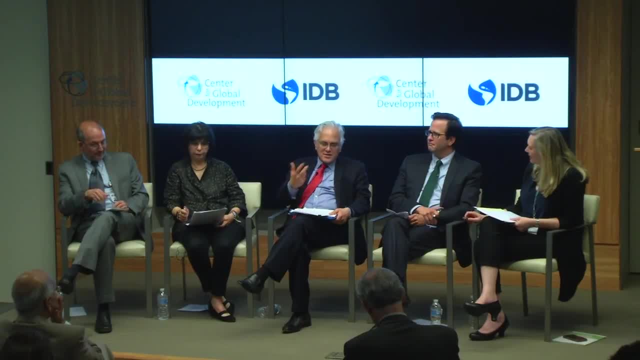 What else? I think what I see is that what I have seen is that certainly, working with international institutions when the IMF goes, and in fact I can tell you very, very specifically, sometimes a head of the statistical office feels that he needs more resources for this and for that. 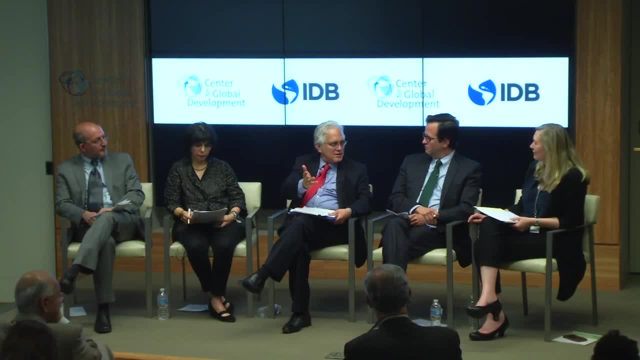 he calls the IMF. He says, look, can you do an assessment? A ROSC, we call it. We go and the assessment usually will realize that there is. so we make a recommendation. He goes to the Minister of the Central Bank here and says, look, the IMF is saying we. 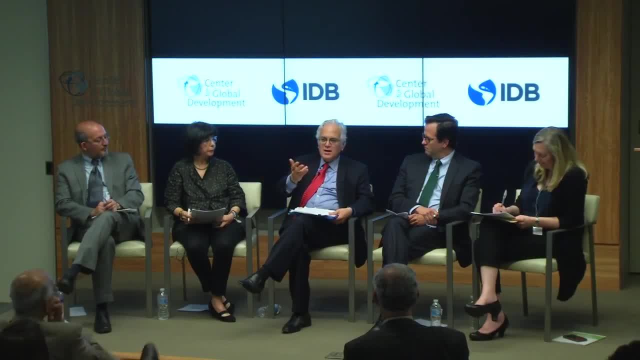 need more resources. The same with the IDB or the World Bank. The IDB may say: you need more resources for better education data, better health data, better hospital data. so they go and say, look, the World Bank came, the IDB came and 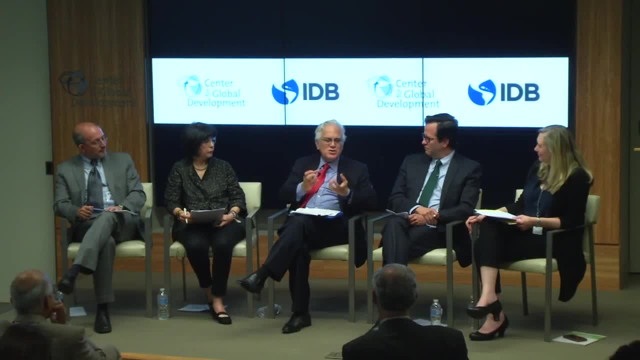 they told us, They told us, and the Ministry of Health is in agreement, so he needs to form a coalition. I think, Yeah, yeah. So assessment as the way to understanding what the resource needs are and, Shida, what. 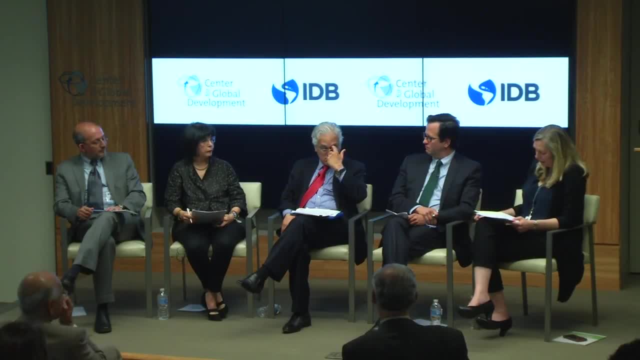 about the role of data users. That was a question that it's governments come and go. data use communities are forever- Yes, I really really— Or as long as your foundation funding lasts right, Absolutely. I think we've seen that the data users have played a huge role in California. 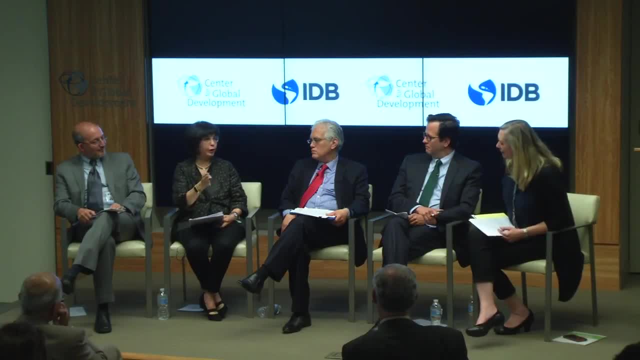 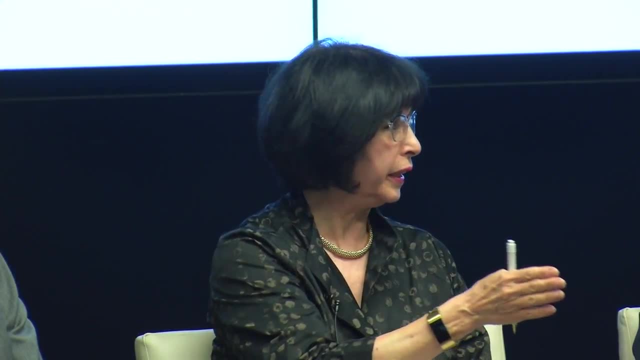 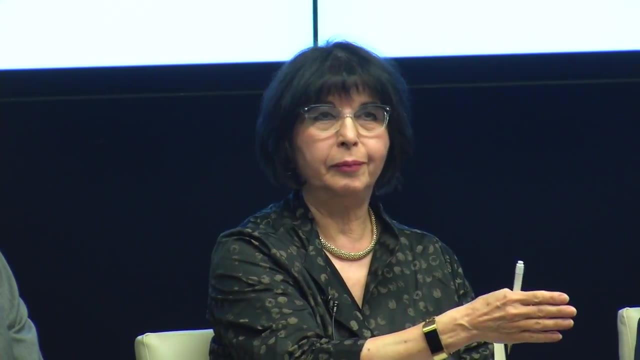 Yes, And capacity building for statistics. if you look back at some of the really successful sectors like national account prices- you know I look back- you see that it started actually with researchers like the Penn World Table with Bob Summers and Alan Heston, and 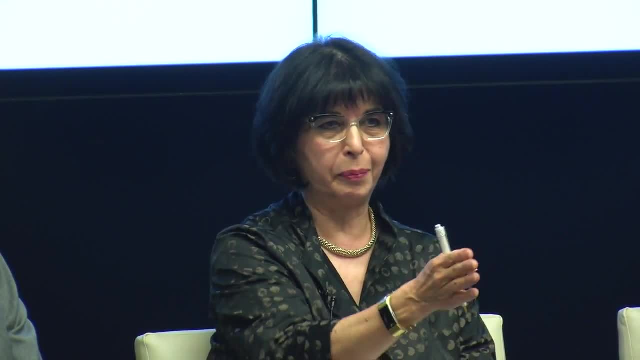 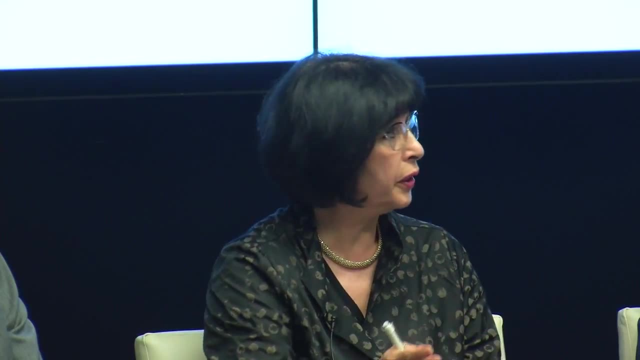 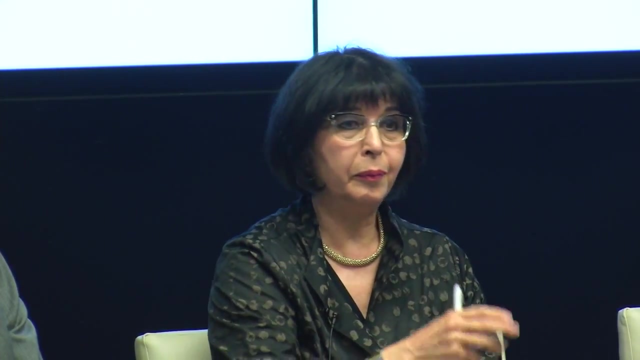 those guys at the Penn University in 80s and 90s- Masoud remembers those. They really were the initiating demand from the—and then the countries responded the UN system. The UN system responded: IMF methodological advancement. So users have a big role to play if it's done right. 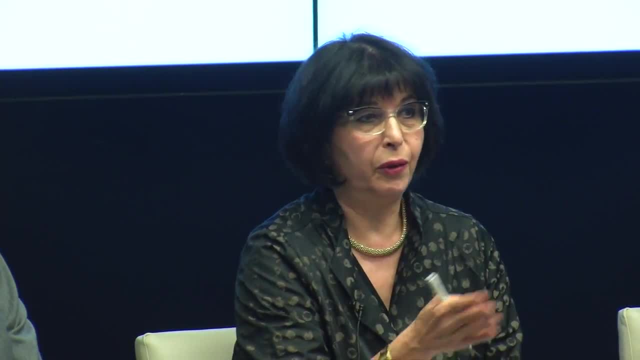 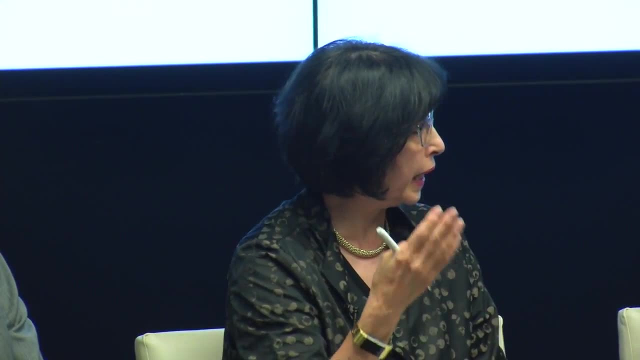 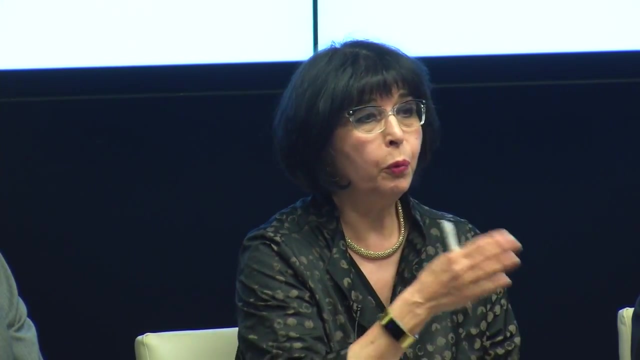 Sometimes the users and researchers set bad examples. you know, because you know in my field of open data they're guilty. Researchers hoard data, they don't make it open, so they also set a bad example. So it's not always, you know, bringing good things to the data ecosystem. 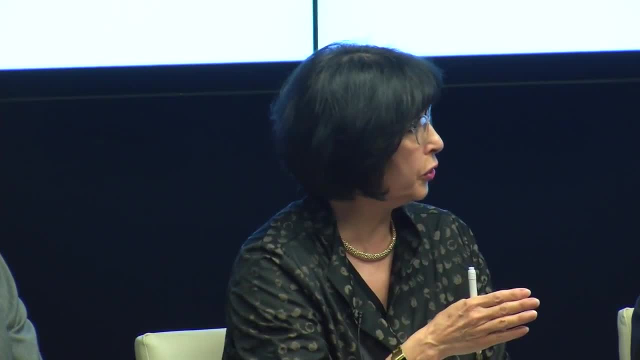 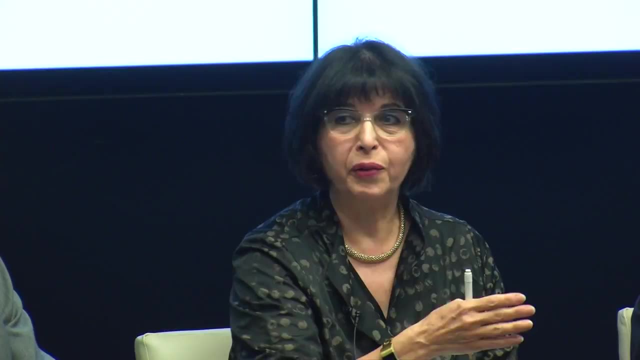 But one group I think we haven't talked about much. Okay, It's the CSOs. the civil society organizations have a big role in this ecosystem And we've seen and respond to some of the questions. that also adds the value as a user. 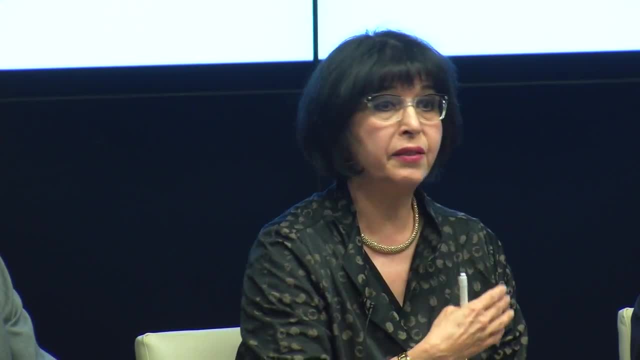 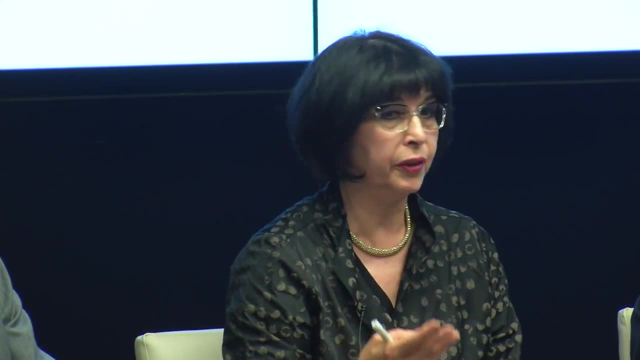 but also as a sort of calling out issues that sometimes is difficult for IMF to raise because of the- you know their standing- or the World Bank, but CSOs can because of our independence And in fact, for example, the gender data has been a big issue for many years and it. 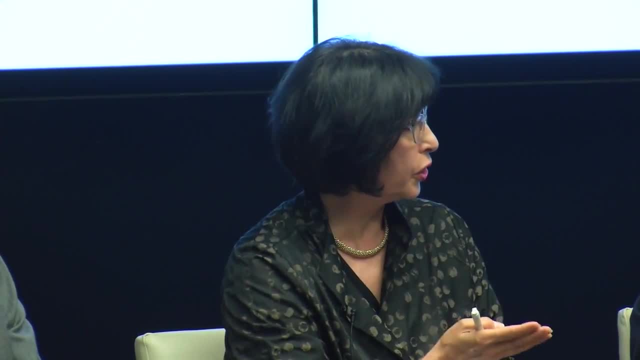 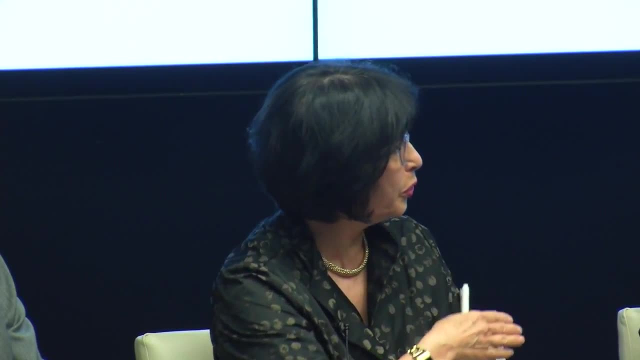 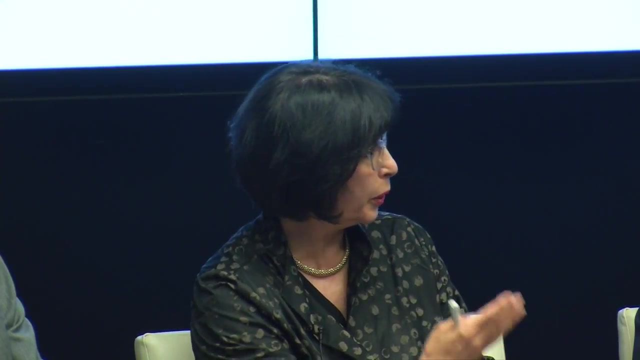 was a CSO, Data2x, that started really putting this on the map that we have a data gender disaggregated data crisis. So, users, CSOs, we need to partner with them and, you know, really bring them into active participants in this ecosystem. 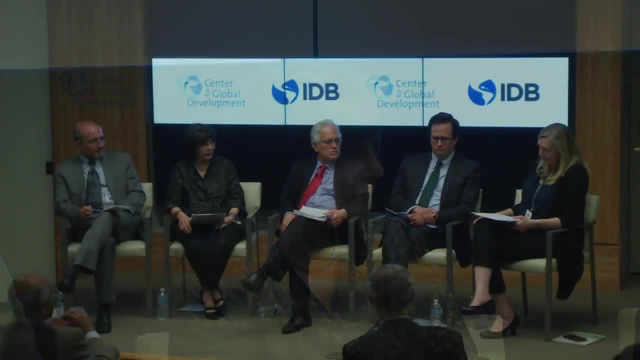 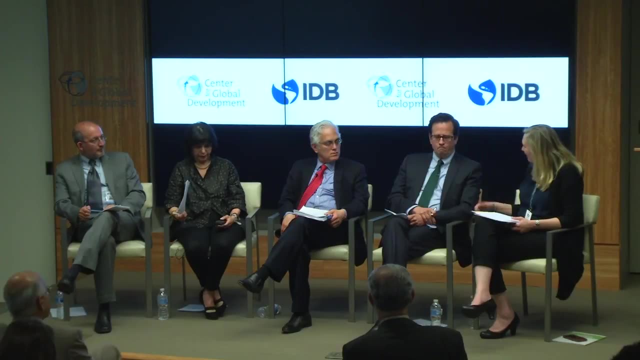 Yeah, that's a really great point. What about the statistical capacity training institutes that we see elsewhere in the world? Why don't we see them in Latin America? Yeah, I mean, I it seems like they actually the statistical institutes themselves actually. 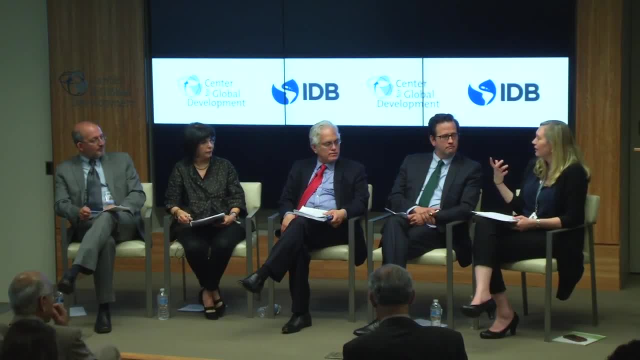 serve that function. I guess the question is: do they? how much funding or how much mandate do they have for those kinds of exchanges amongst themselves? Do you have a sense In the golden age of Maccoby? Do you remember Maccoby? 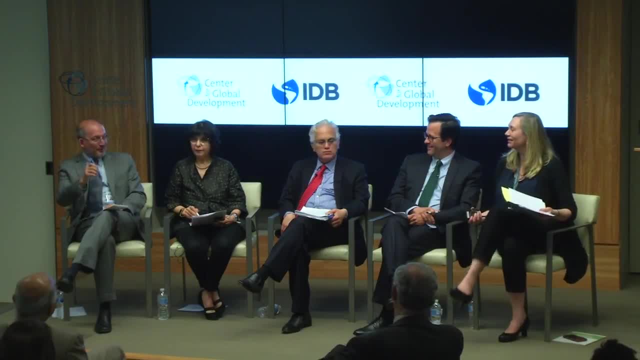 For example, Anyone here, I do, yeah, And I'm too keen on the numbers. I remember part of it. yeah, Kira knows right. It's a program to work on the standardization and use of household surveys in Latin America. 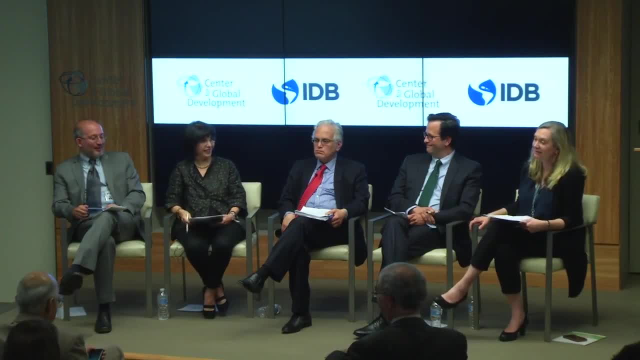 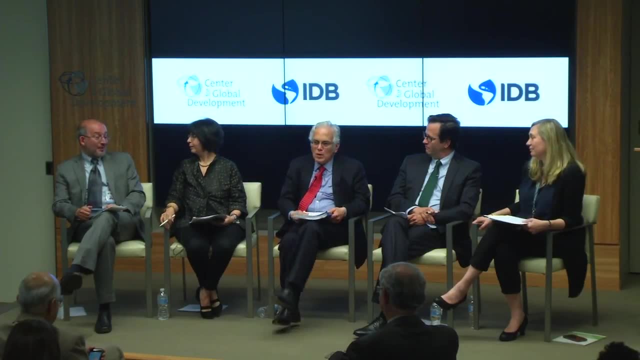 And it started from the users, from the researchers. It started from the users. yes, In Latin America in the 60s and 70s, you know, first you know, they have CELADE, which after a couple of years they had a master's in demography and many of the older generation. 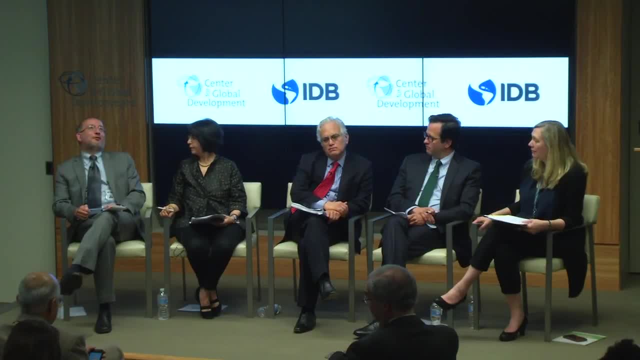 of demographers in statistical offices come from there, And there was another one that I keep. I cannot remember the name, but there were some, some and again it's an issue of has turned out to, I think you know, an issue of funding. 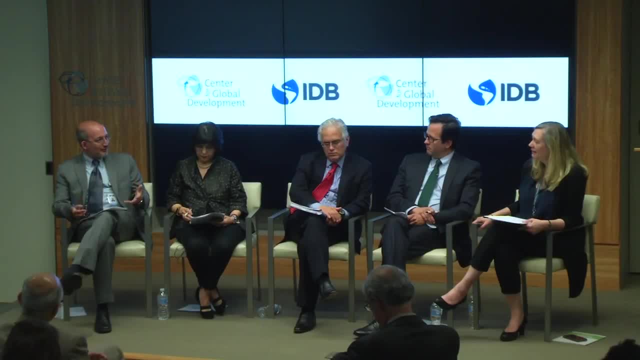 and also an issue that, as you said, you know some of the, you know some of the you know some of the more advanced countries have taken that role. Colombia has a training institute, Peru has one, Mexico has one and, I think, the community. 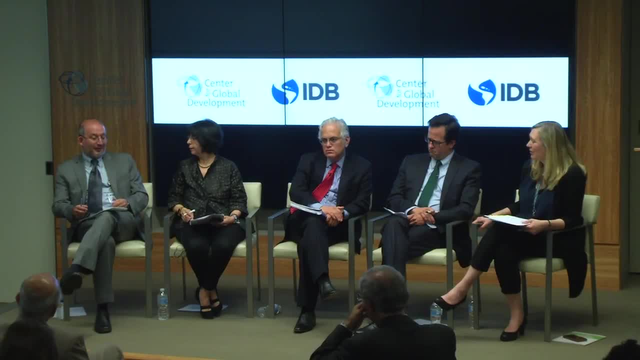 of statistical offices. the Statistical Conference of the Americas is, you know, trying to informally have that without having a, you know, without the need of a building having, you know, this online training course That works, yeah, Mm-hmm. 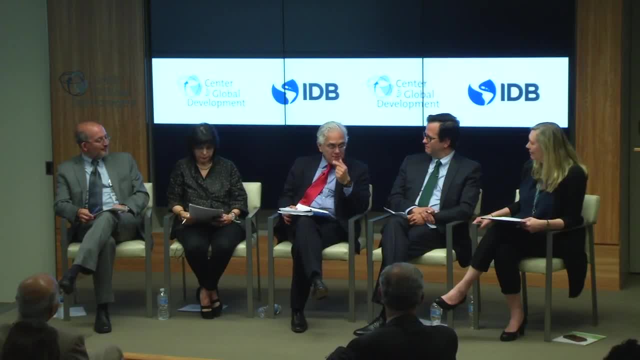 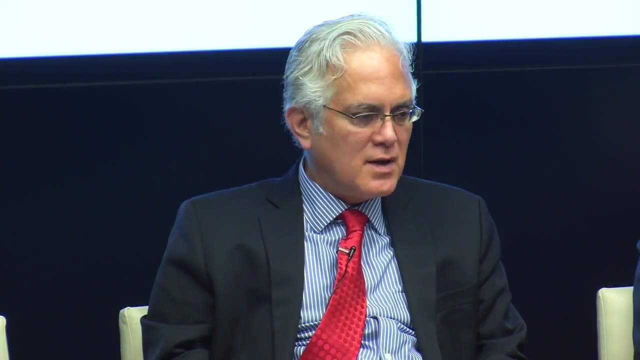 In the case of the IMF, I have to say that we do have considerable training on microeconomic statistics for central banks, ministers of finance and the statistical offices, including in association with the Bank of Brazil. We have a regional training program there. 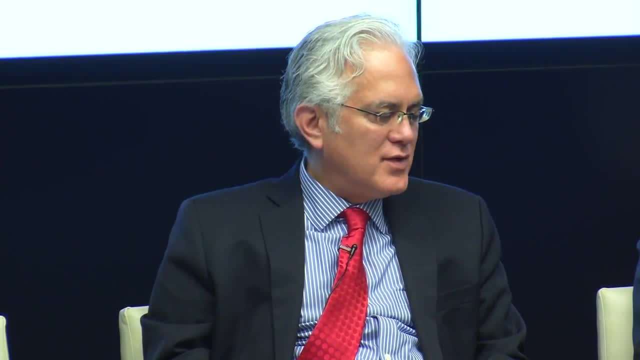 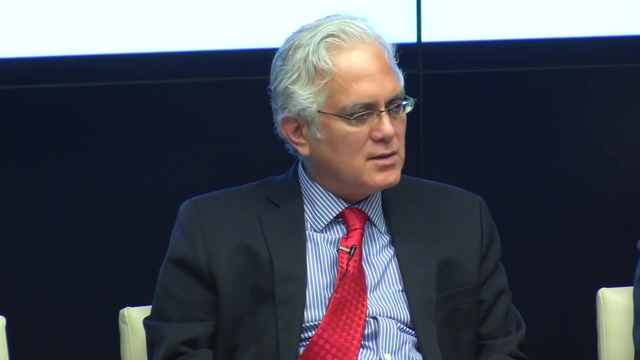 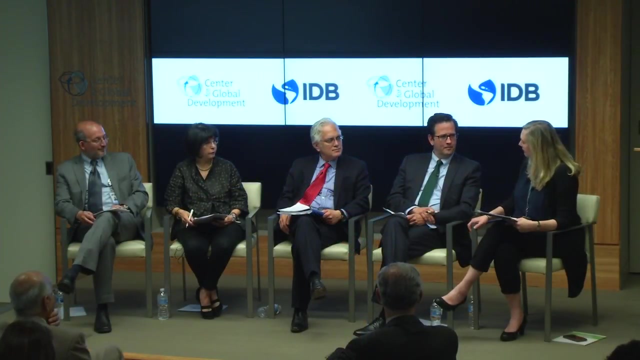 So I'm very confident that in this area there is plenty of training for Latin America, Plenty of supply And demand. maybe, I don't know, Do you have any thoughts on this, On bad news, what to do? So I think that's a fascinating question. 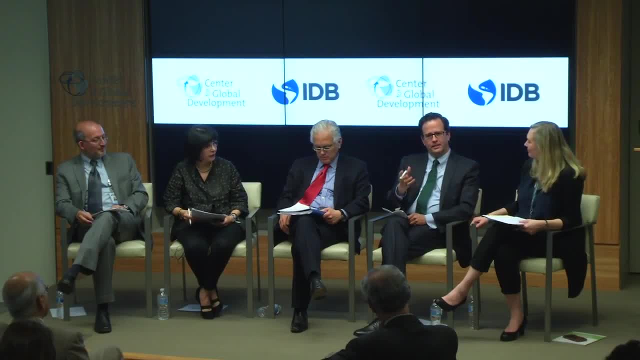 And I. it maybe points to the flip side of politicization. You know, bringing other communities in can be good in the long term but it can also be damaging in the short term. I think of the literature on judicial independence And I accuse my academic sort of 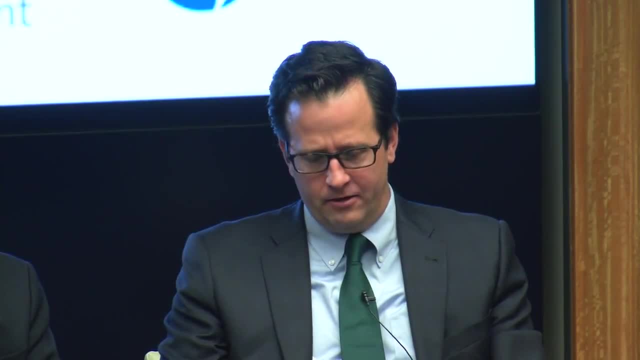 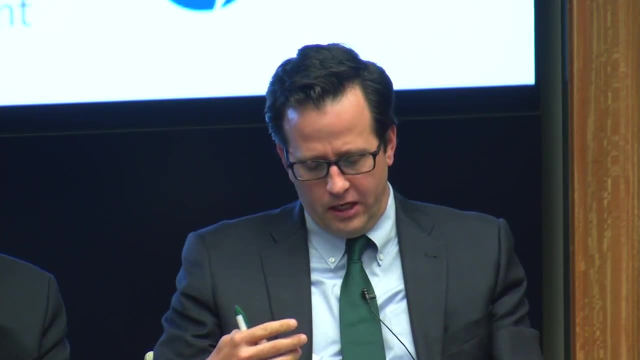 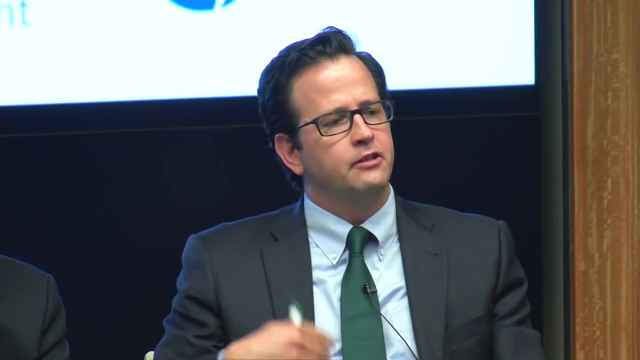 Yeah, Meandering here. But in the literature on judicial independence there's a thing called insurance theory, And it's that courts become independent when incumbents realize that even bad news can serve them in the long run And the opposition realize that at some point they'll be in the incumbency. 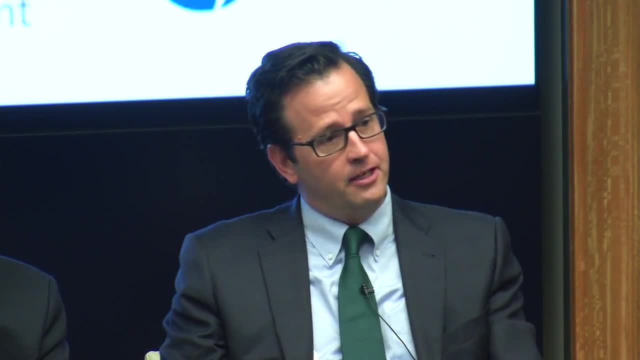 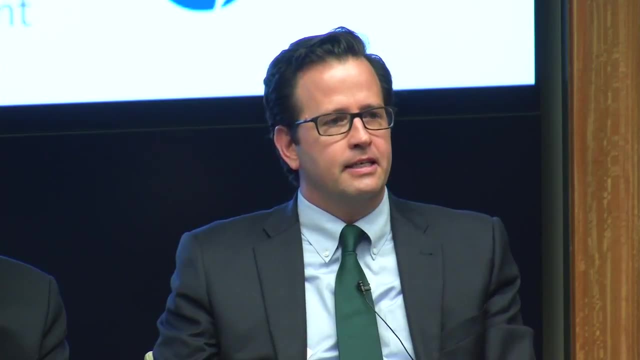 And therefore they should tolerate bad news when they're in incumbents, because they can use bad news when they're in opposition. And so you know, I think that statistics is a little like this right, That there are reasons why parties in Congress may want to encourage statistical autonomy. 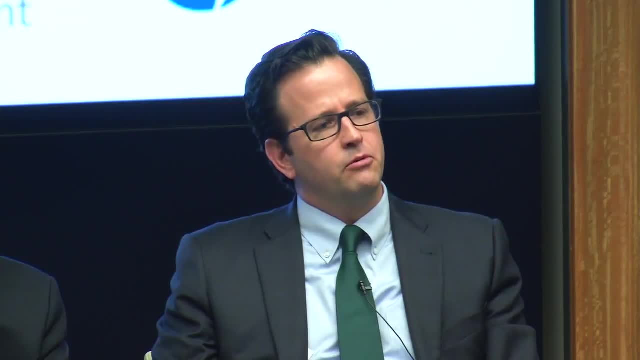 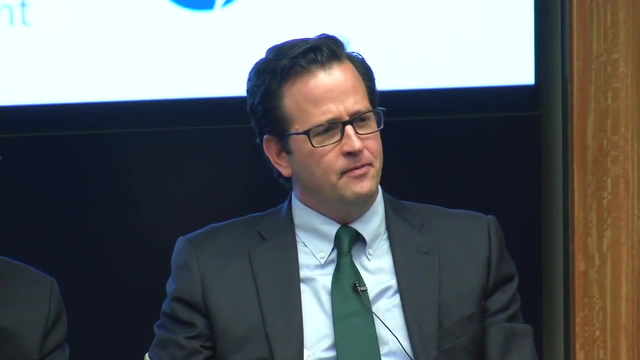 But there's also there are reasons that incumbents may want to encourage it as well. The incumbent today may realize that if they tolerate bad news today, they'll be able to use bad news against their opponents when they're out of office, And that's sort of the general theory. 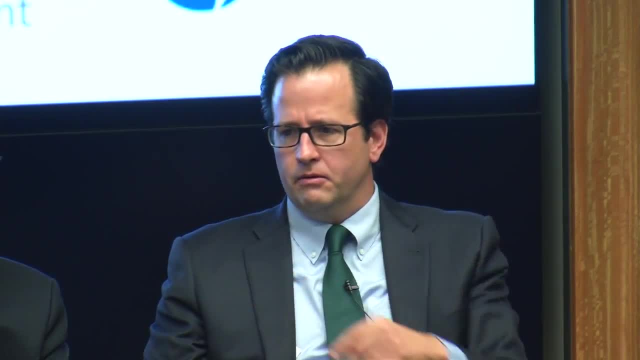 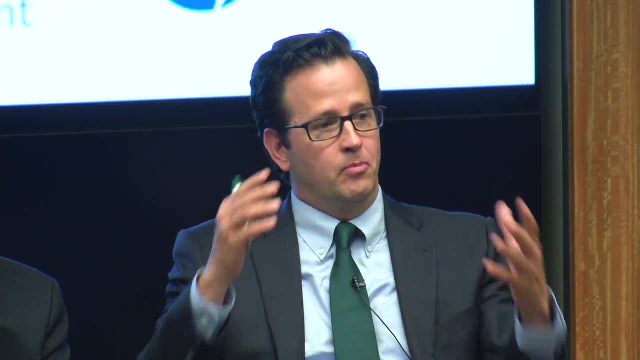 Now, from theory to practice is hard And I you know there was this question about Indecchi in Argentina And it's really hard to think about Indecchi in Argentina without reference to the broader political context of Argentina which for the past 60 years has been, you know, tacking. 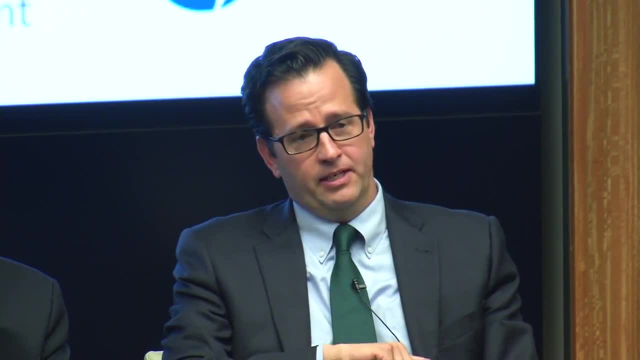 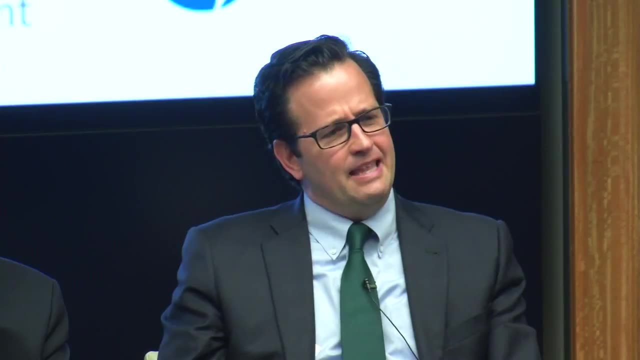 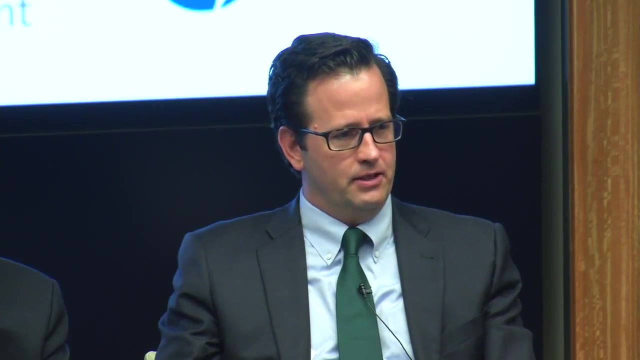 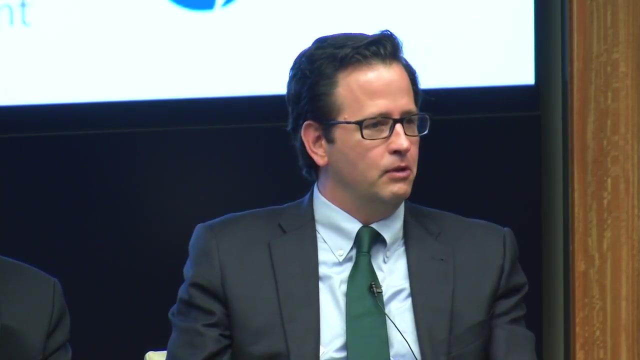 from left to right, from left to right, with hyper-presidential political system. that makes it, you know, a winner-take-all system. And so, in that political context, what does politicization mean, and what does politicization of statistics mean? So there's sort of a sweet spot between too much politicization and perhaps too little. 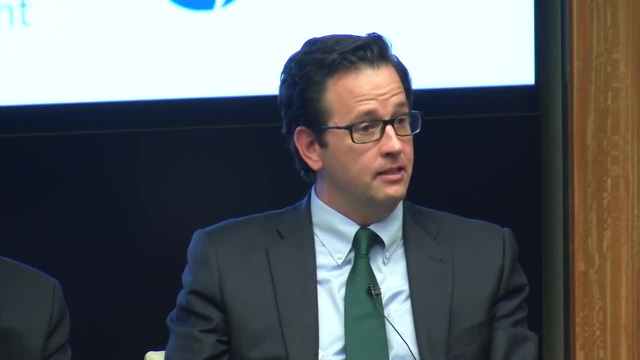 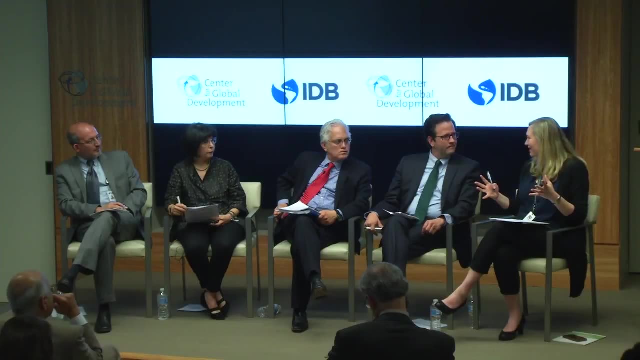 which means that statistical agencies aren't getting the attention that they deserve and that they need in order to build autonomy. Yeah, I think that's really important to put the function of the NSO into the politics and the institutional structure That the countries are living in any moment, as you're right. 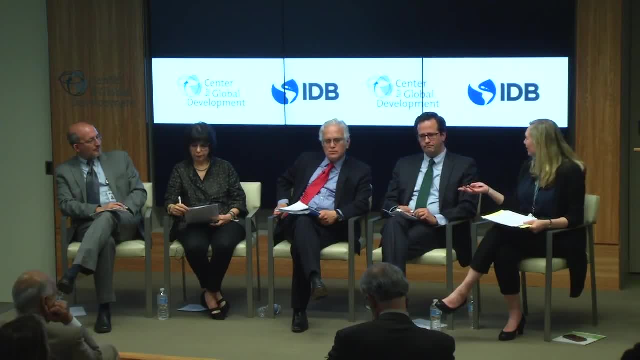 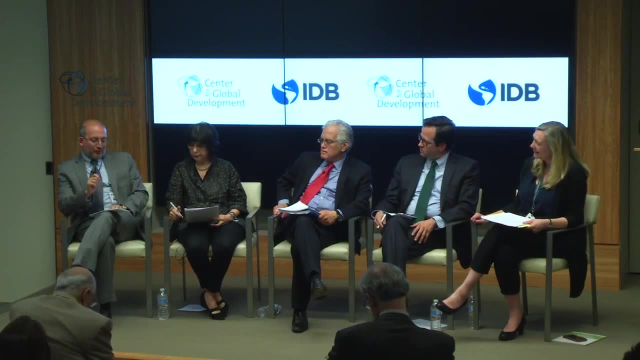 It's just a symptom. It's not necessarily that there's anything about Indecchi that could have changed, that would have made a different outcome possible. And on that I think there's. you know, just from recent experience with Inegi you know. 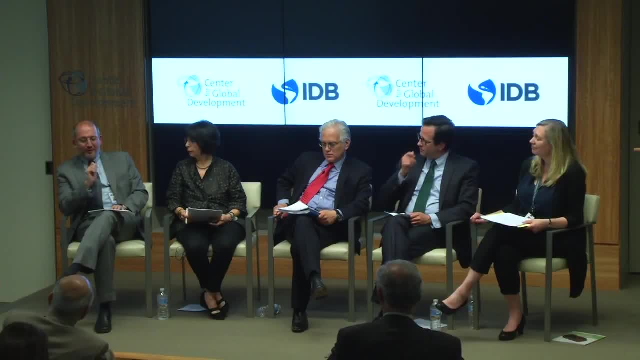 the law of Inegi states that in Mexico- the statistics of Mexico- any survey that is conducted by Inegi is public by definition, Unless it's a You know it provides data that is confidential or personal information In that sense you know when an agency comes and wants to contract Inegi to conduct a survey. 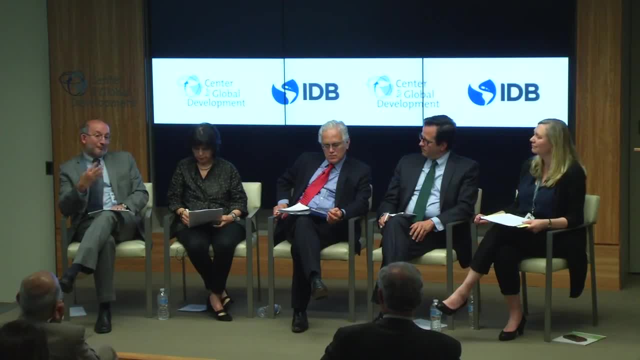 they know that in the contract it states that that data is gonna be public, regardless of if they like or not like the results. That sounds like a smart policy, then, to protect independence and the ability to publish bad news. There was a question about administrative data in health and you made the really great. 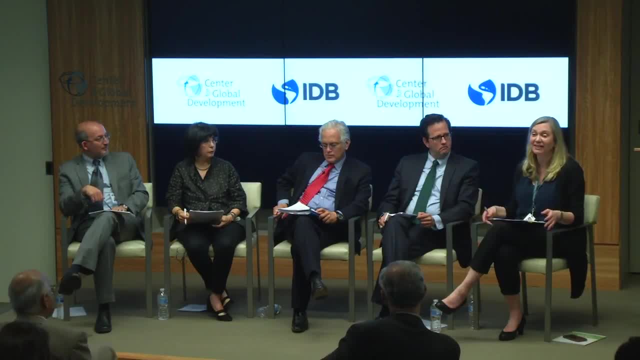 point that administrative data is the original big data and we're not using it enough. And some of the countries in the region actually have amazing databases of hospitalization and prescriptions and utilization in general. The statistical system doesn't wrap their arms around all of that data at the moment. 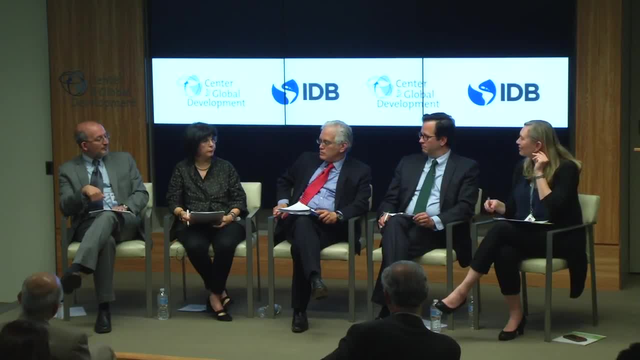 Could you reflect a little bit on the connection Shider, Jose Antonio and you know, these big administrative data sets that are owned by ministries, and what's the role of the NSO vis-a-vis the Those ministerial data sets and using them, checking, triangulating data sources? 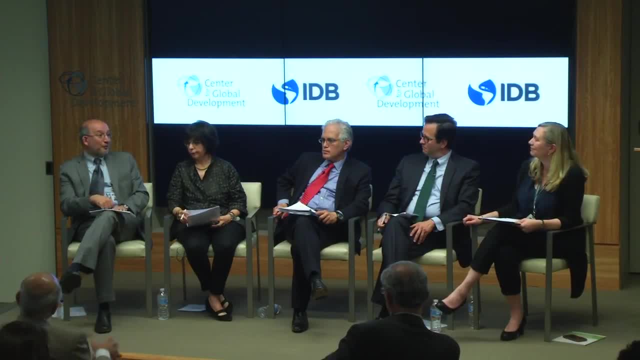 What do you see as sort of best practice from your case studies? Well, you know, of course. you know education and health, and now social development are the three areas of the government that have the biggest data sets, and I think that goes. 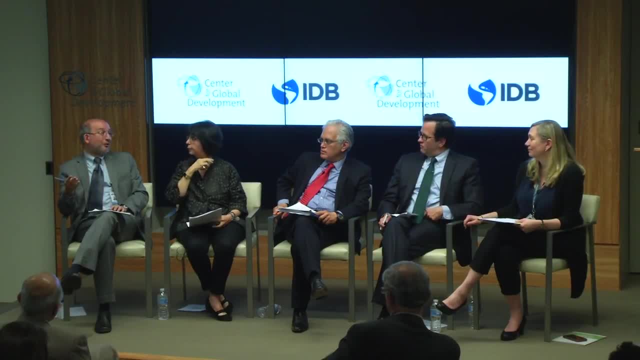 In one way it goes back to a legal issue of access to that information. In many cases, you know, there's not- There are no agreements, or there's no ground to make those agreements- for the statistical agency to have access to that information. 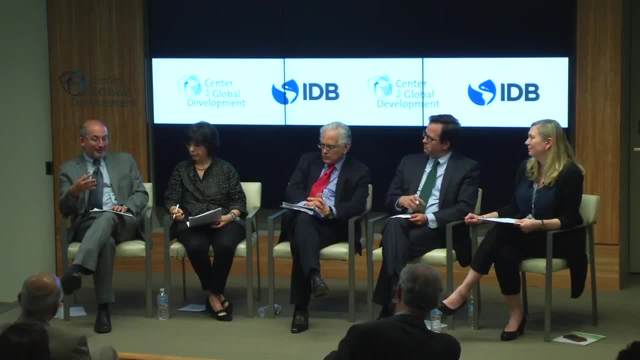 From another perspective, the statistical agencies, as coordinator of the national statistical system, should be able to set the rules of you know, in conjunction with these line ministries, of what are You know, what is the international standard we're gonna follow on the definition of disease. 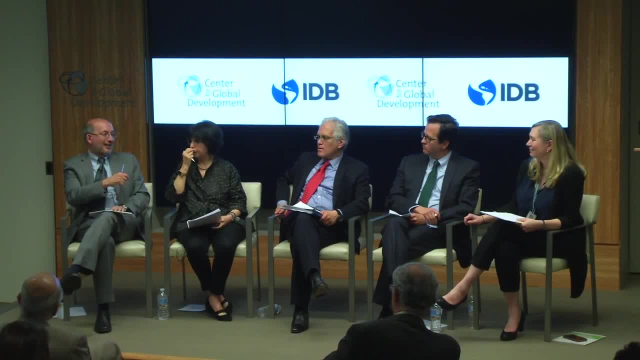 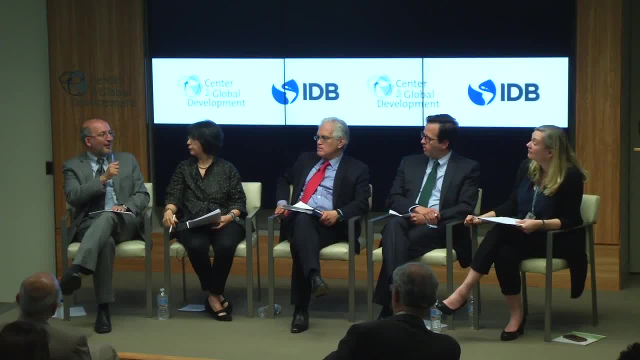